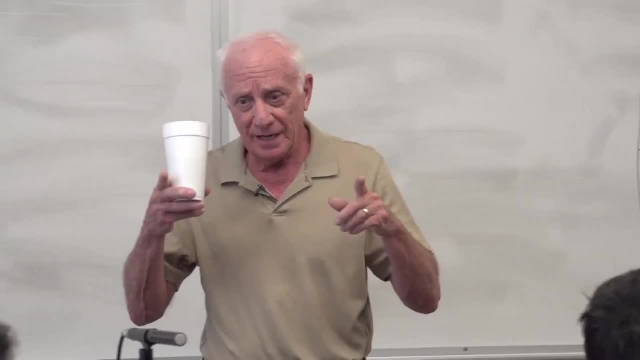 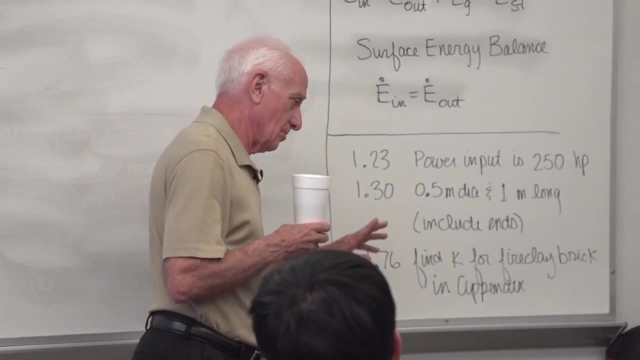 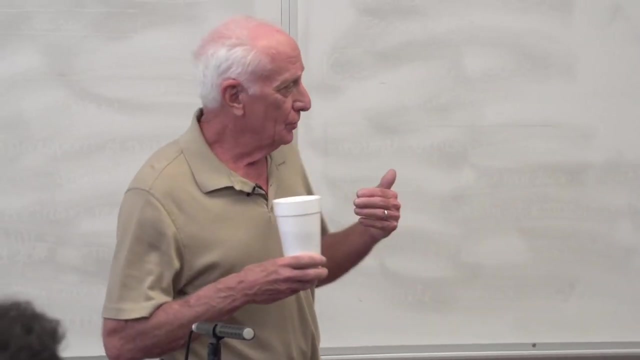 include the sides of the cylinder and the two ends of the cylinder. the sides and the two ends of the cylinder. The third example problem, or the homework problem 176.. I changed the material from the one given in the problem to fire clay brick. 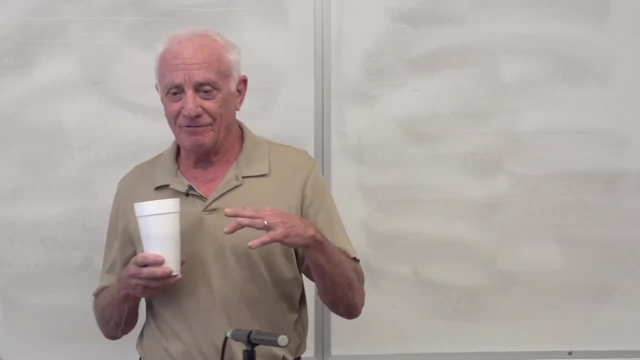 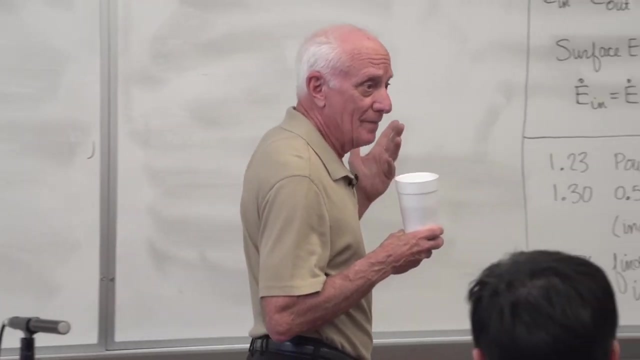 and I had an e-mail that said: where do I get K for fire clay brick from a student working the problem? Well, we can, I said, go to the appendix. You'll find fire clay brick. in the appendix, the K value. 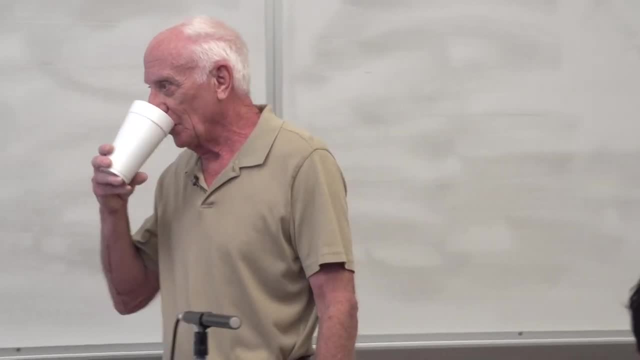 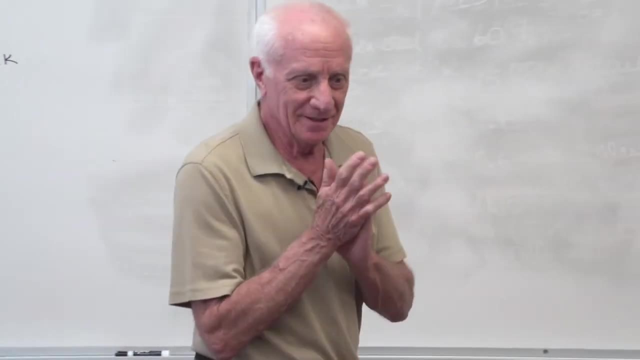 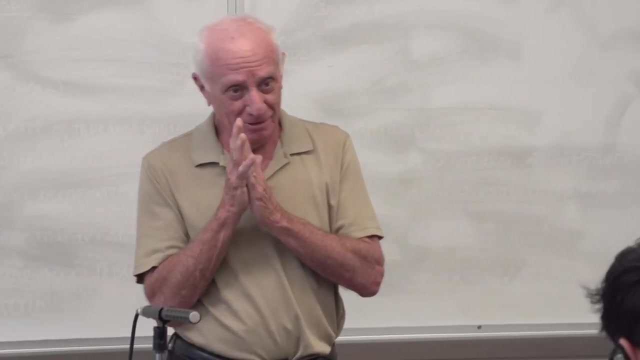 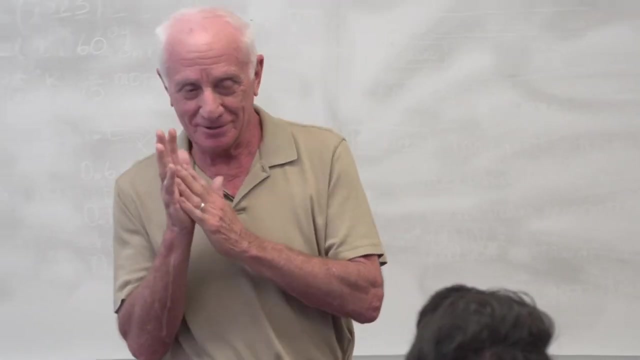 So go to the appendix to find that Now, if you happen to miss a lecture for some good reason, you can always go online to the ME department videos or YouTube and find my heat transfer lectures there. They was done three years ago. 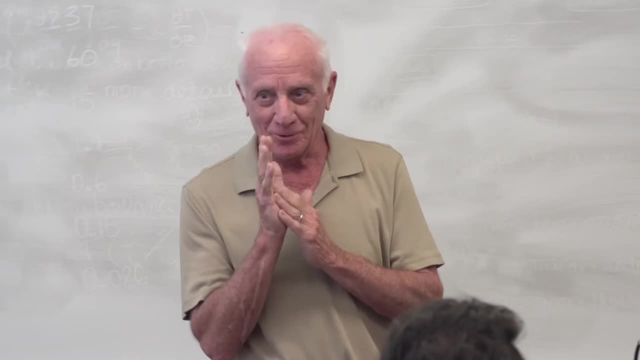 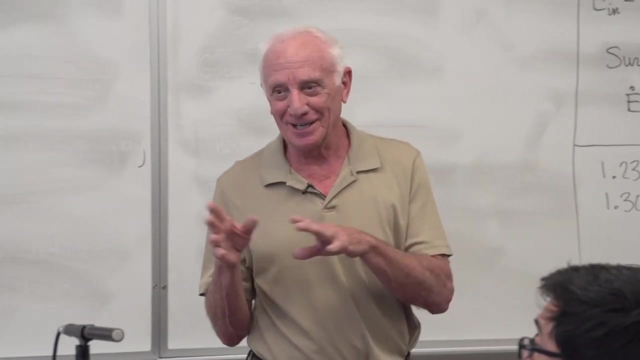 It turned out, the audio and the visual quality was not really that good, but they're online right now, So you can go there and find almost the identical lecture on those videos that I did three years ago. We're re-taping them because we 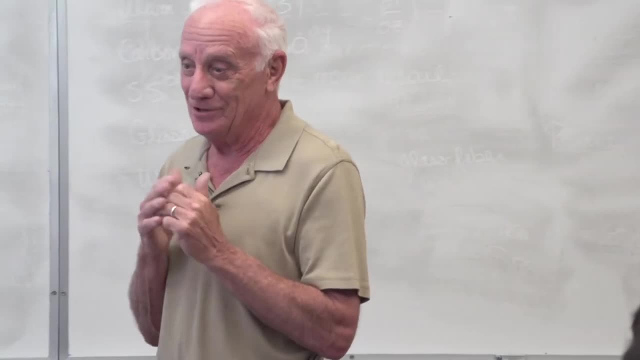 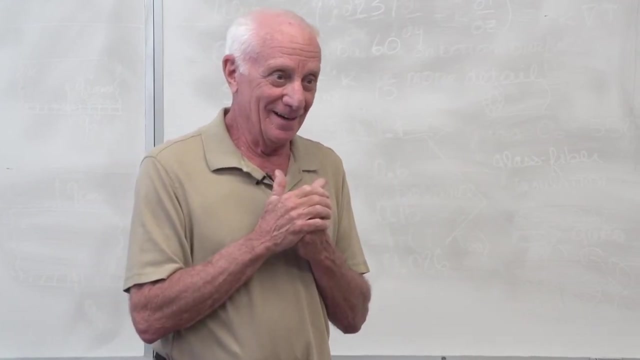 want better audio and video quality, But you can go right now to the videos and look at my lecture today. It'll look just like this one, But I hope you keep coming to class because if you don't, my ego is trashed. 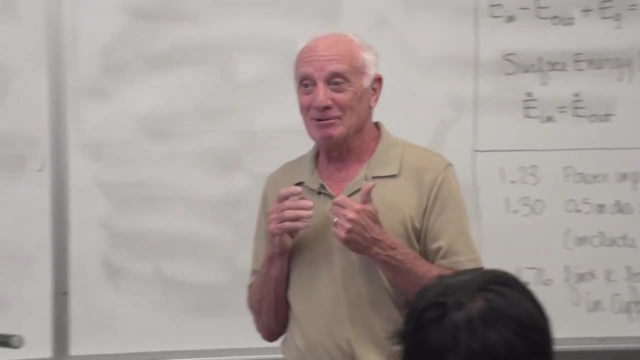 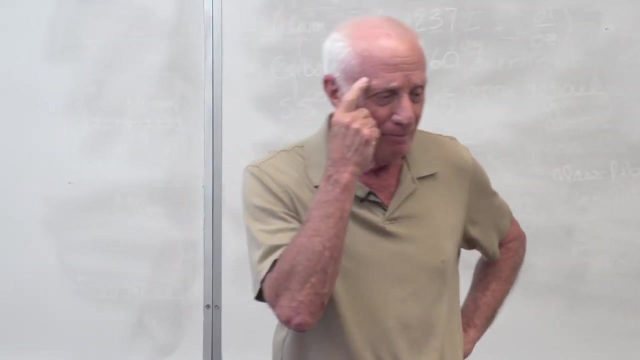 and I don't want my ego to be trashed. okay, I want you here. Okay, Those videos are great when you're studying for midterms. and a final, Because if you say, gosh, what happened back in January? I forgot that lecture. 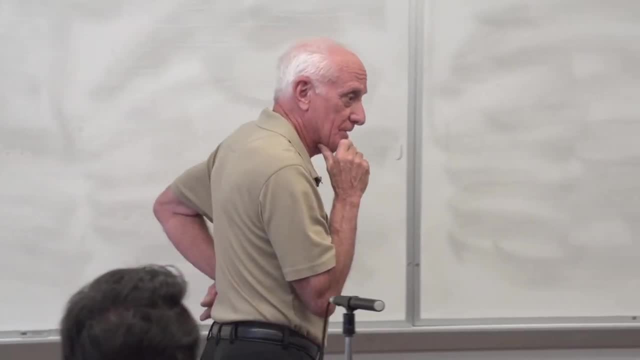 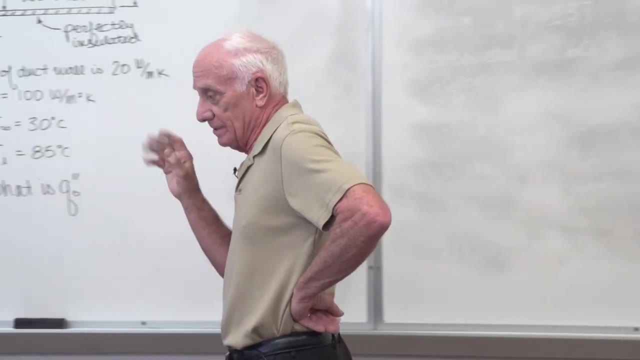 You can go back there and review that lecture. So it really helps when you're studying for things like that: midterms and final exams. Okay, Now we're going to finish Chapter 1 today, and here's the problem. we're going to 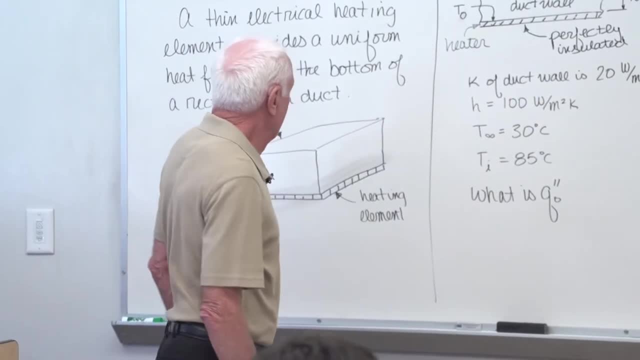 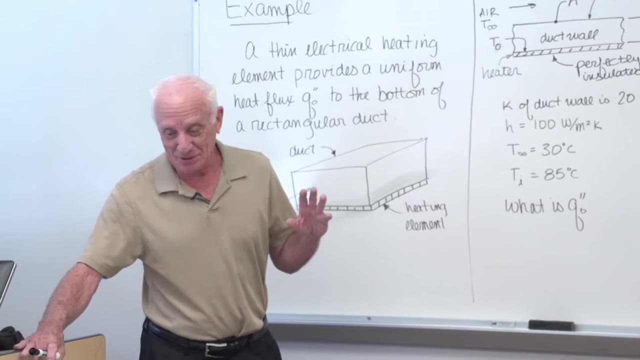 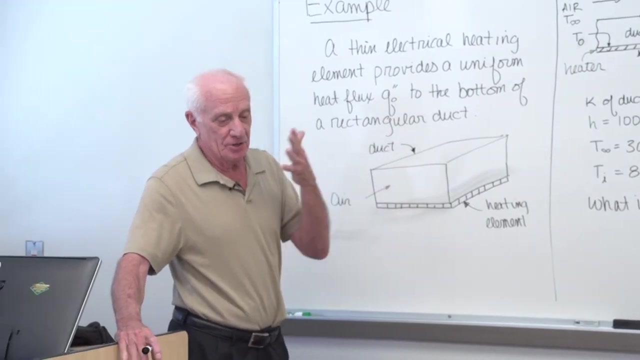 work with those two equations. up there The problem. these problems come out of the textbook. We have two possible textbooks. It depends which one you have, But they come out of the textbook, Because I'm not sure what textbook you have. I'm going to try and explain in. 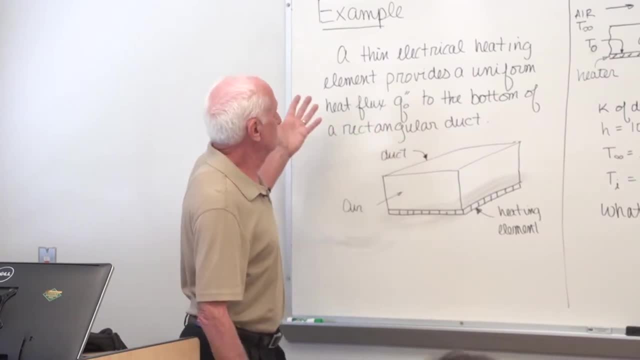 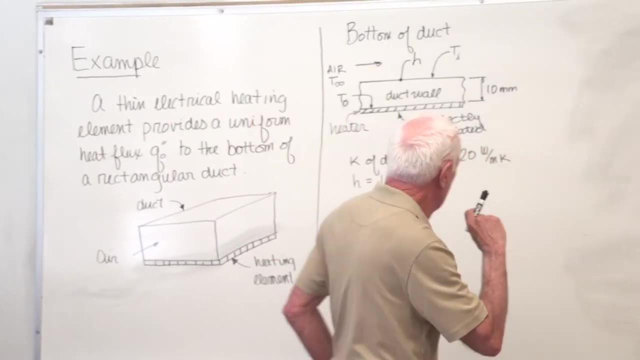 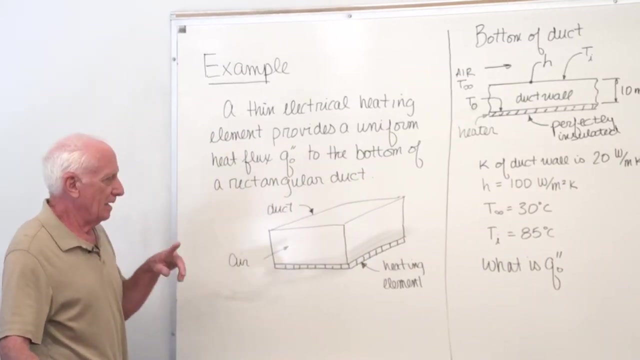 very much detail what these problems say. So this problem is a duct, a rectangular duct, like the HVAC duct in the wall up there. We're going to try and heat air in that duct. Air is flowing in that duct. To heat the air we're going to put. 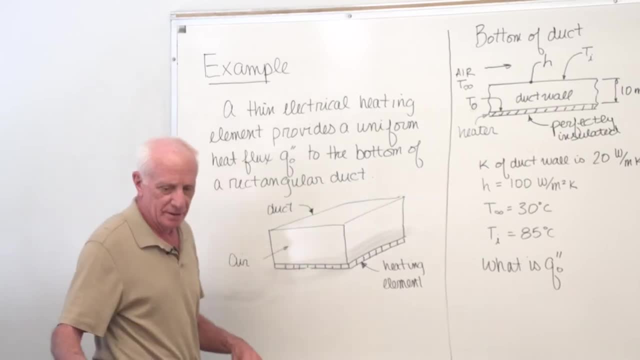 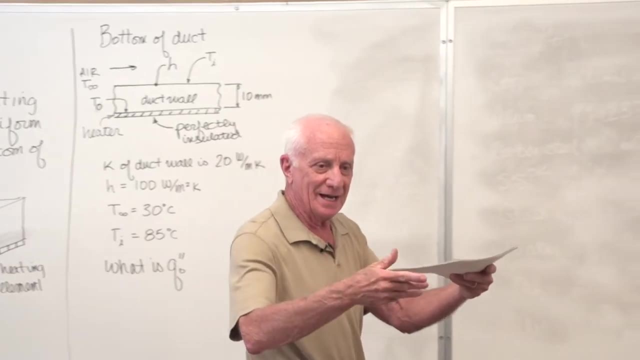 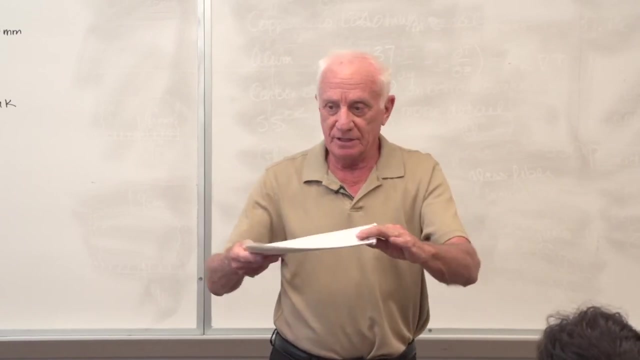 a heating element on the bottom surface of the duct. That heating element could be something like this: with two wires coming out and you put this guy across some power supply and it'll generate heat. It'll generate so many watts per square meter. 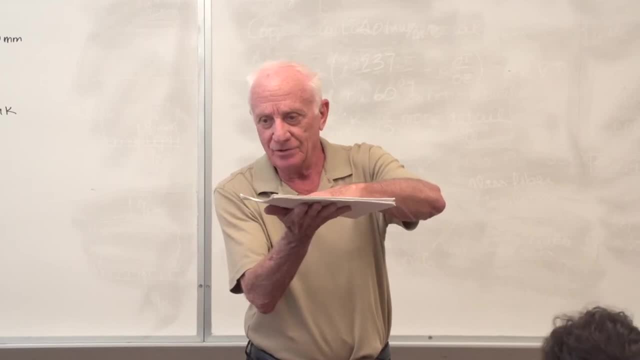 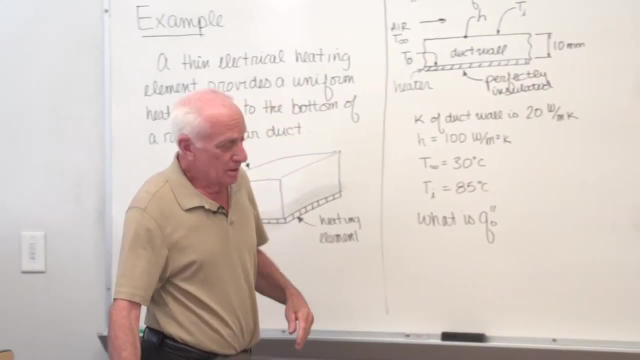 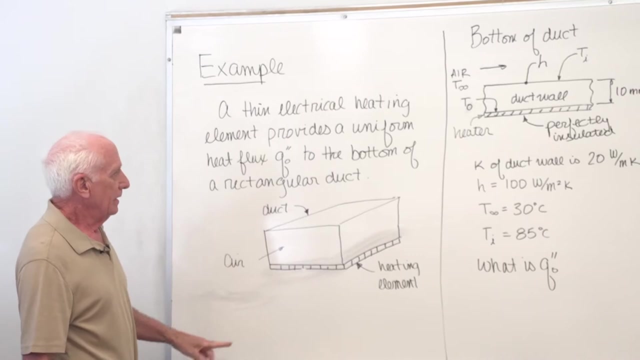 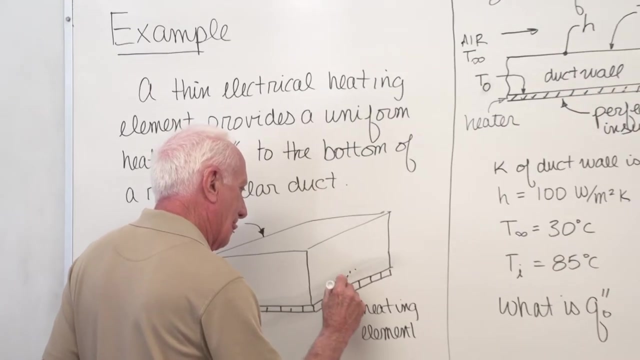 and you attach that to the bottom side of the duct and now you heat the bottom duct wall, which then in turn heats the air going through the duct. We call that heat flux Q naught double prime. Here is. I took a piece of the wall out to show you. 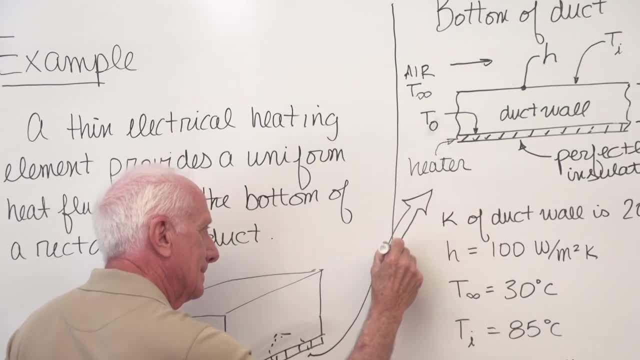 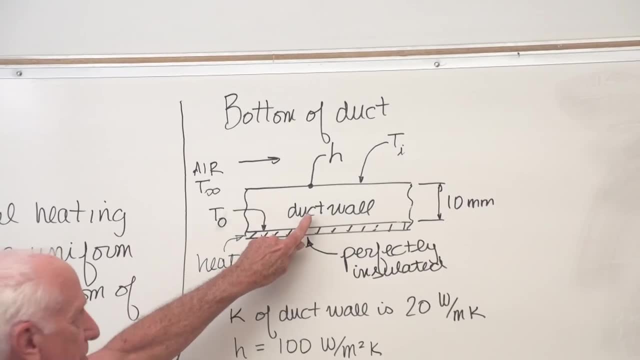 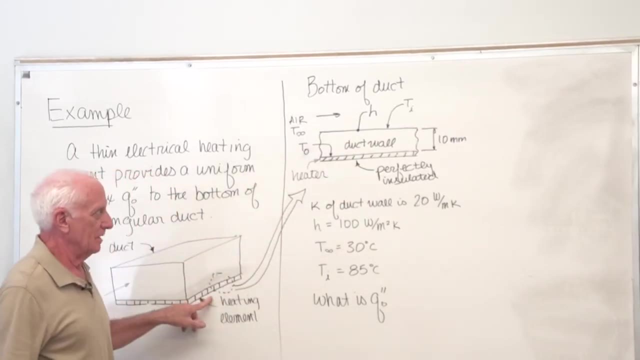 And that's up here. So take a piece of the bottom wall out. Here's the duct wall, bottom duct wall. The heating element is attached to the bottom of the duct wall. Below the heater is perfectly insulated, assumed to be perfectly insulated. 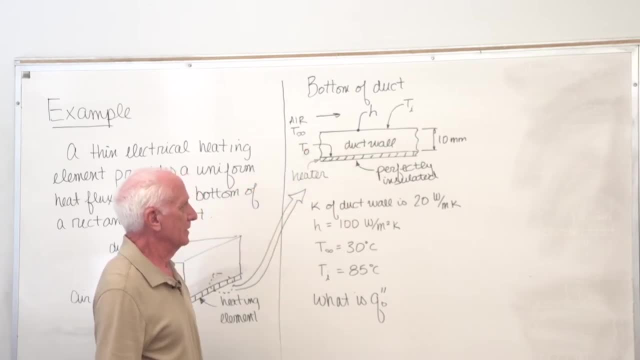 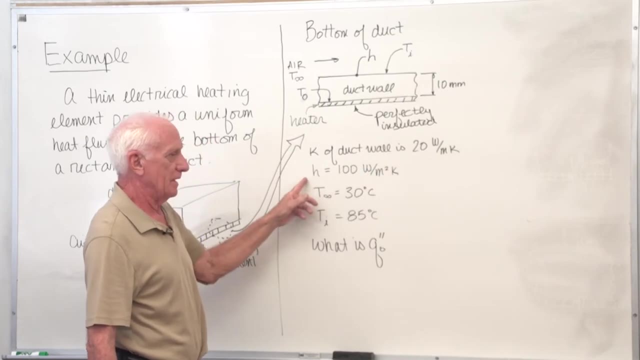 which means no heat gets out the bottom. We're given the duct wall thickness 10 millimeters. We're given the K value of the duct wall 20,. we're given H convection coefficient. we're given the free stream fluid temperature where it's air. 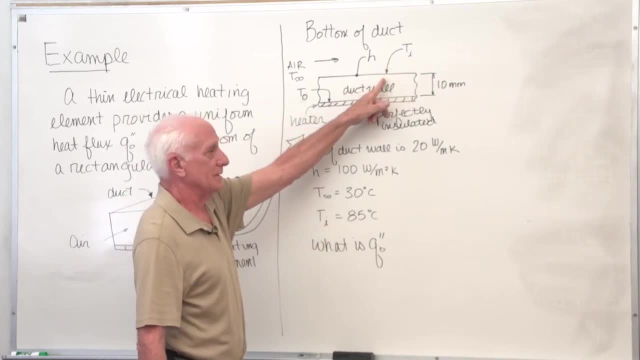 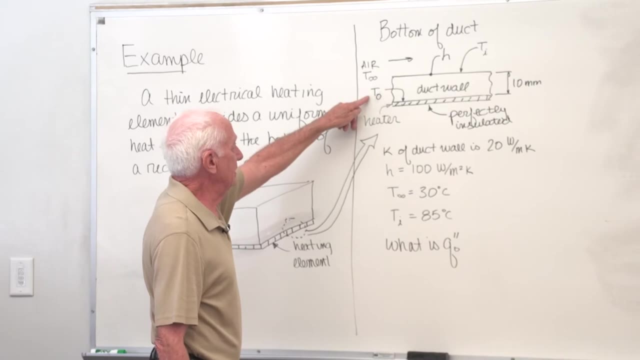 and we're given Ti, which is up here. Ti is the top of the duct wall. Now, this is the bottom of the duct. of course, the bottom of the duct We call T naught the temperature by the heater itself. T naught is the temperature of. 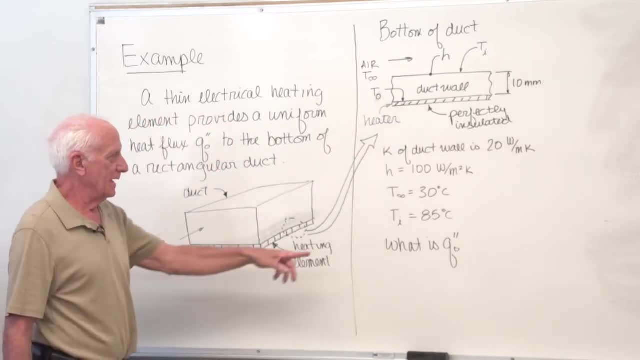 the duct wall at the heater location. We're asked to find what is the necessary heat flux for this problem. the necessary heat flux Q naught double prime. Any questions on the picture? Now we're going to start this by looking. 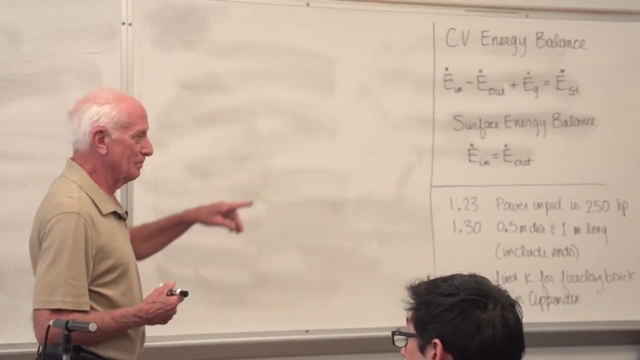 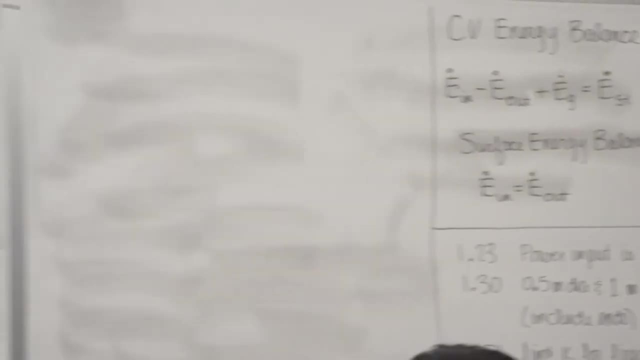 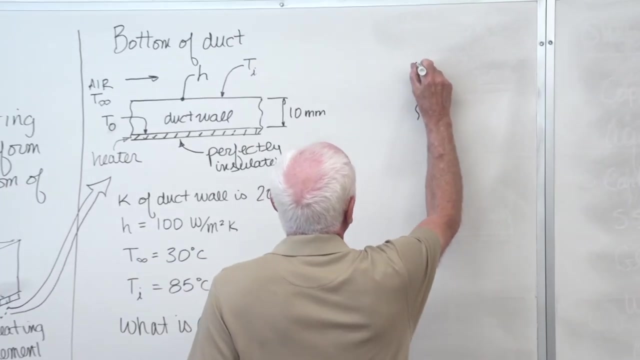 at these energy balance equations. I'm going to start out with the simpler one, the surface energy balance, and I'm going to do that for the. I think I'll do it for the top up here. So I'm going to draw a picture here. 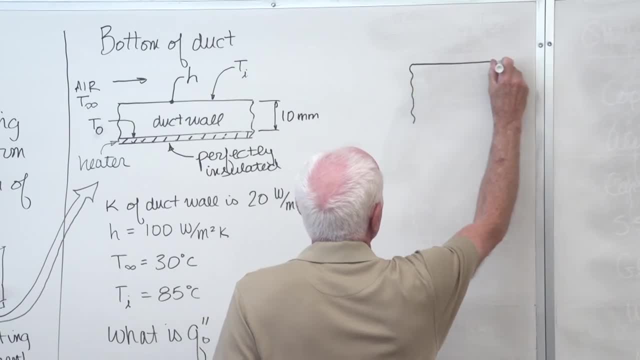 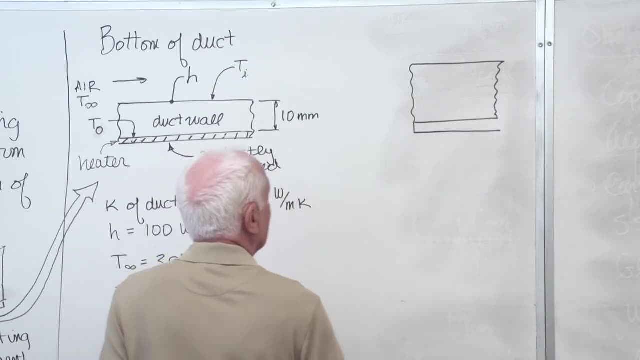 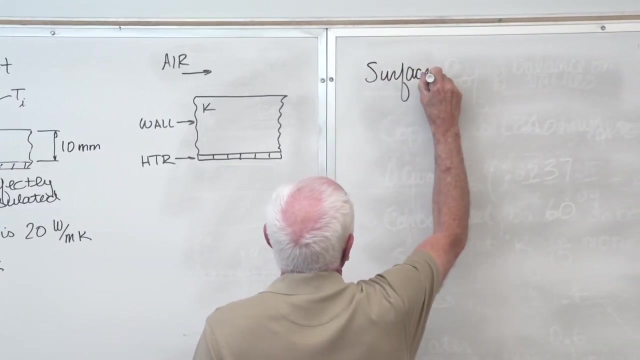 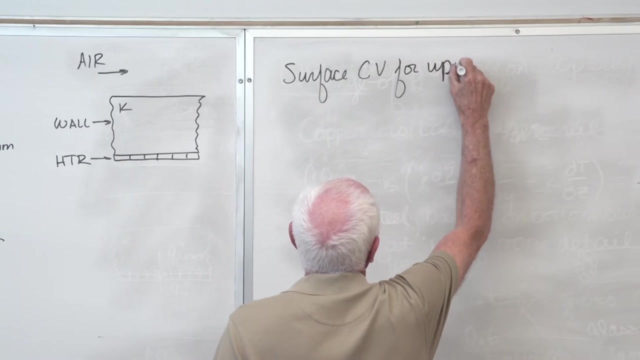 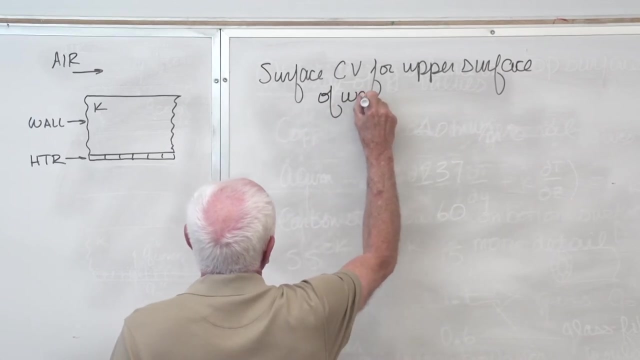 Okay, let's take this like this. So here's the duct wall. That's the duct wall right there. This is the heater Wall. K value: air: My control volume. surface control volume for upper surface. Here's the upper surface. 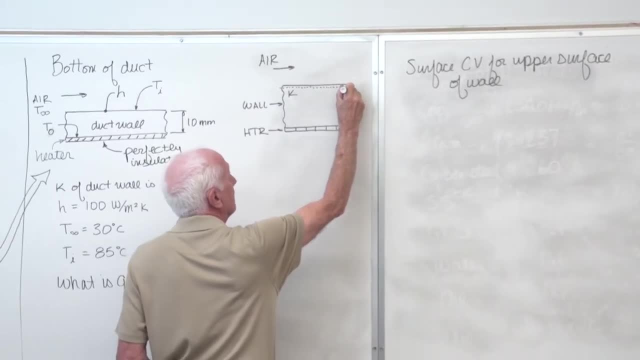 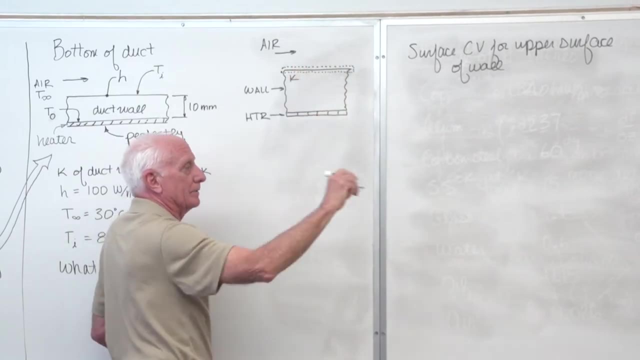 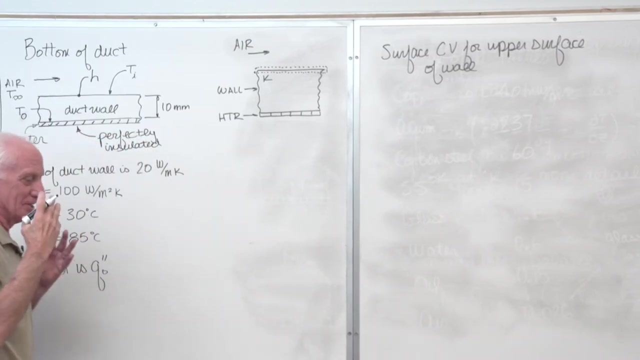 I take my control volume for the upper surface Surface control volume. What comes in goes out. What now, First thing we'll do for any problem is trying to understand what's going on. If you don't understand it, there's very little hope to get. 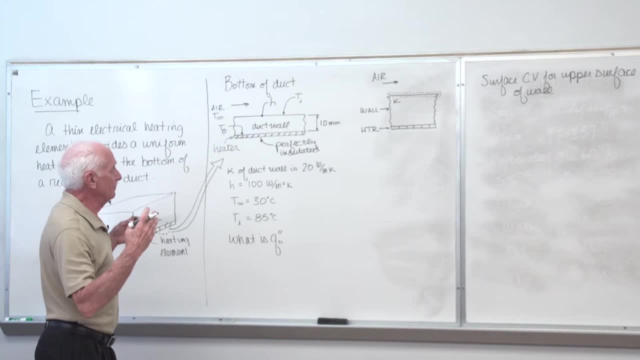 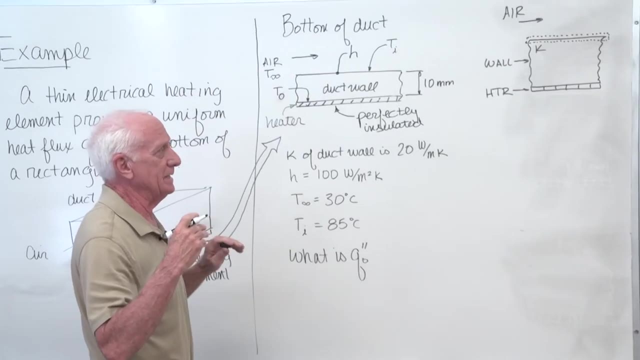 anything solved for correctly. Okay, Heater is hot. of course Heat comes out of the heater. Where do you want to go To the air, to heat the air? To get to the air, What does it have to go through? 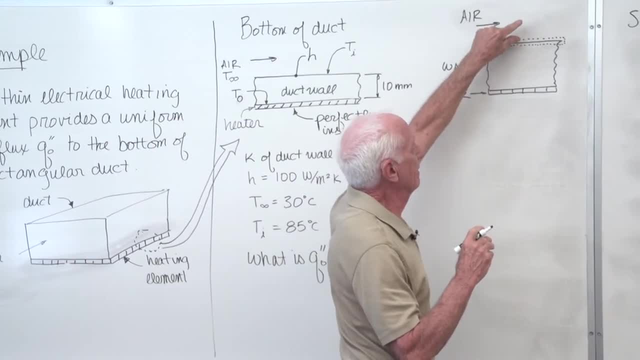 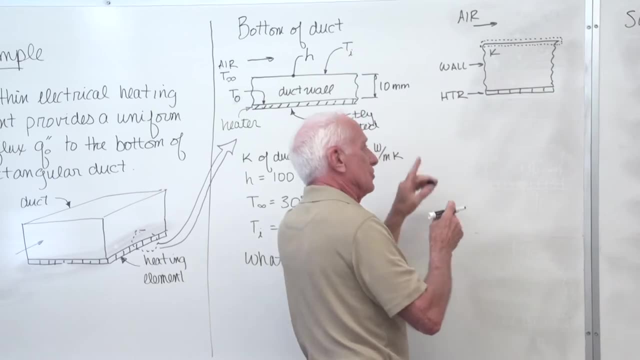 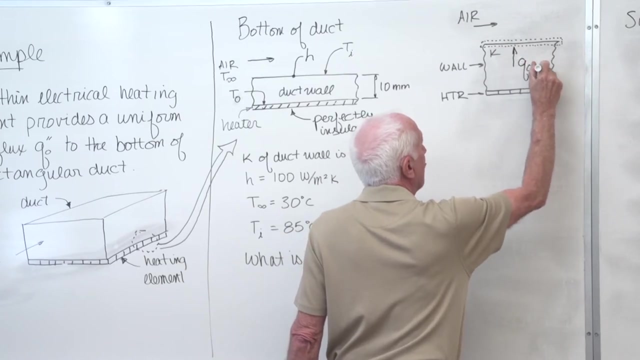 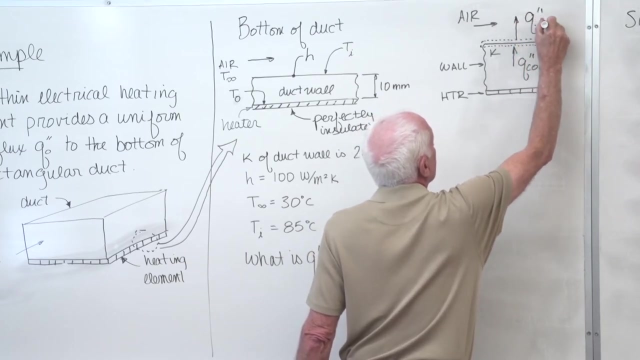 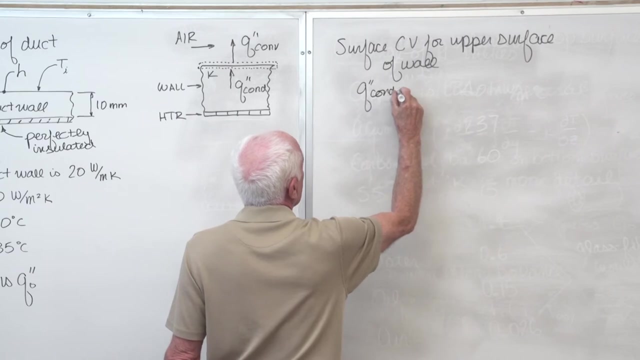 The wall by conduction and convection from the free surface on top. Conduction through the wall, convection to the air. So from my little surface control volume I have conduction coming in And I have convection going out- Q double prime conduction equal Q double prime convection. 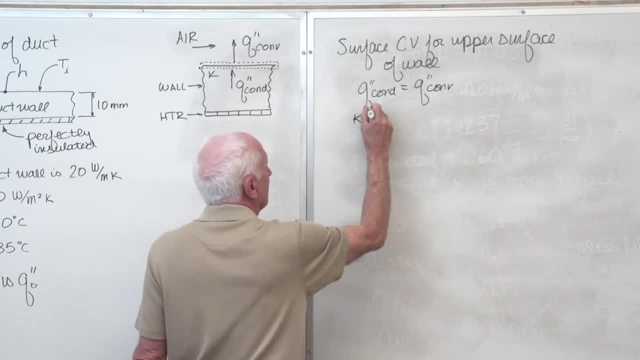 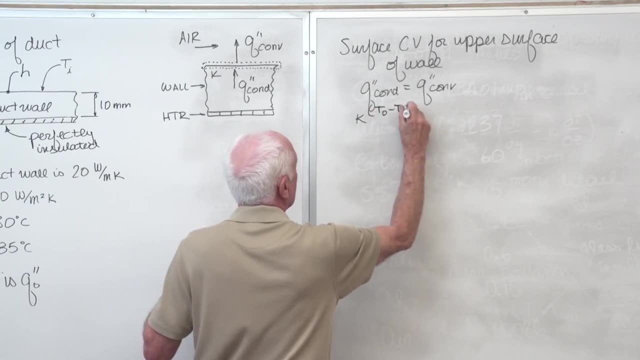 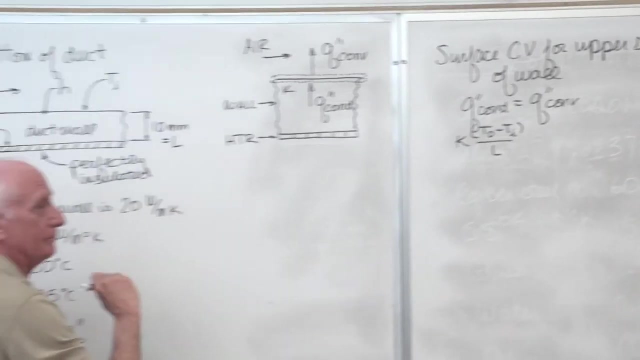 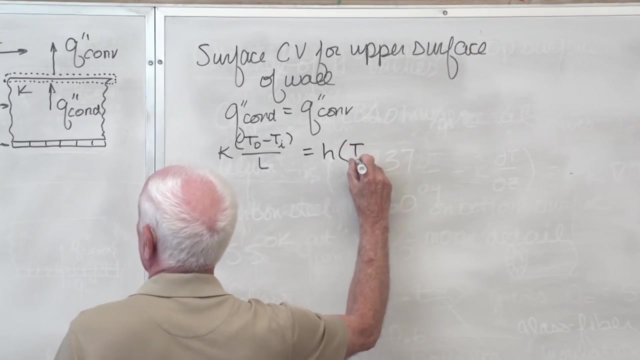 Conduction is K. hot temperature, T naught. Cold temperature, Ti, divided by the length or the thickness of the object. This is L, of course. Convection H, T, surface Ti, T, fluid, T, infinity. 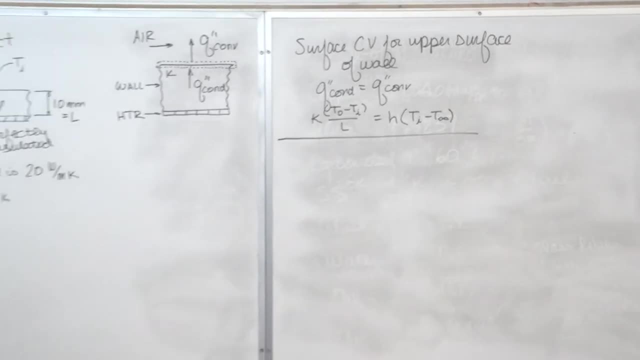 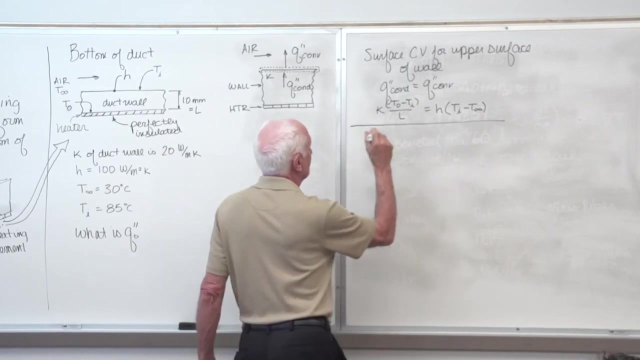 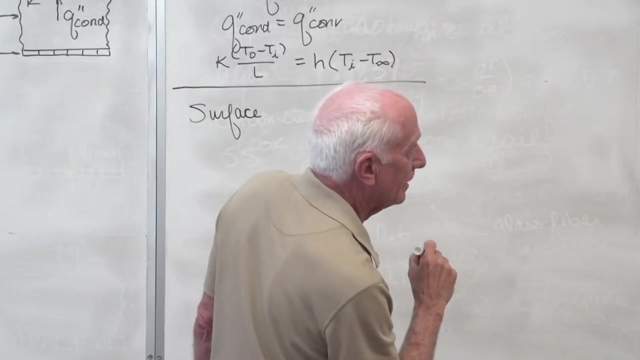 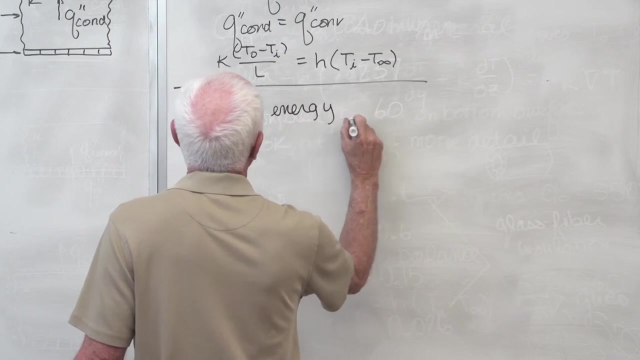 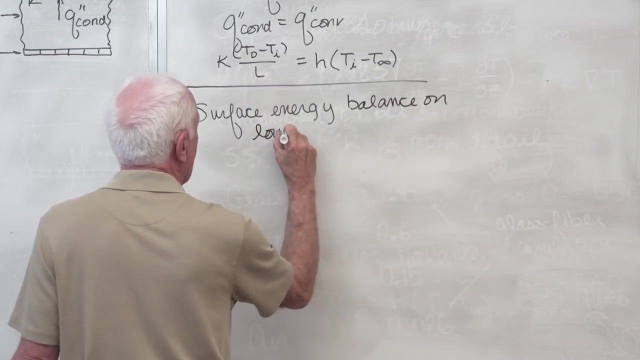 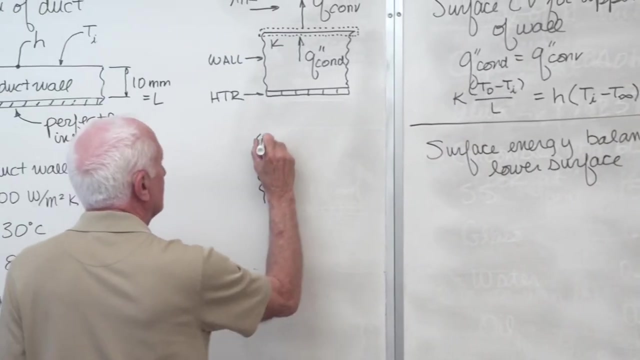 There's my energy balance on the top surface. I'm going to write several of these, So I'm going to just write down the energy balance on the lower surface. So our surface energy balance on the lower surface. All right, same picture. 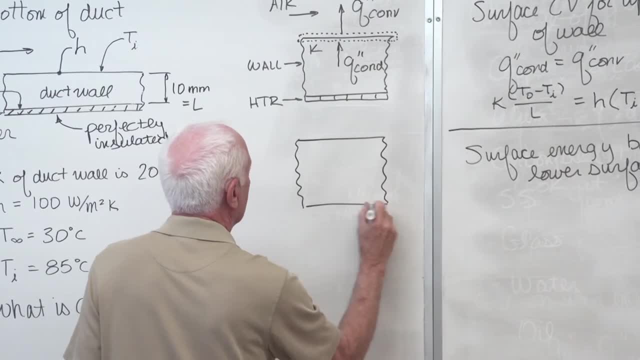 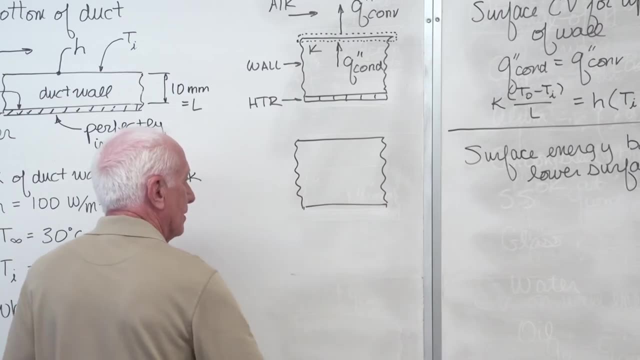 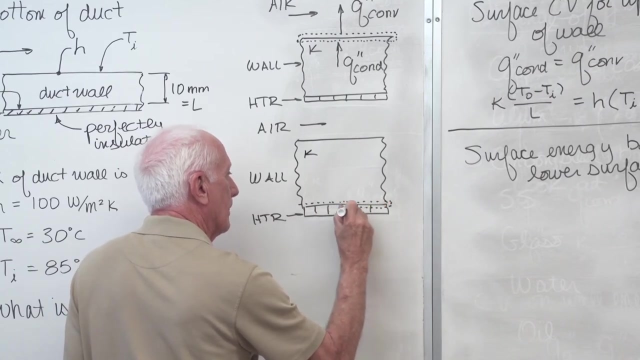 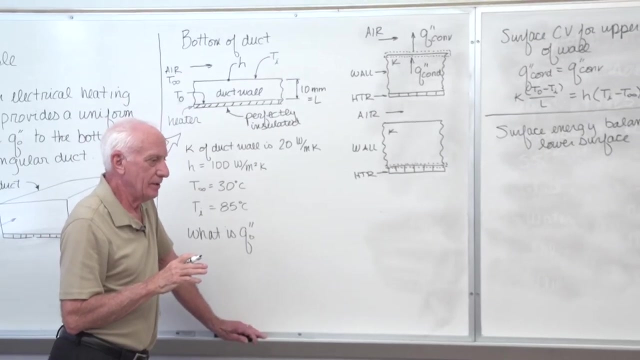 All right, I'm going to make this a little bigger so you can see it more clearly. Heater wall air. Here's the lower surface control volume, All the heat leaving the heater. well, let's put it this way: None of the heat leaving the heater is going to go down. 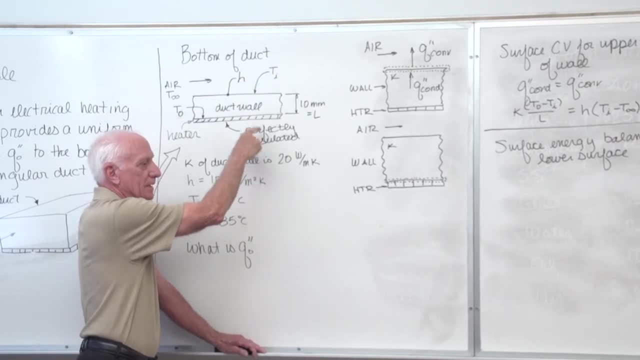 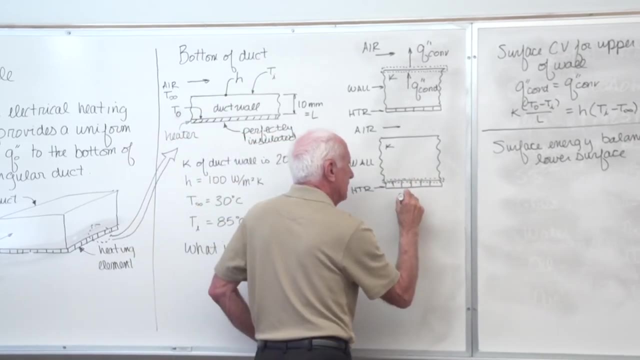 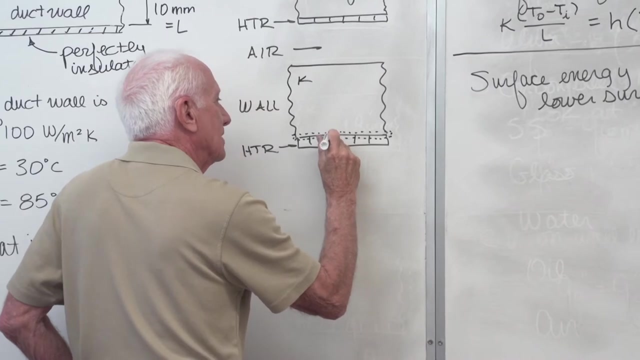 Perfectly insulated means no heat transfer in a downward direction. That means all the heat has to go up into the wall. So what comes into here is into the wall by the heater. So Q naught double prime. Once it gets there, what does it do then? 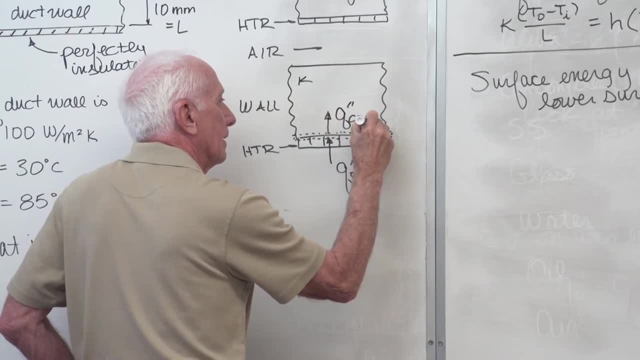 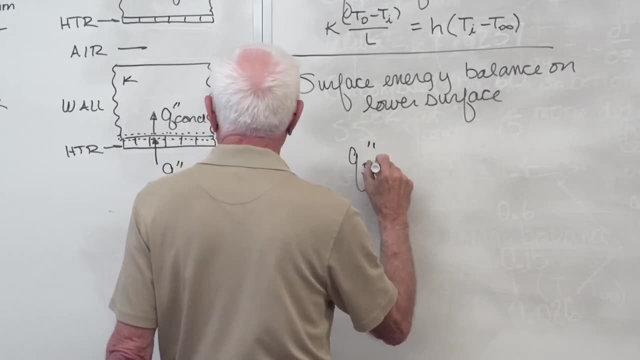 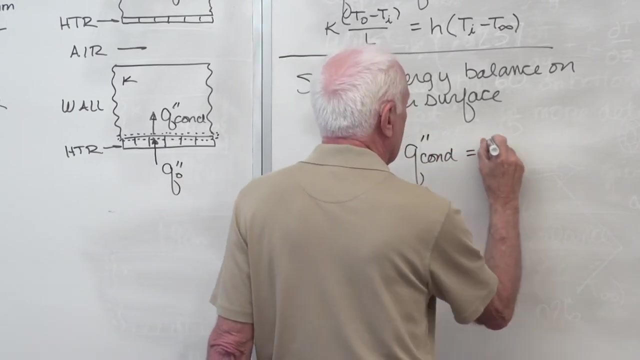 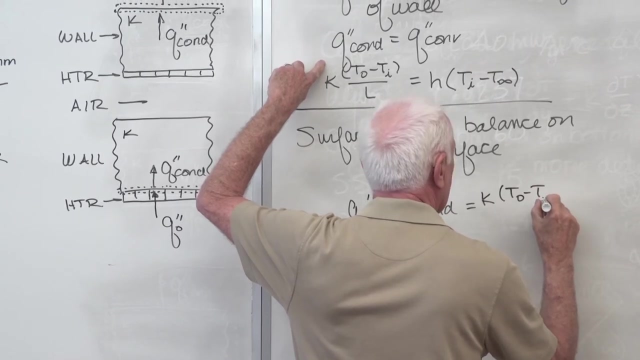 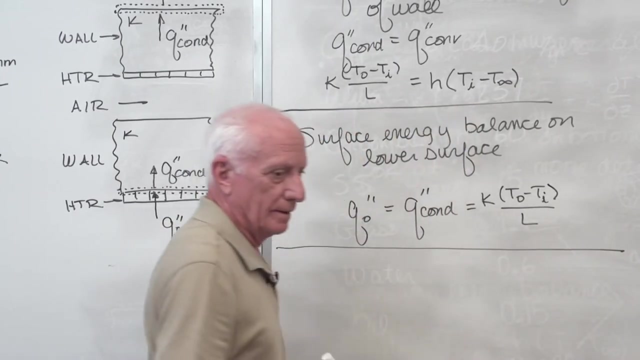 It goes out by conduction Q, double prime conduction. Okay, Q naught double prime equal Q conduction double prime K, same as this T naught minus T and Ti divided by L. I'll write one more. I'll write. 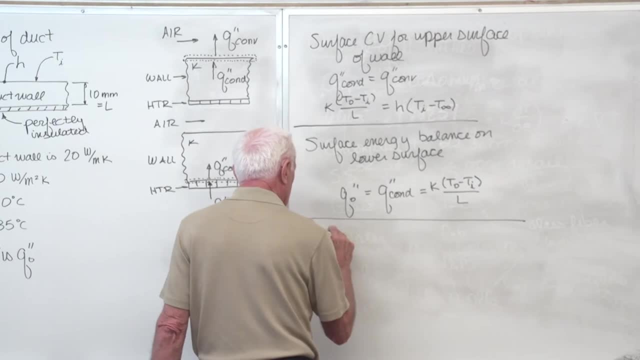 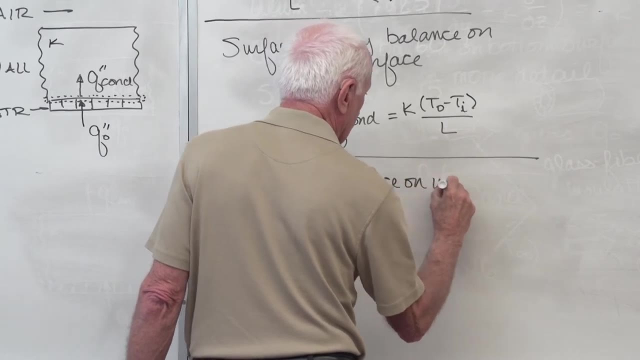 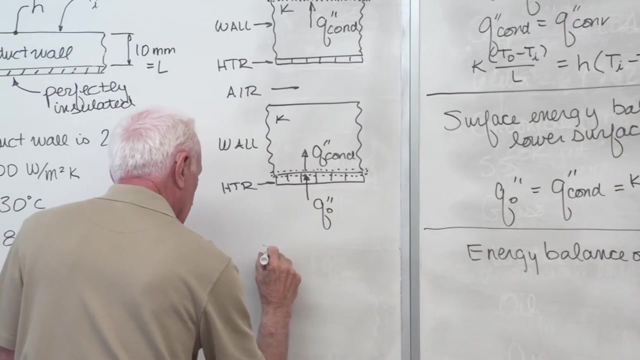 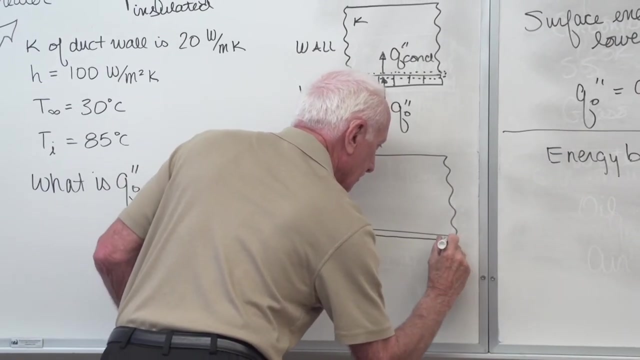 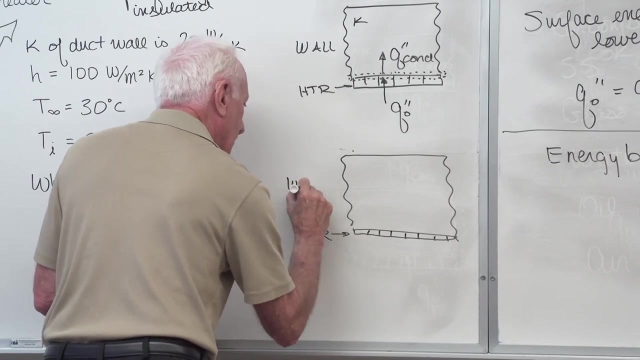 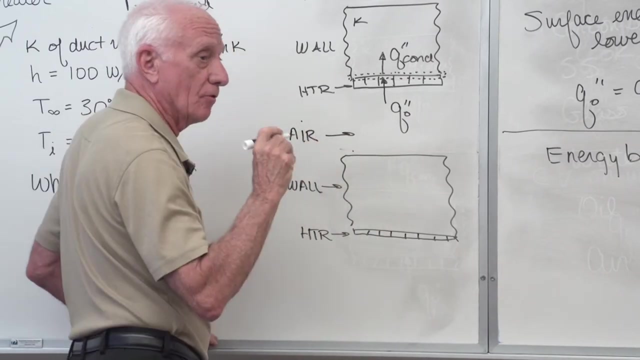 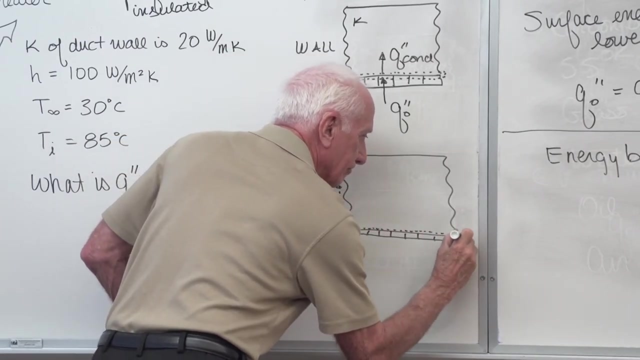 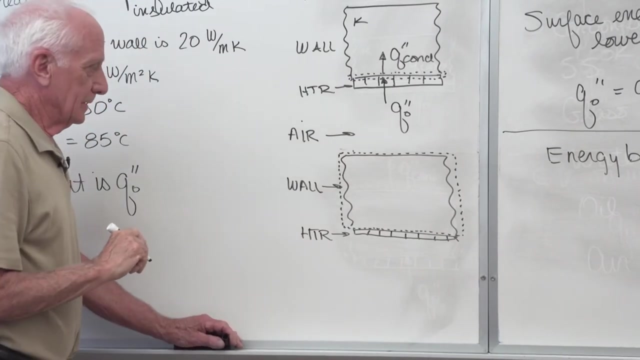 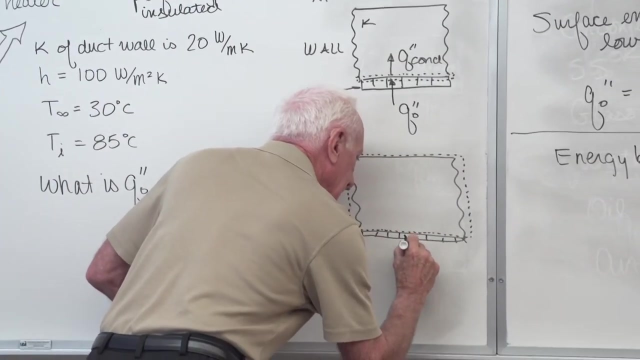 an energy balance on the total wall. So energy balance on the wall control volume: Okay, Heater wall air. Now my control volume is the whole wall. Okay, There it is Okay. What comes in the bottom? It comes in from the heater. 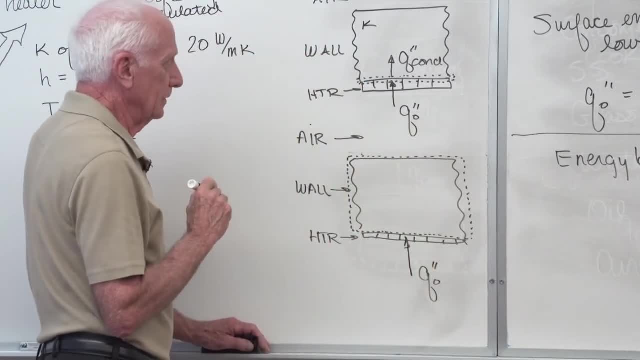 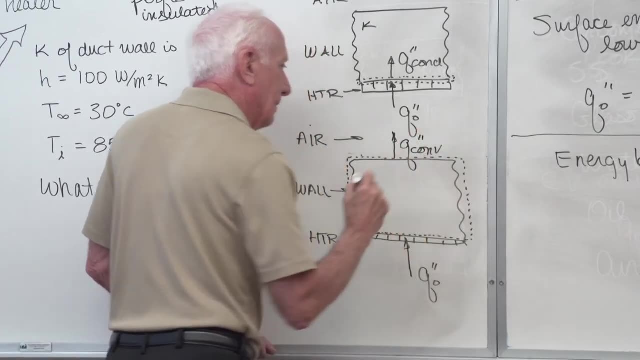 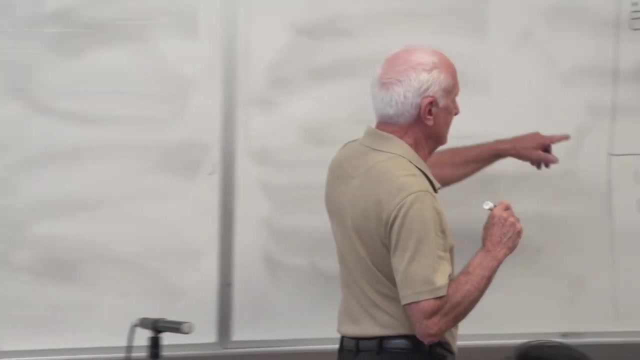 Q naught double prime. What goes out? the top Convection Q convection, double prime. Is there any generation in there? No, Is it steady state Yes: E dot G zero. E dot storage zero. What does that say? 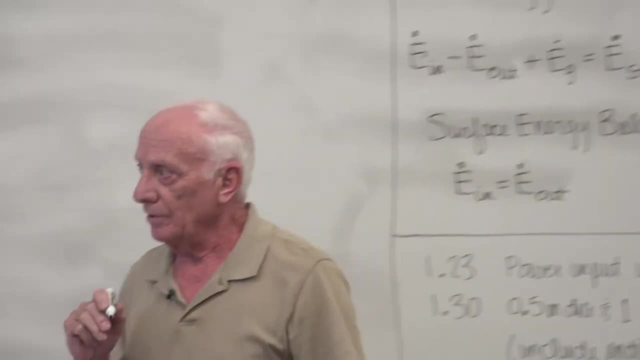 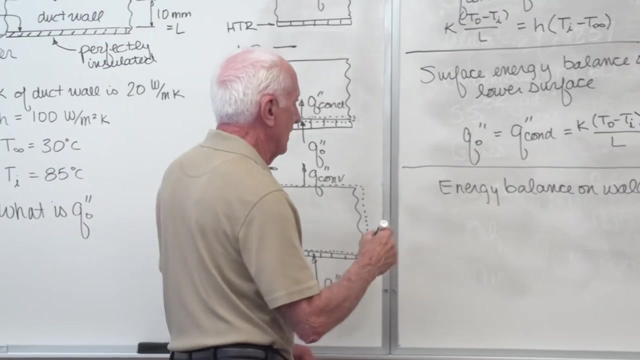 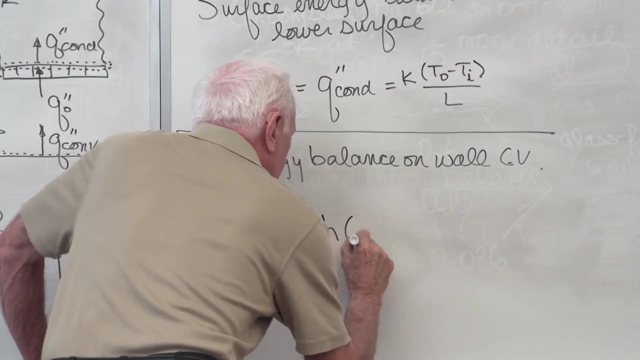 Energy that comes in must equal the energy that goes out. What energy comes in? Q naught double prime. What energy goes out? Q convection double prime. Q naught double prime equal H T. Hot temperature in the wall. Hot temperature is the bottom. 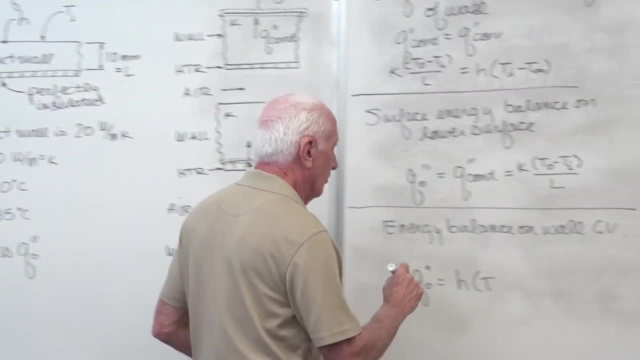 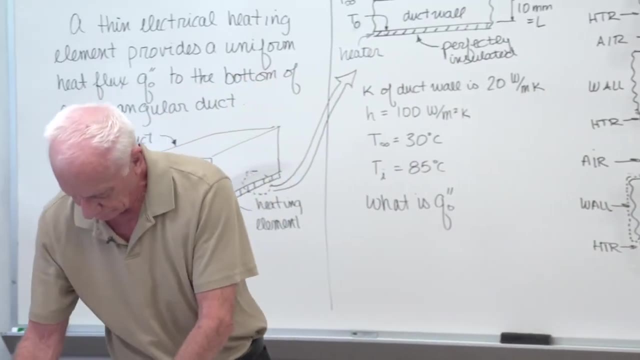 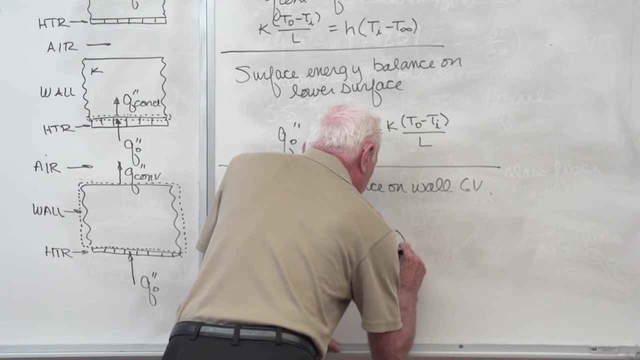 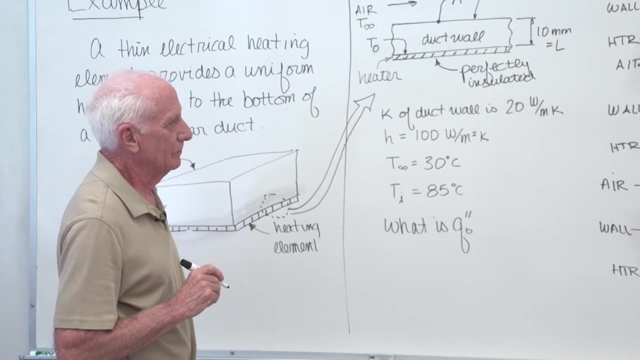 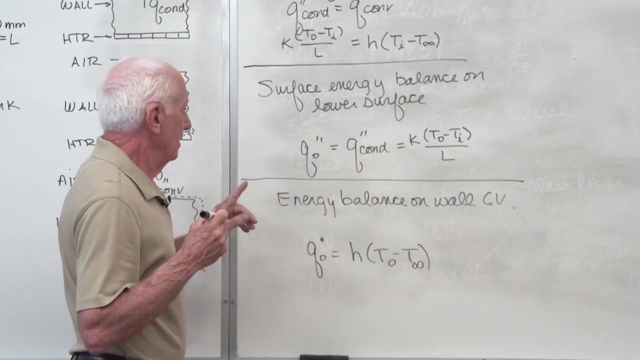 T naught. It's by the heater, of course. T naught Cold temperature, Ti, T, infinity, pardon me, Convection. Okay, Now try and solve for something. Okay, I'm going to take the surface energy balance on the lower surface. 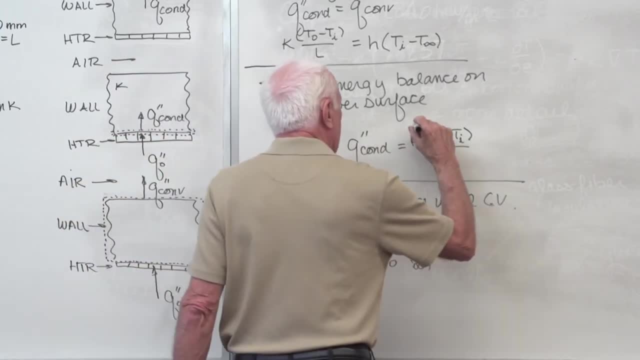 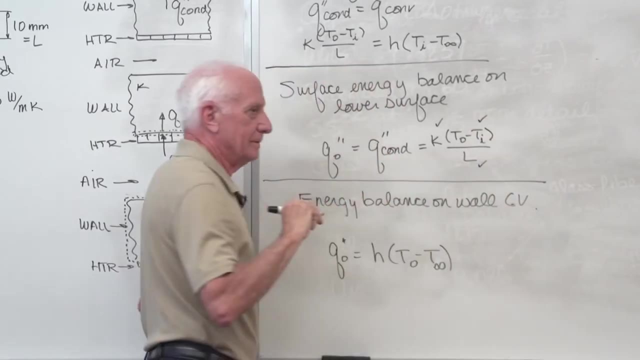 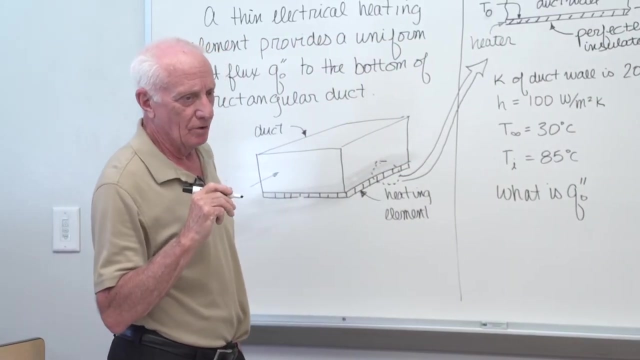 Put a check mark by what you know. I know K, I know Ti, I know L, I don't know T naught and I don't know Q naught. double prime One equation, two unknowns won't work, Sorry, Try again. 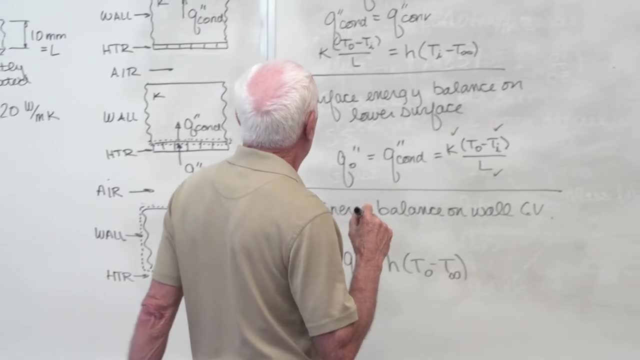 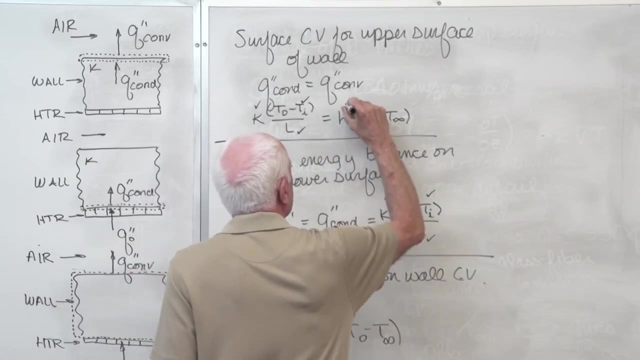 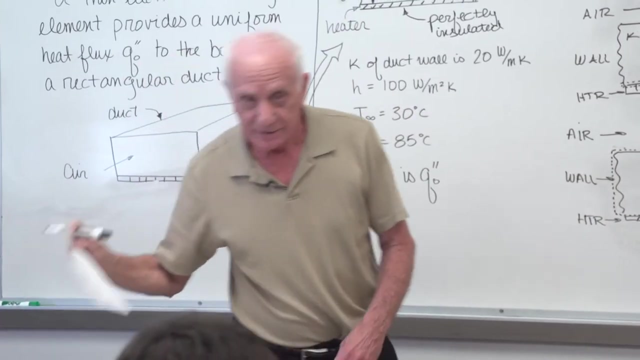 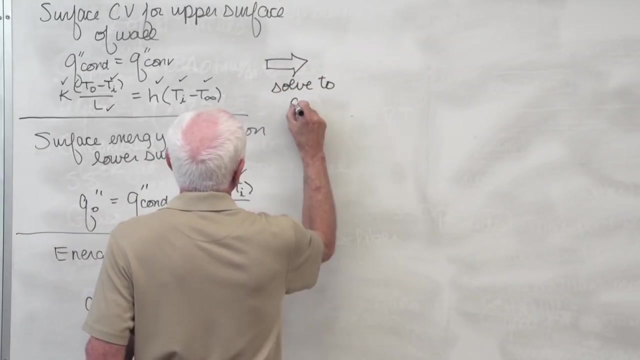 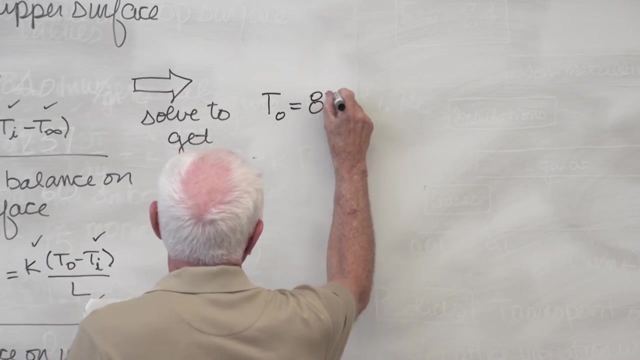 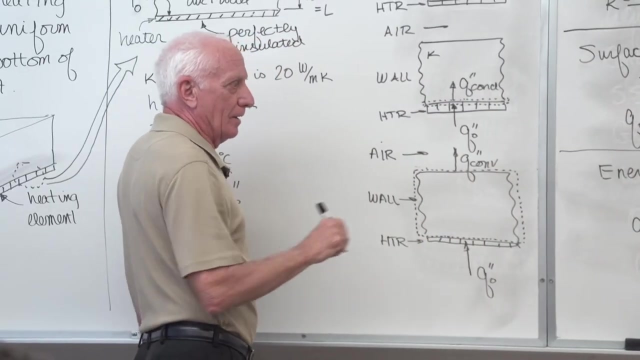 Okay, I'll try this one. then Check mark, check, check, check, check, check, check. One equation, one unknown Good. I like that one. Solve that guy T naught 87.8.. Okay, I think I'll try the last one. 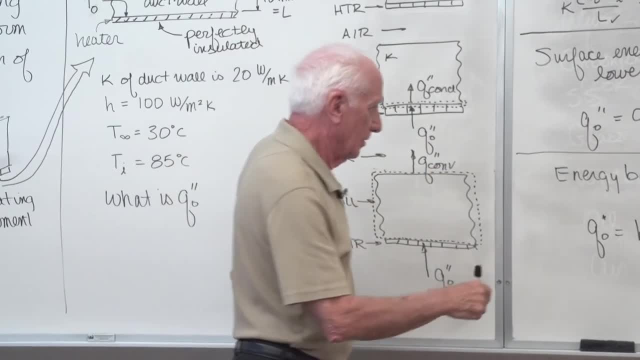 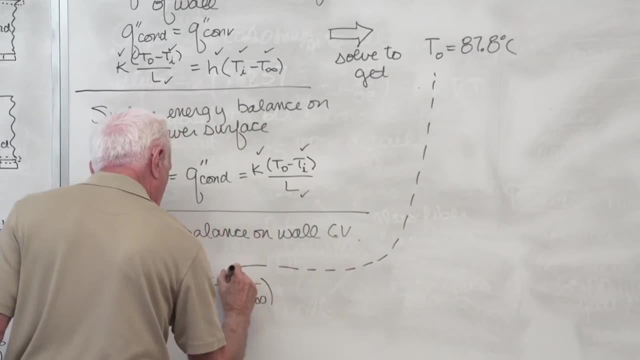 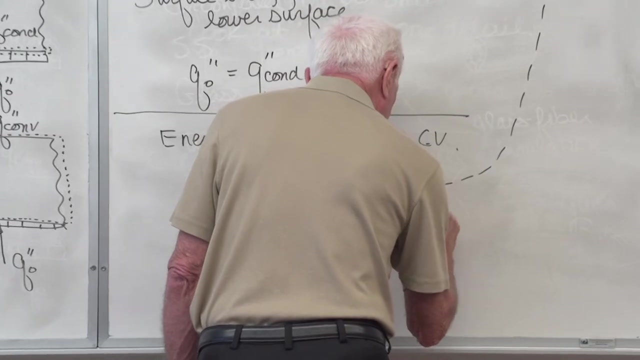 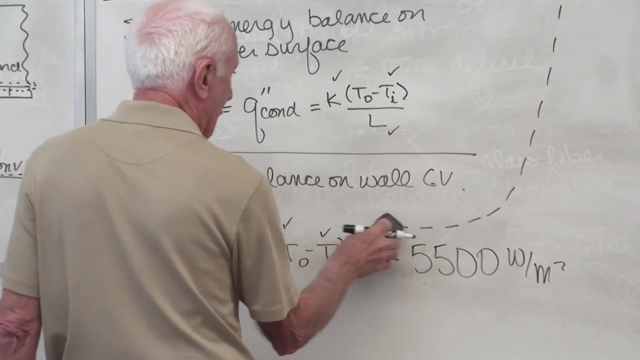 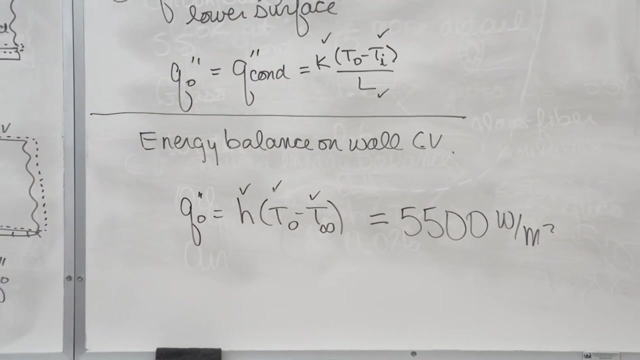 This is a control volume of the whole wall. What do I know H? I know T naught now I know it. Good, Solve for this. Put those guys in there. 5,500 watts per square meter. Now you say, well, how about this one? 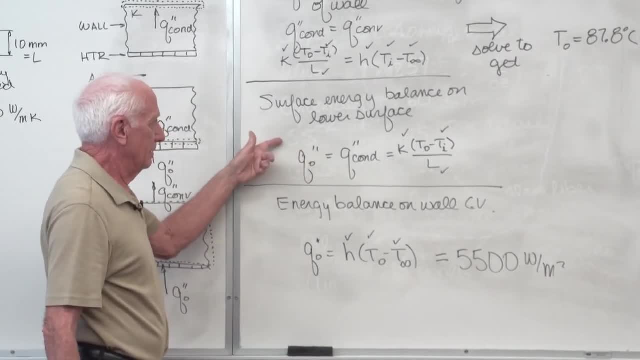 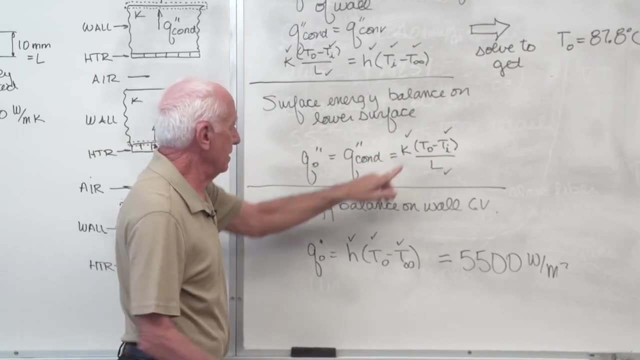 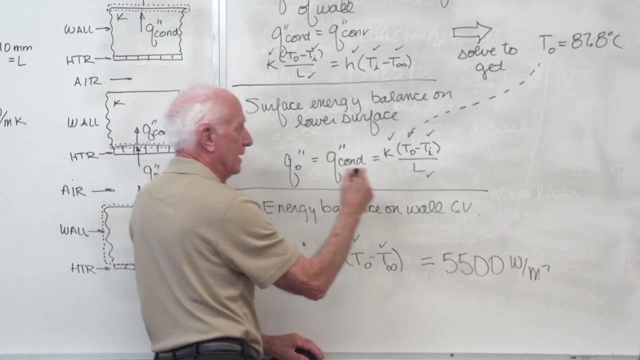 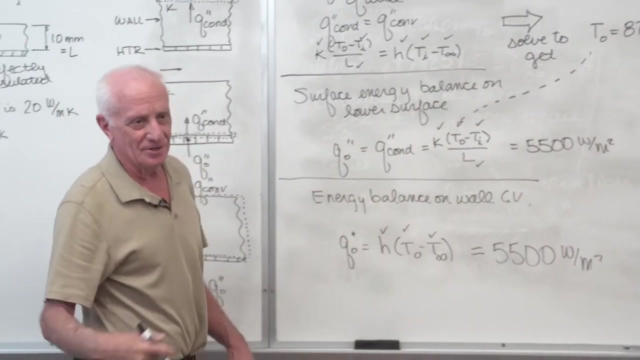 Isn't this a good one too? Sure it is. Once I find T naught, I'll put T naught in here and I'll solve this guy. Okay, Same answer. Well, that's because I wrote three equations. How many unknowns are there? 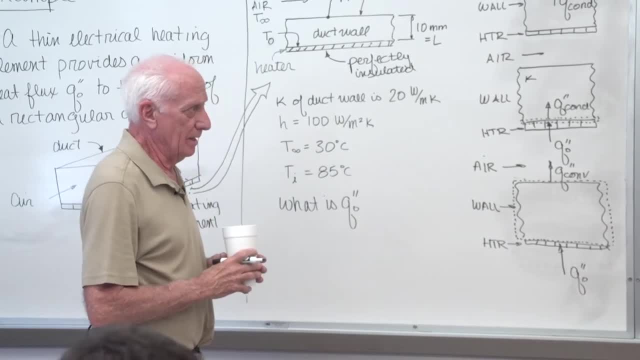 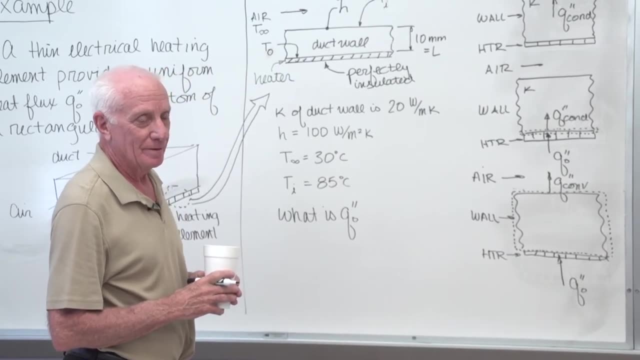 There's two, Q naught, double prime and T naught. How many equations do I need to solve for the two unknowns? Two, I wrote down three just to show you that there's many choices you can make. These equations aren't independent. 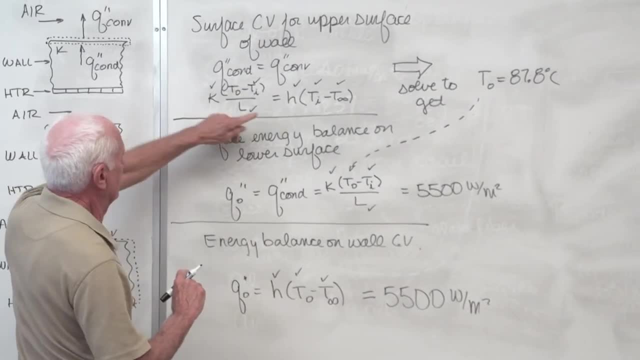 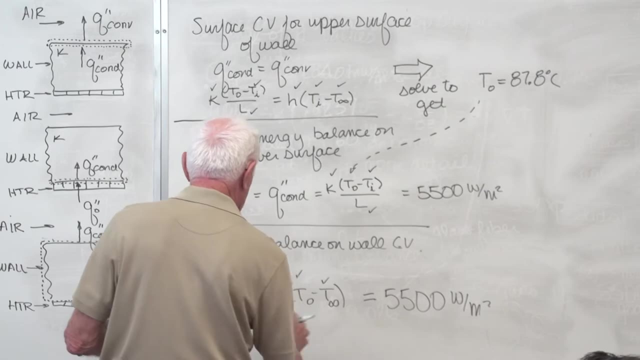 If I take this one and I see the H T, this should be my H wrong there. I got my H T I. I want T I pardon me, That's T I, excuse me, That should be T I up here. 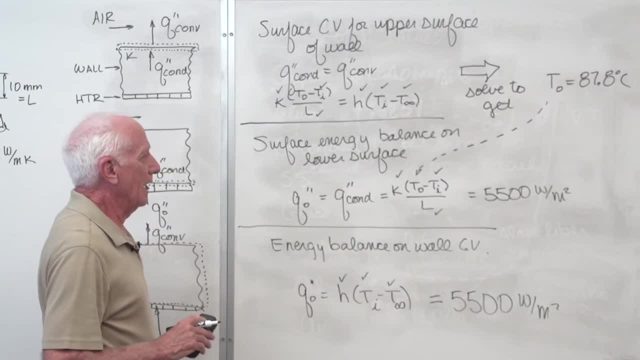 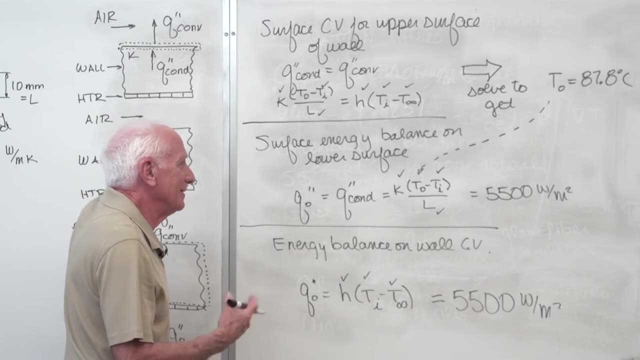 I had the wrong one, That's okay. Same answer If I wanted to. three equations, two unknowns. What does that mean about my equations? They're not independent. If I take this guy- see this term right here- they're the same. 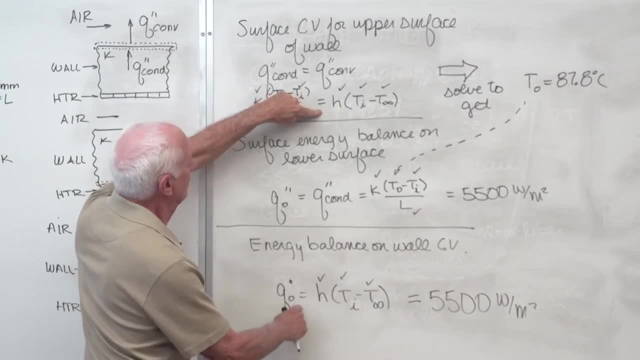 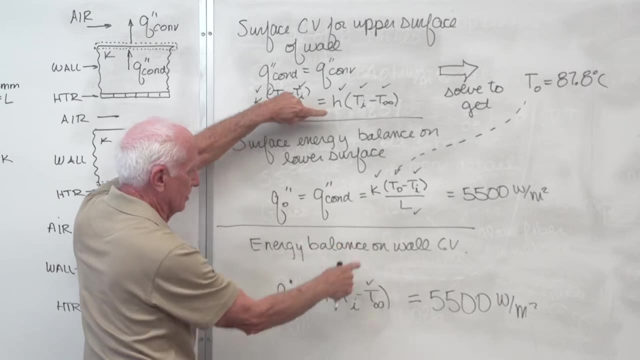 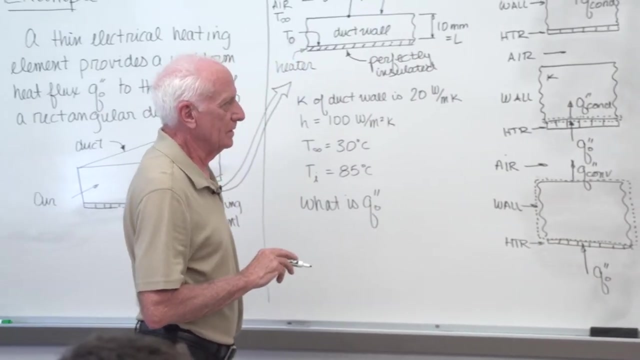 This H is equal to Q naught double prime. Put that up here. This equal Q naught double prime, Same thing. Or you can subtract these two equations and you'll get this equation. They're not independent, But my point is sometimes in. 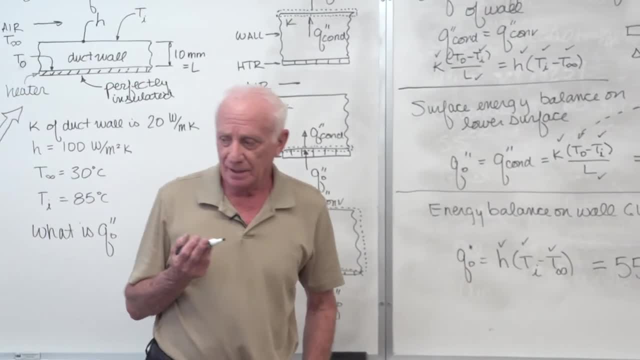 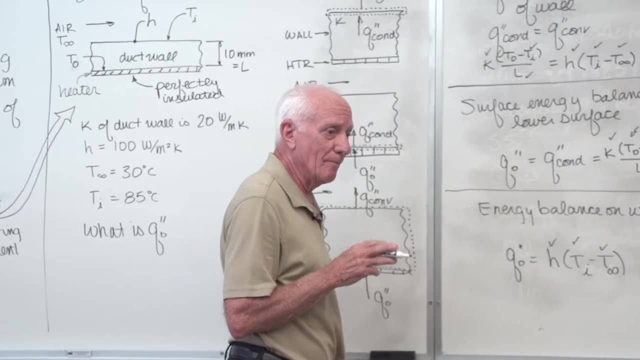 an exam situation in which you're under time stress and you don't know where to start a problem. what you should do is just write down some equations you think might work. Stare at them. You say: I can't solve that guy. There's two unknowns. 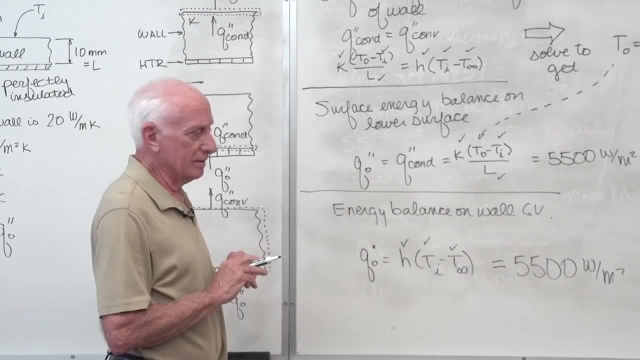 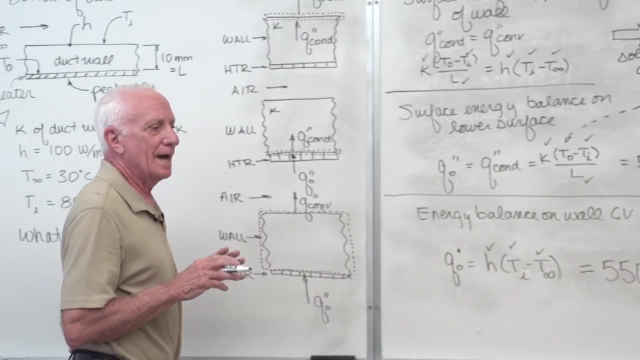 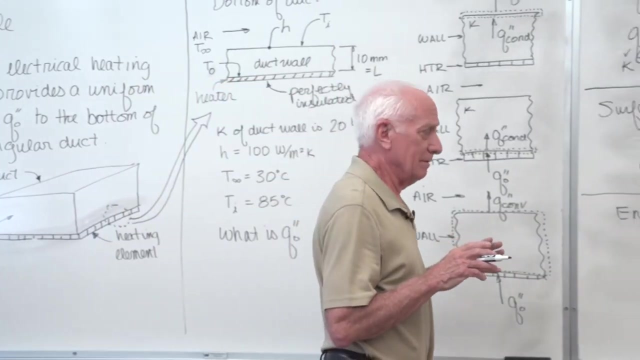 Okay, fine, Stop Write another equation down. Look at it, This one, Yeah, I got him. Then I'll take that answer and I'll put it down here. That helps you to write equations down on exam. You don't get quite as stressed on exam if you stare at them. 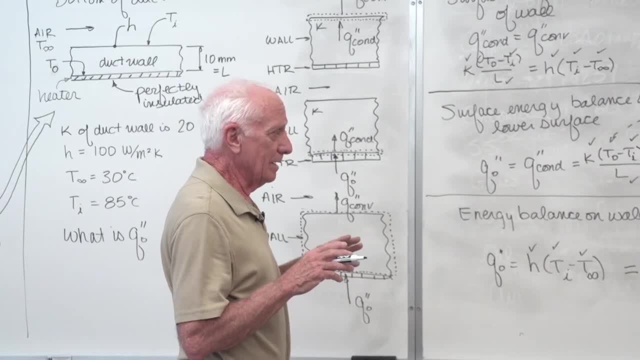 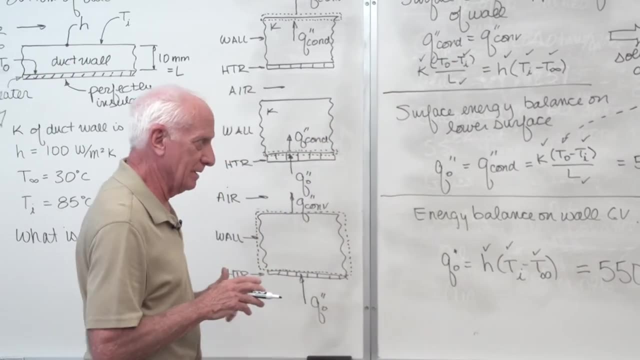 Then you might say: I don't see it right now, That's okay, Come back in 15 minutes. Then the answer might be: oh, now I see it, But writing the equations down is critically important. So three different control volumes. 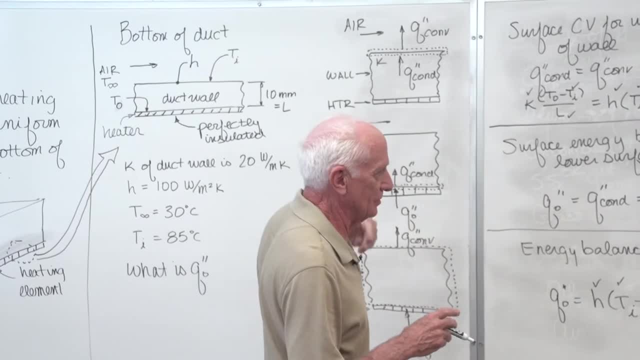 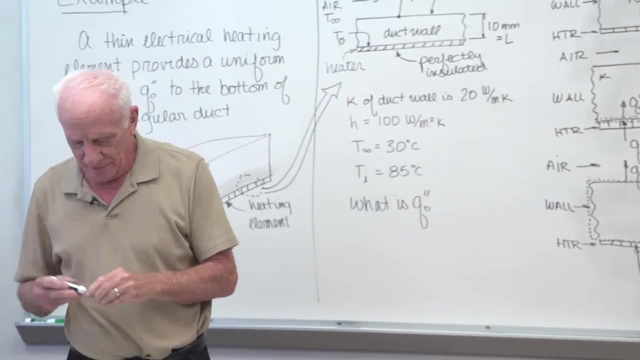 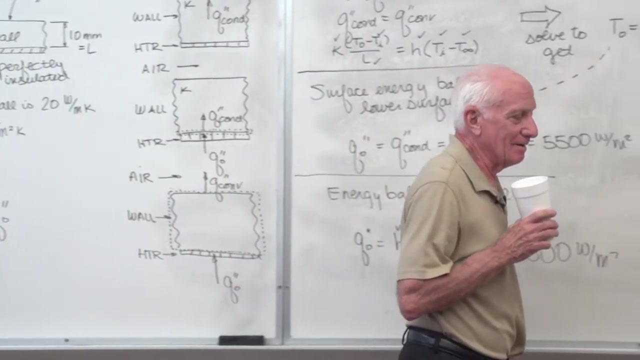 two surface and one that's control surfaces and one's a control volume. So that ends up Chapter 1.. Now we spend the next four chapters- two, three, four and five- on conduction. That's a long time, because conduction is very important. 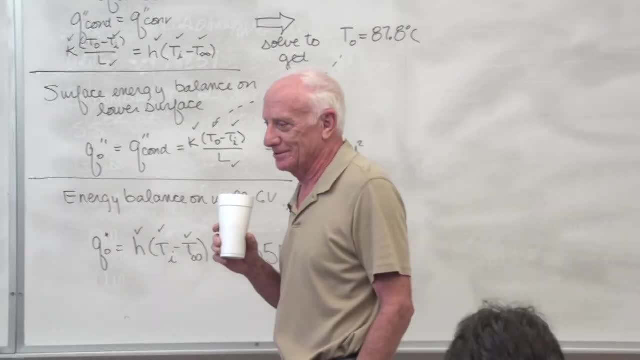 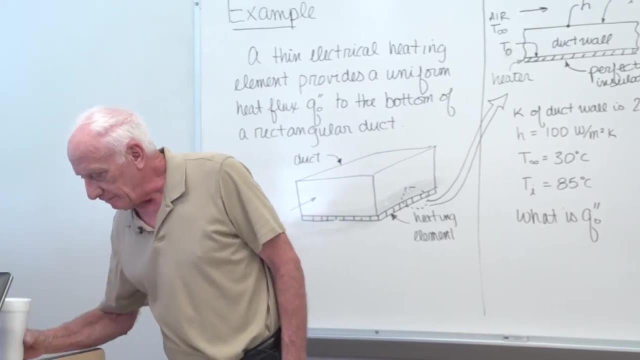 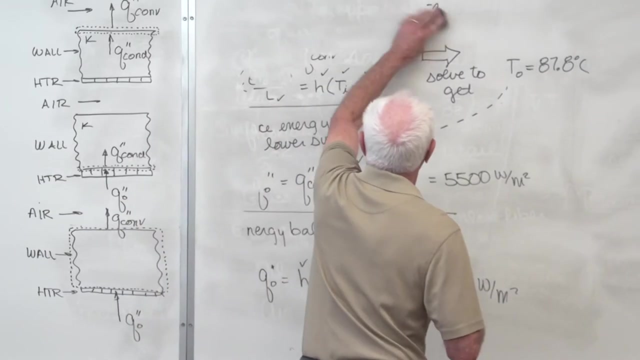 Chapter 2 is titled Introduction to Conduction. of course Okay, So we're going to look at that first. So first thing in Chapter 2.. In Chapter 1, we pretty much treated Fourier's law in one dimension, In our case it was x. 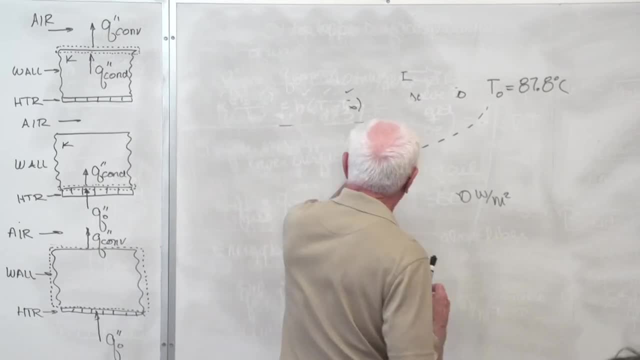 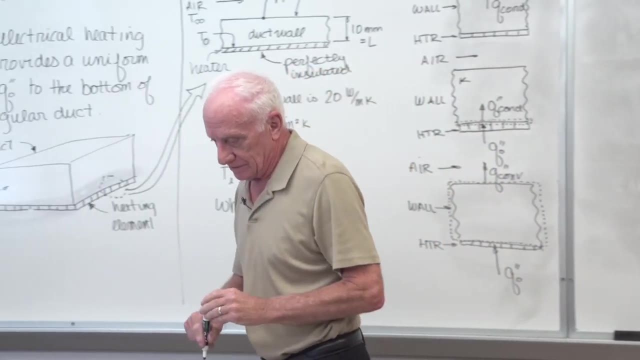 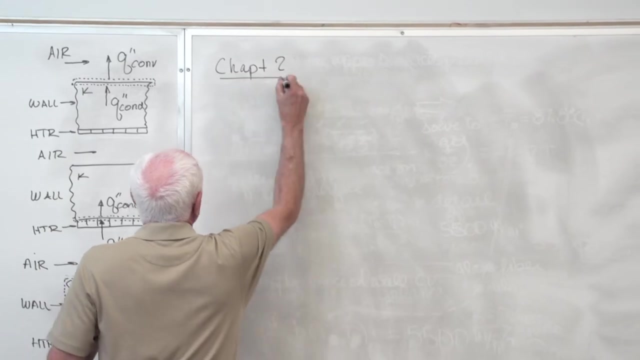 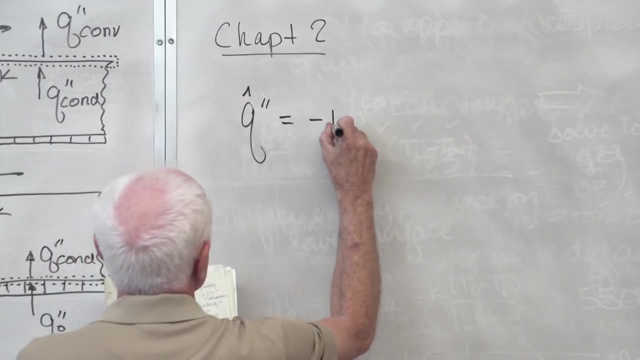 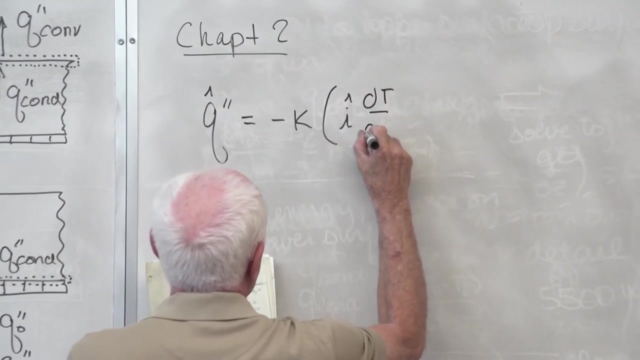 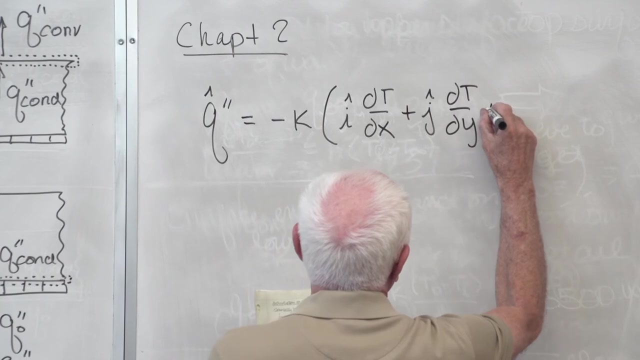 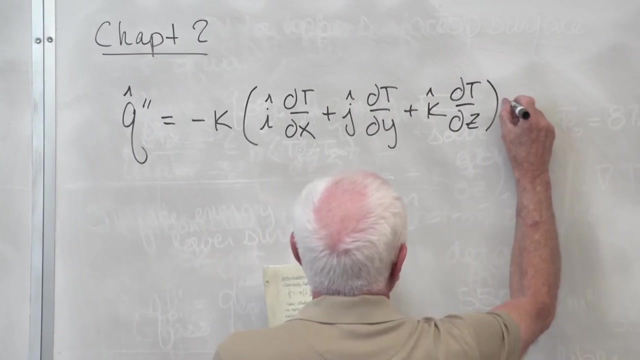 But in general, heat conduction is in three Different directions, in rectangular x, y and z. So let's start out with Chapter 2, then Q, double prime. this is the vector notation minus k, unit vector i Or in shorthand, vector notation. 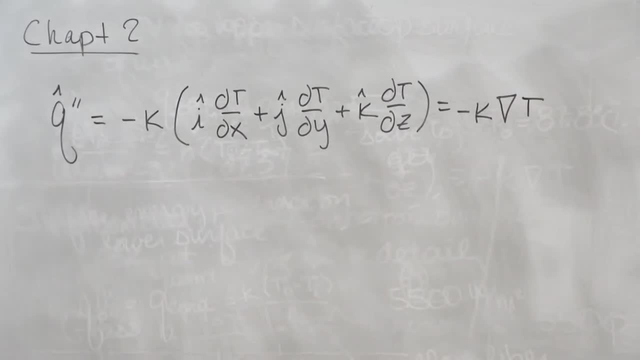 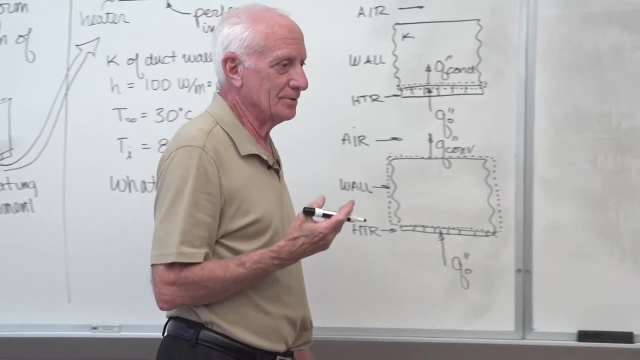 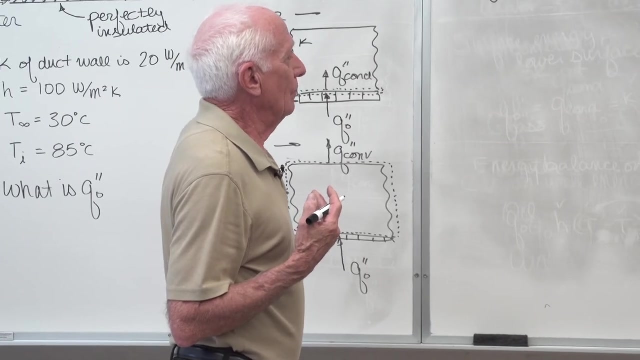 the del operator, k, del t. So in general conduction, of course we know that occurs in three directions: x, y and z. in a typical solid, rectangular solid. We're going to pretty much focus on 1D, heat conduction. 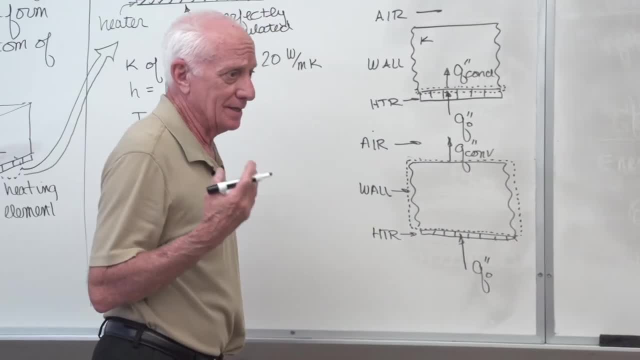 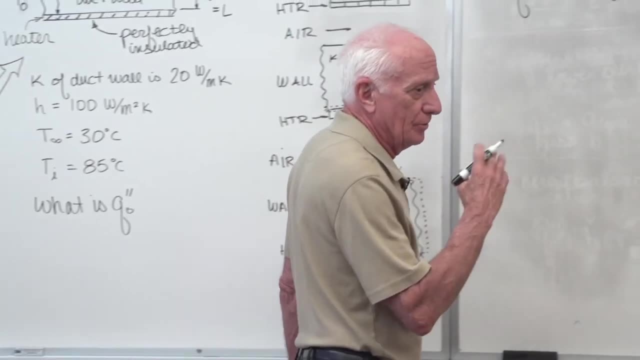 although in Chapter 4, we will look at 2D heat conduction. That's as deep as we go into conduction 1, Chapter 4 on two-dimensional conduction. But we won't do any 3D stuff in this first introductory course to heat transfer. 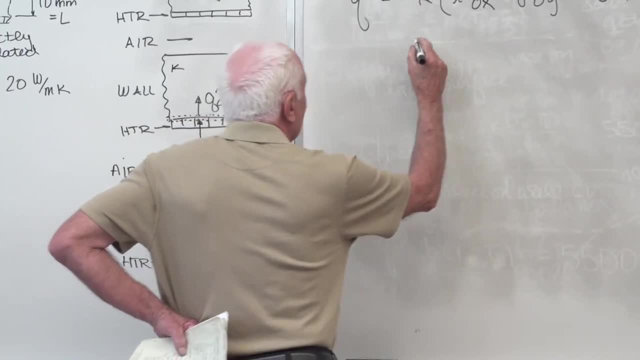 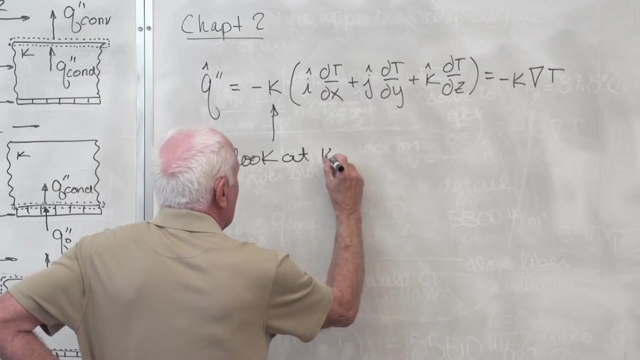 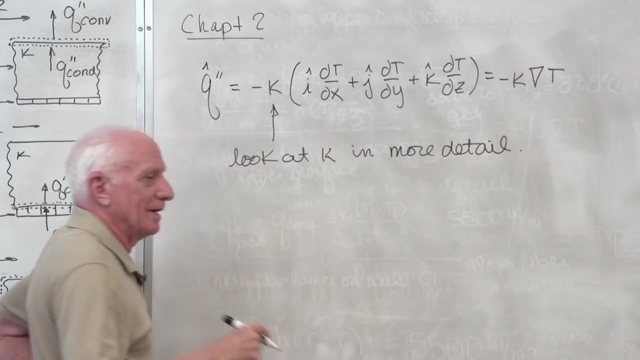 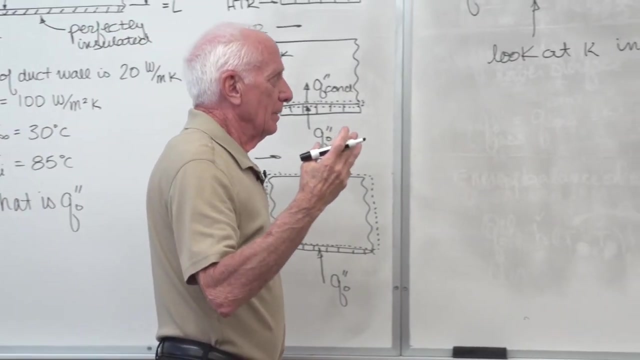 So now we're going to look at k in more detail And we looked at it very quickly in Chapter 1.. We said k is a thermal conductivity, a property of the material. I told you it's in the back of the book. 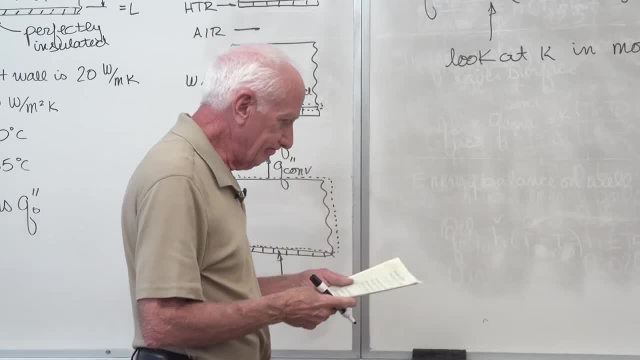 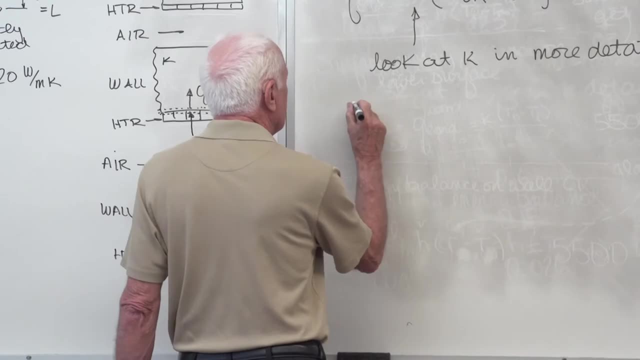 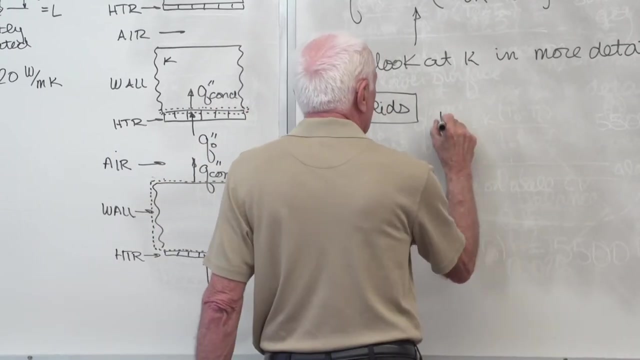 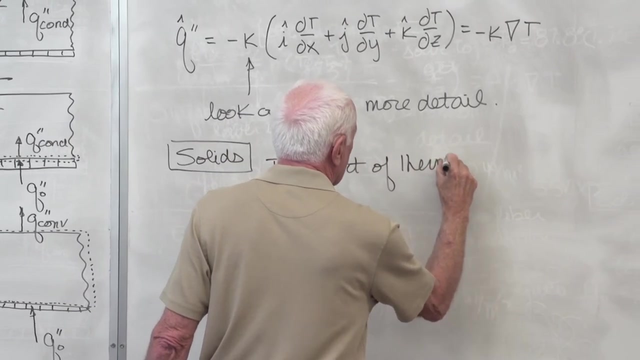 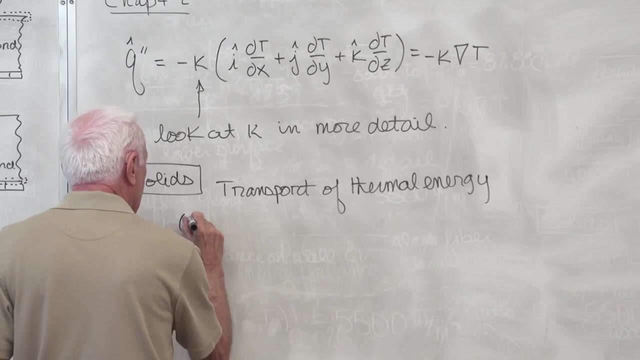 but in Chapter 1, they give you the values for the homework problems. So let's see what k means in a solid. So we'll look at solids First. transport of thermal energy by two modes. First, lattice vibrations. 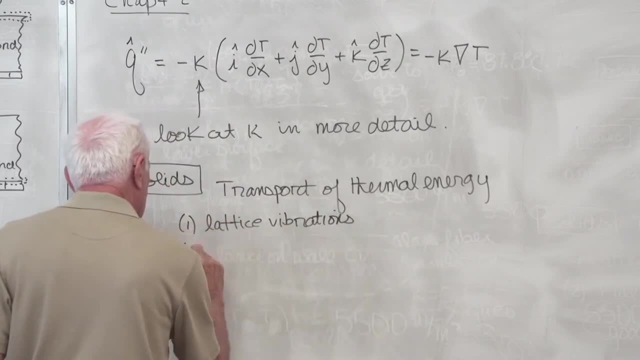 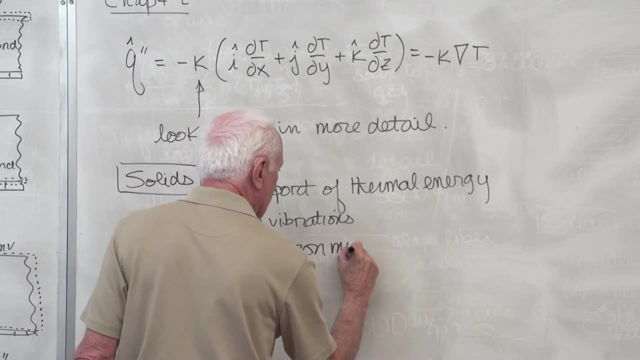 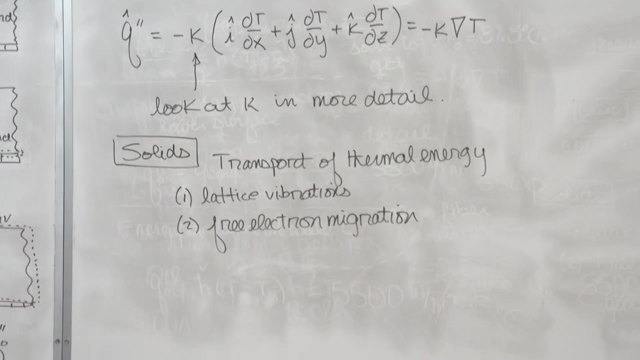 3D heat conduction. 3D heat conduction, two free electron migration, If it's a solid 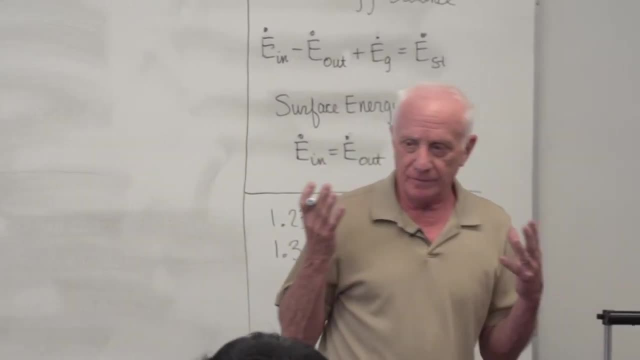 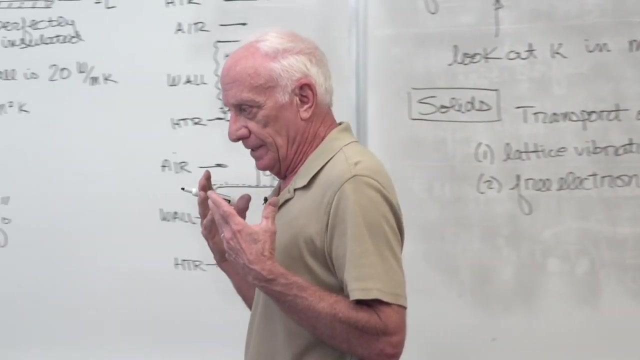 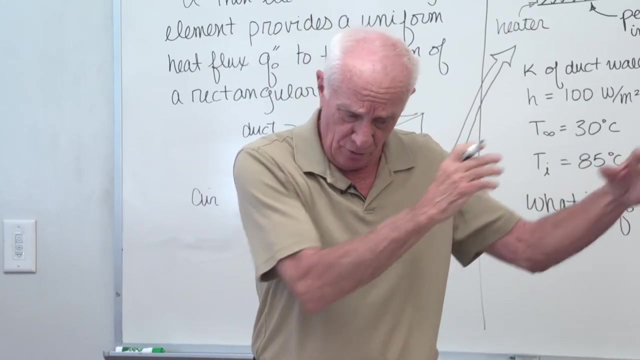 it's a lattice structure. So if the atoms start to vibrate on the lattice structure, then the energy is transported to its neighbors. When it starts to vibrate, neighbor starts to vibrate, and so on, and so on, and so on. 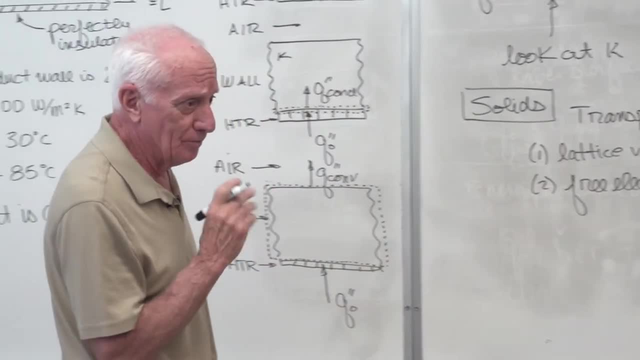 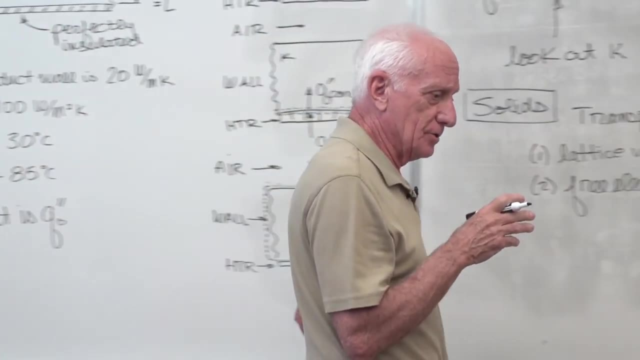 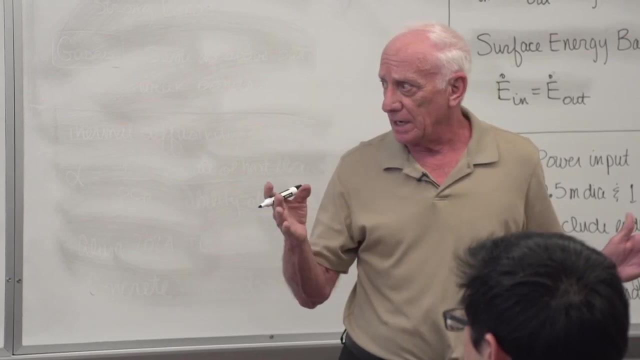 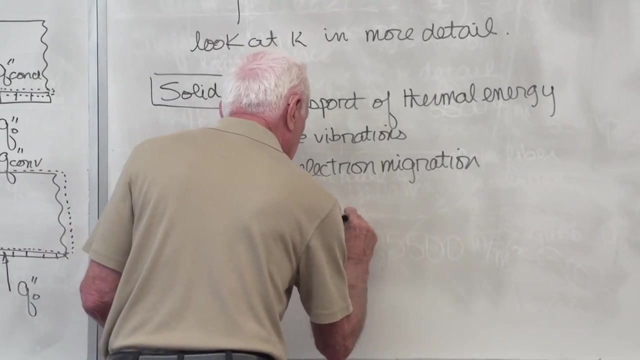 Some solids also have free electrons which help the conduction of thermal energy, because those free electrons have kinetic energy and they bump into others and they transfer that kinetic energy to other electrons. So you get transport of energy that way. These free electrons occur typically in good electrical conductors. 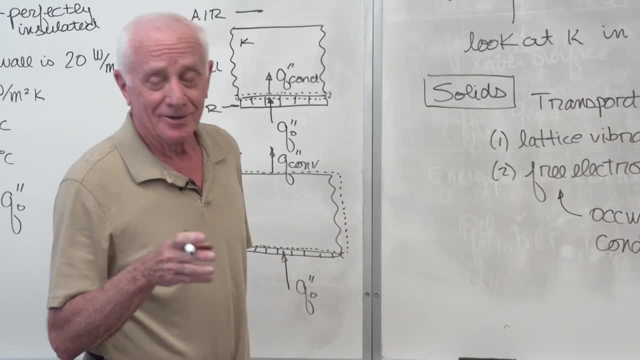 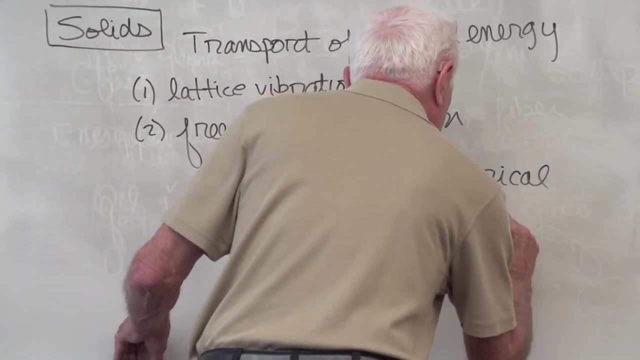 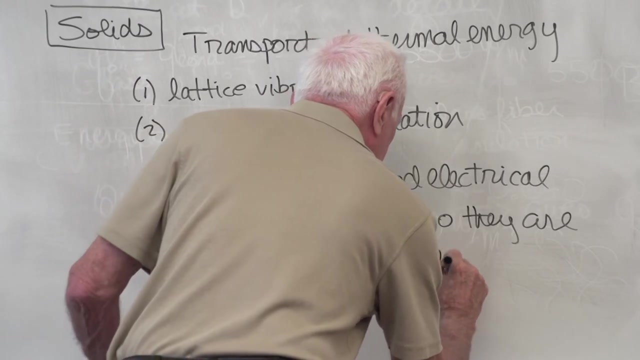 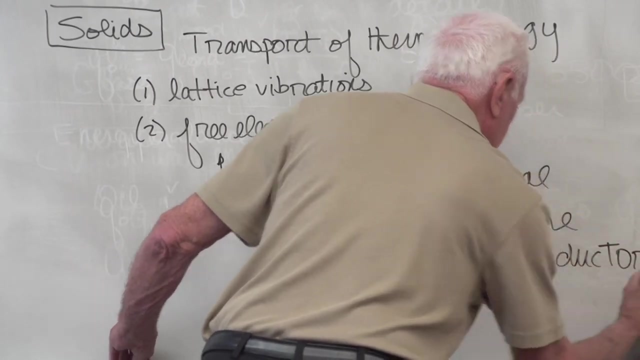 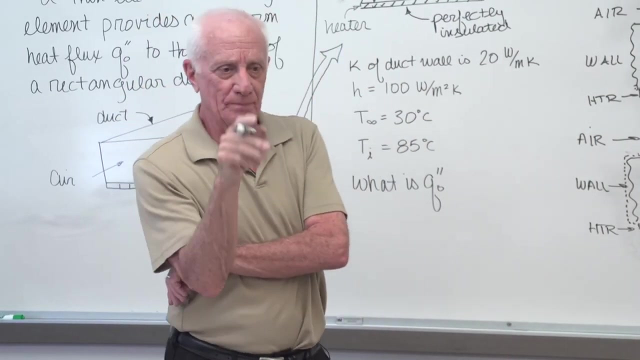 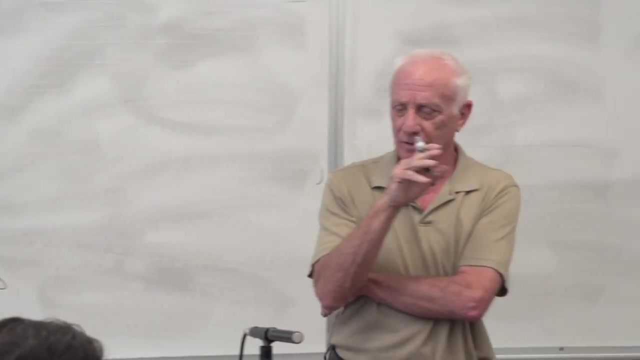 So a good electrical conductor turns out to be also a good thermal conductor. So copper wires, great electrical conductor. What does that mean? I expect copper wires to be good thermal conductors. Of course it's good. Copper conducts heat really well. 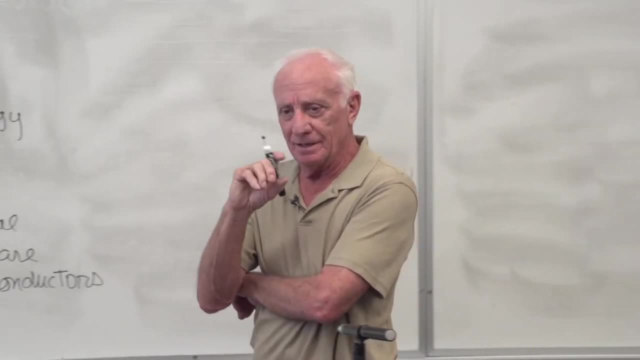 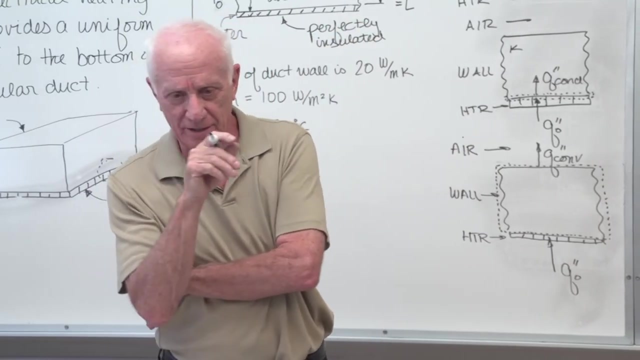 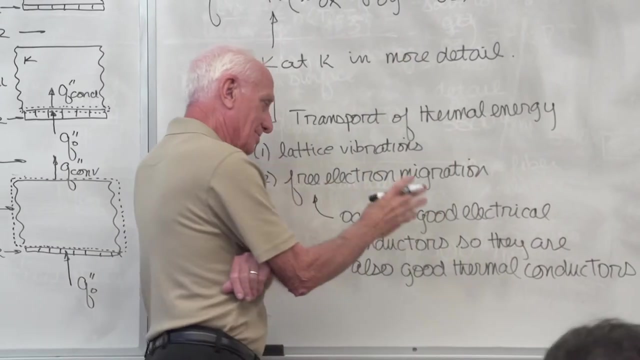 Aluminum wires, oh yeah, they're okay. They conduct electricity, but not as well as copper. But aluminum is also a good conductor of thermal energy. So as long as they're good electrical conductors, they're going to be good thermal conductors. 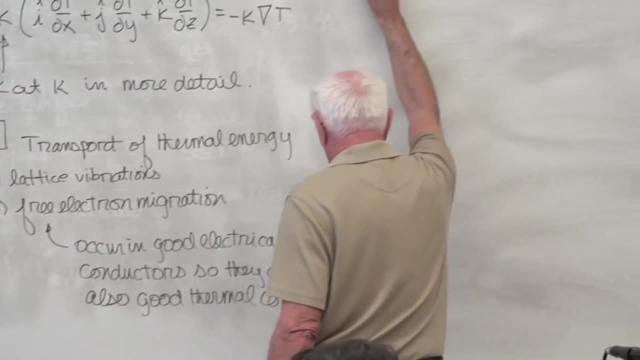 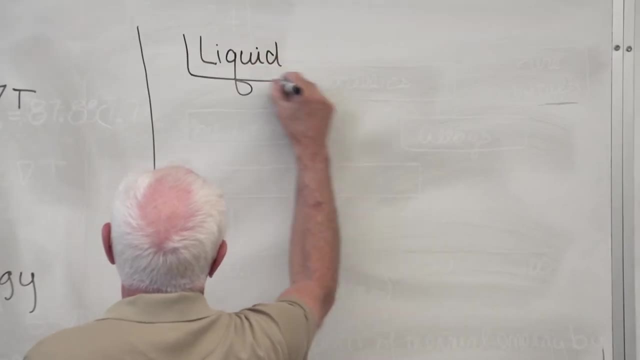 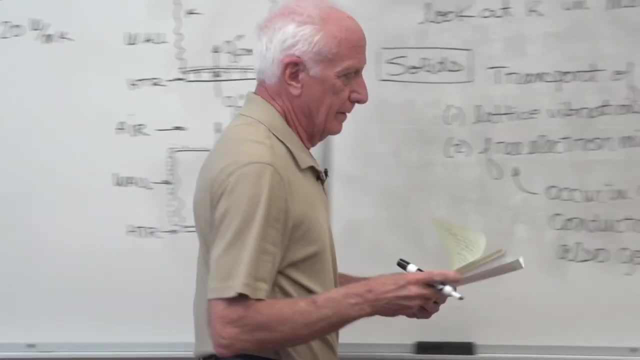 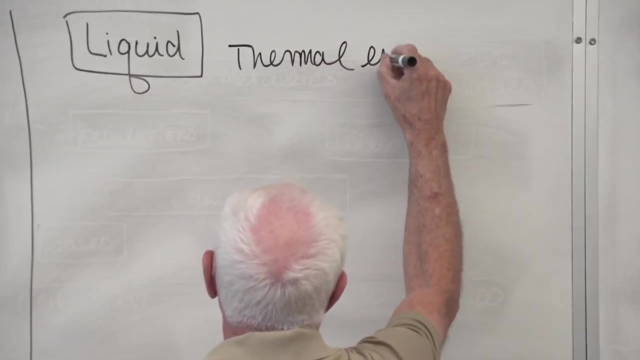 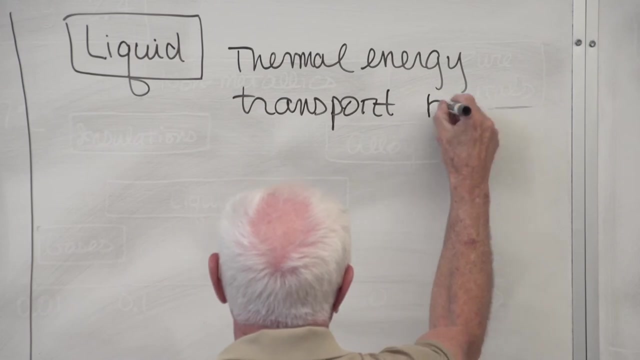 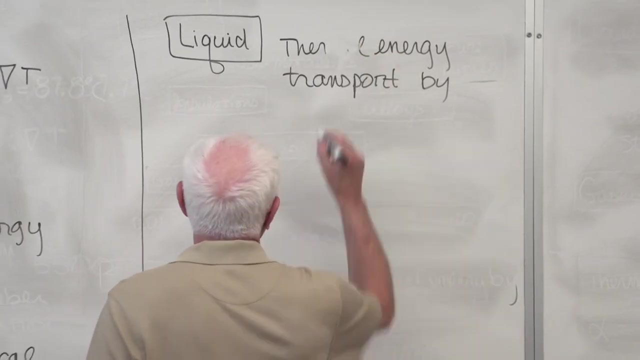 Let's take a look at what happens with a liquid. I'll take the typical one, you know: water, Water, maybe oil, So this has thermal energy transport by this one. So this is a liquid, This is a liquid, This is a liquid. 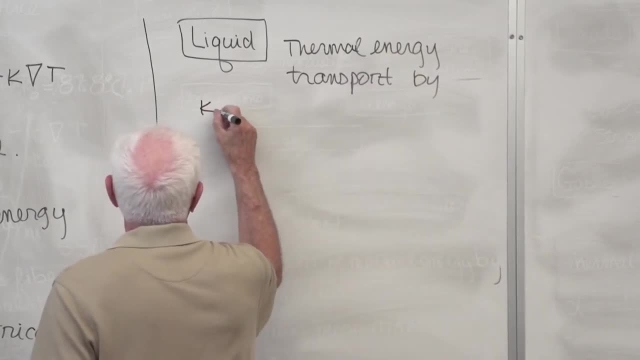 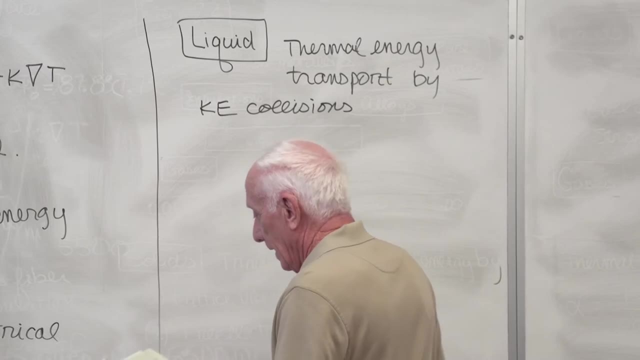 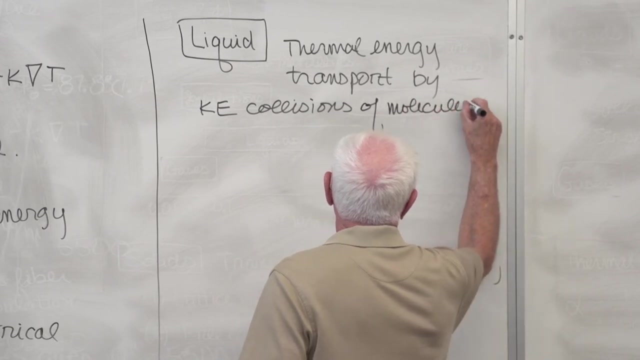 So this will passing over. This is a liquid. We're not just talking about hot 쿠川. Are there any other ones? There are. There's actually oneziehes hot coulis. That's hot couldis. It is in the glu. pur short solution. 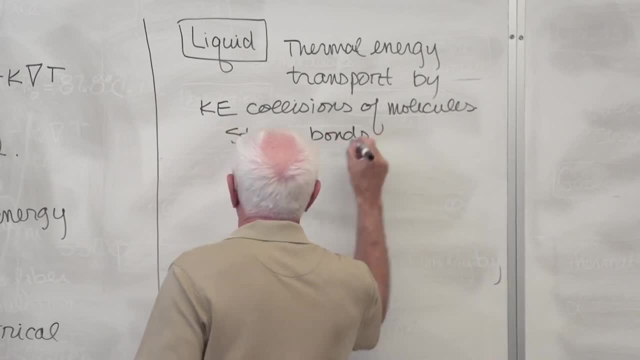 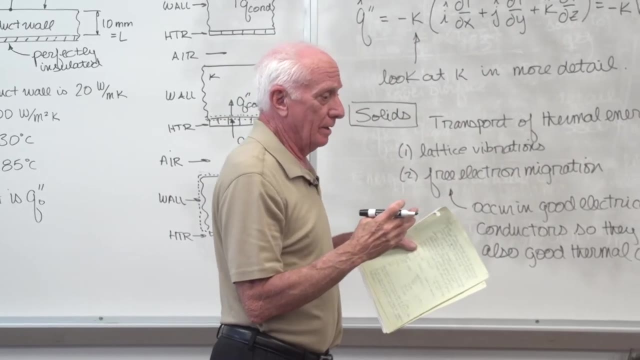 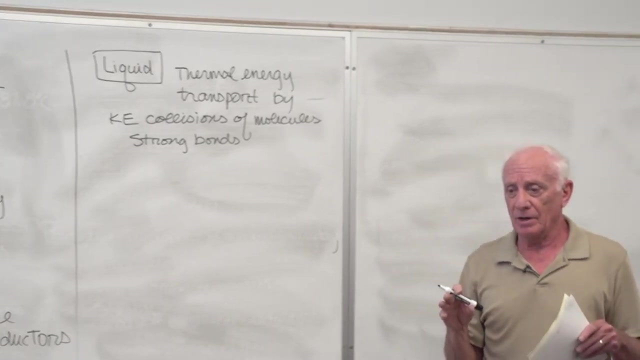 I studiedありますati and I've seen an��aites and it's a liquid treatment windows. That doesn't mean it builds up. You heat water and when it's heated these molecules start to move with kinetic energy. They impact or have. 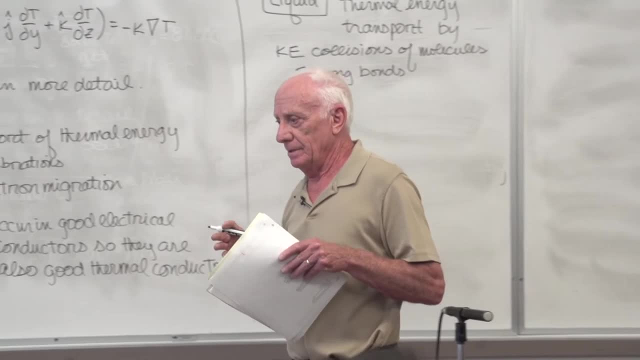 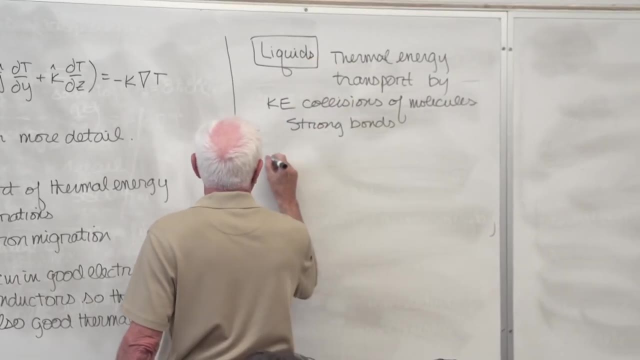 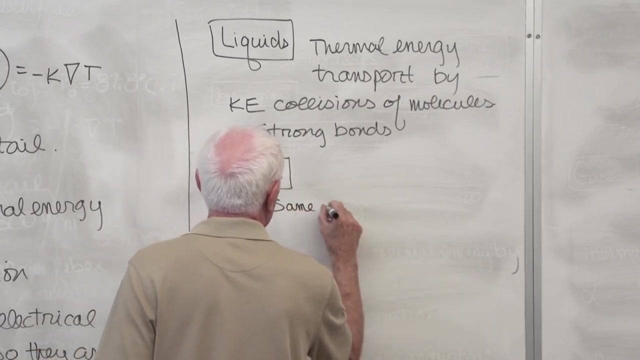 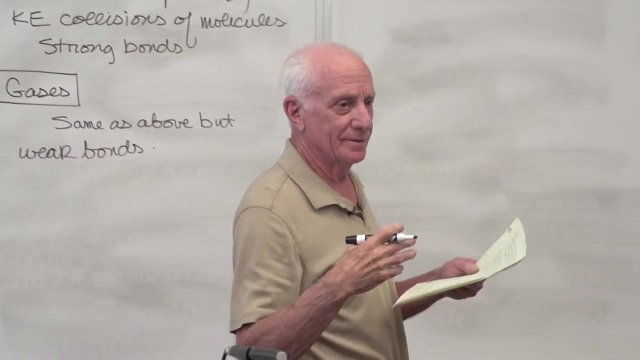 a collision with a neighbor and transfer that energy and it continues that way. Gases same as above, But they have weak bonds. They're spaced further apart in a gas So there's less chances of collisions occurring. So you don't get the transport of. 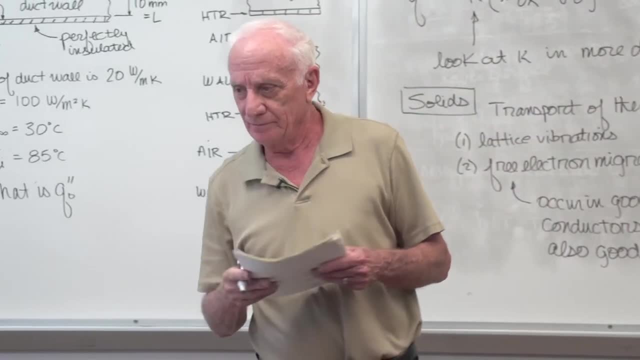 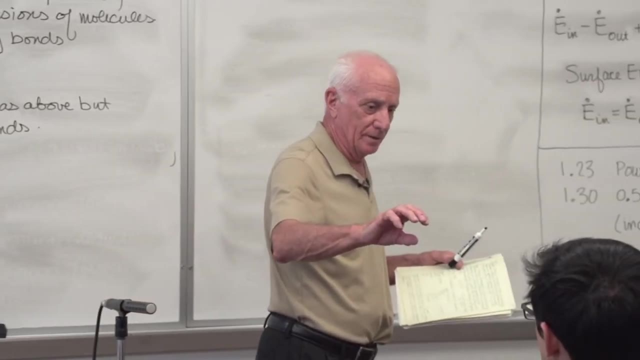 thermal energy in a gas that you do in a liquid. I mean you take a glass of water and dump it on the floor, I'll see a puddle down there. Take a glass of air and dump it on the floor, and I don't. 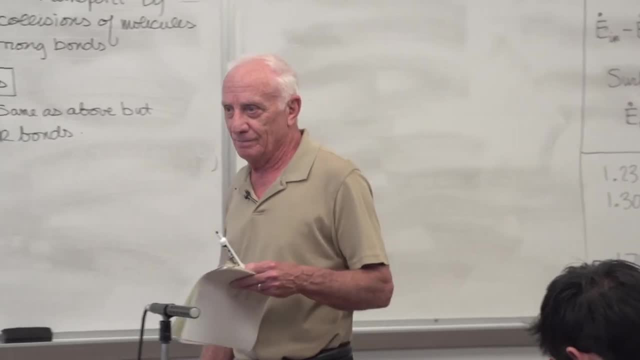 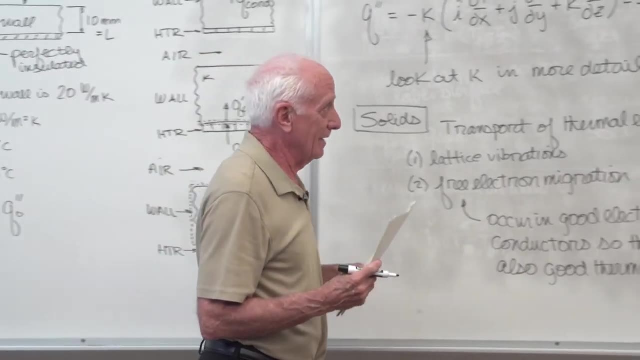 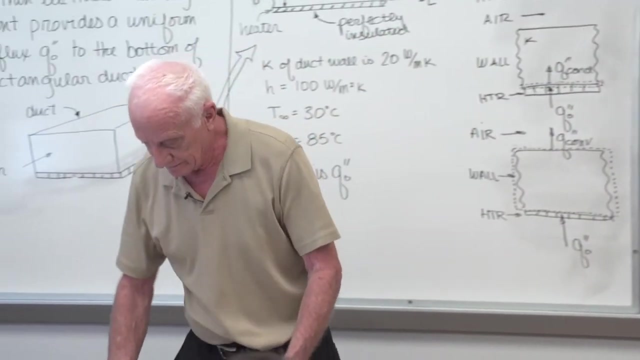 know where it went. it's gone, it disappeared Because the bonds are weak. they just spread out, They don't stay together. Okay, So that's pretty much what's happening with those three. Let's take a look at so you get an idea of how. 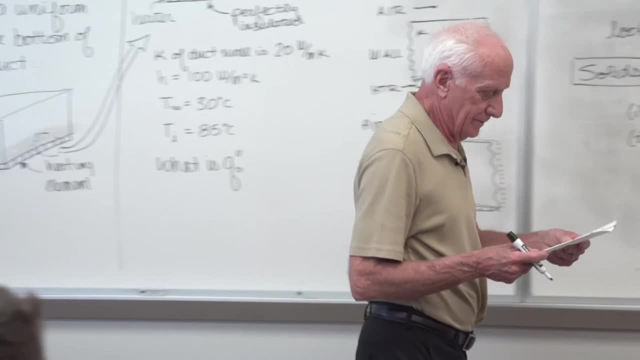 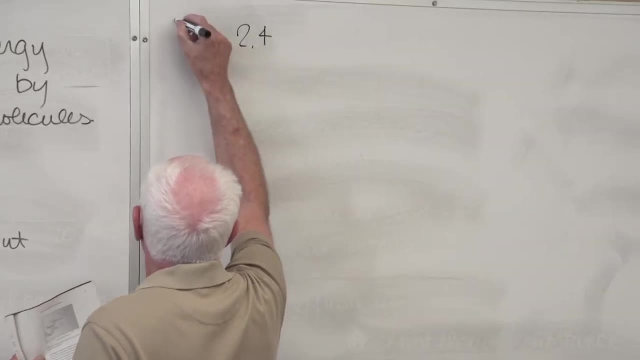 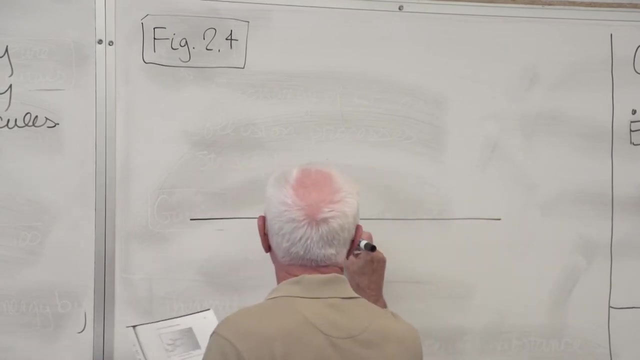 these guys look when I put them on a little graph here. This is in the textbook, figure 2-4.. So I have a x-axis here which is k: 0.01, 0.11,, 10, 100.. So typically, gases occur in this range somewhere around 0.02 to maybe 0.3.. Let's just take typical liquids. They occur from about 0.2 to about 8.. Alloys occur from about 10 or 11 out to maybe 150.. 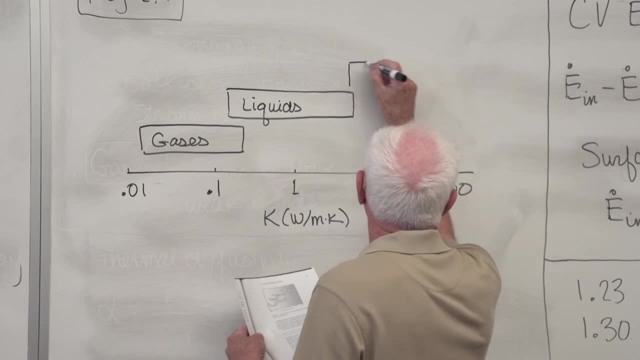 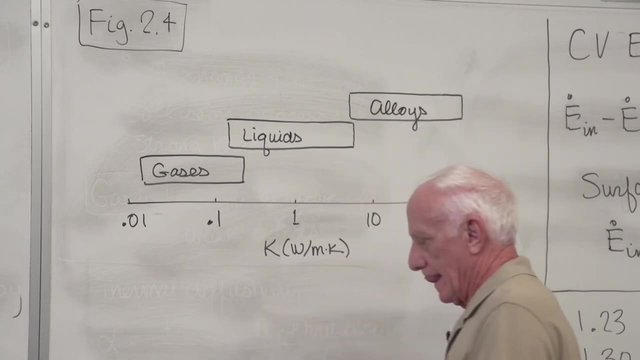 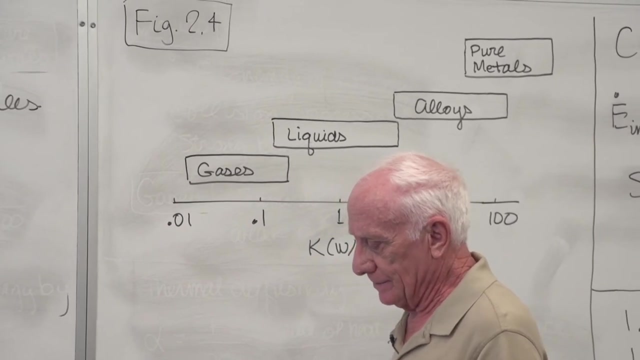 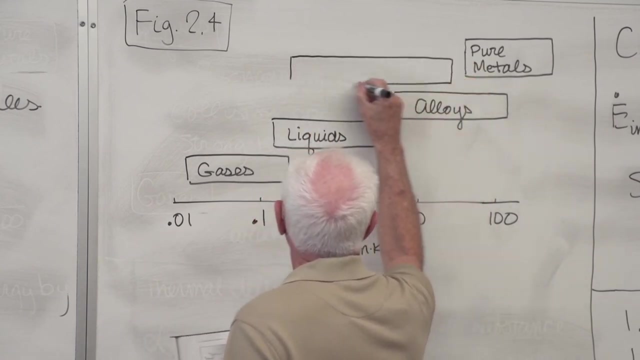 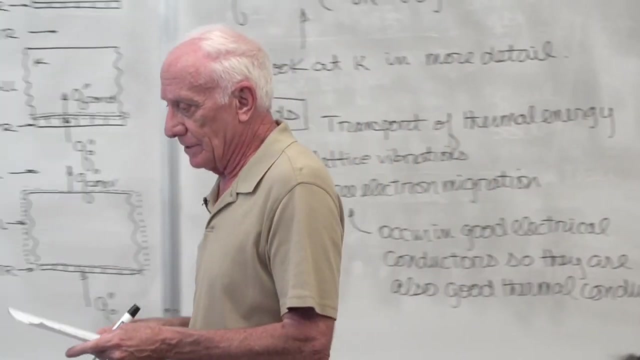 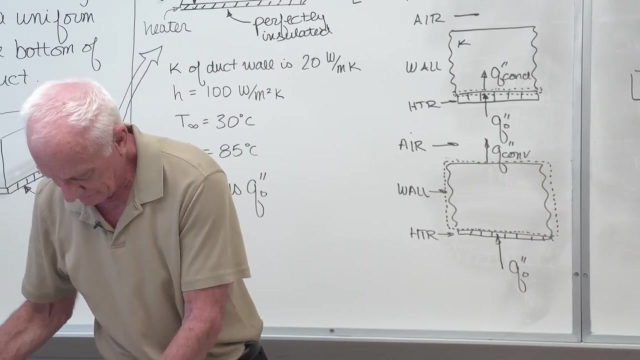 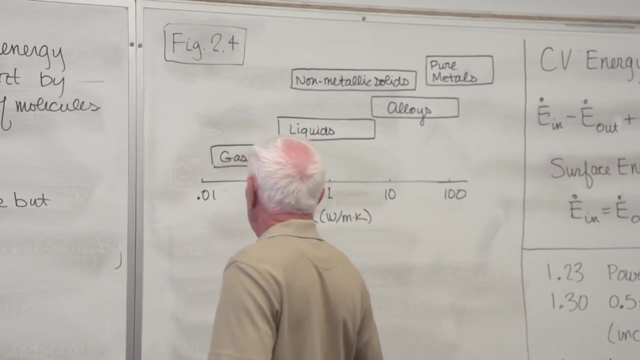 So alloys and pure metals from maybe around 50 on up to 500.. Non-metallic solids From about 0.3 to about 50.. This gives you a rough guide on the thermal conductivity of these various substances. If I want, I'll just 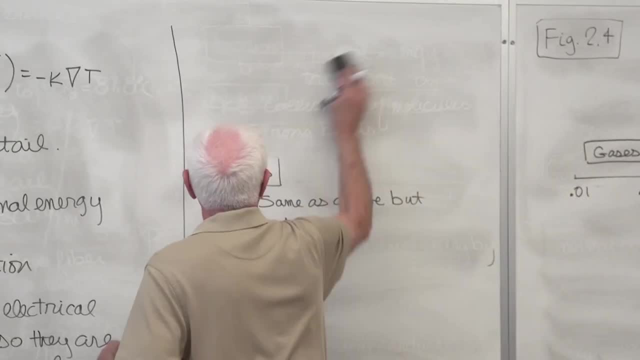 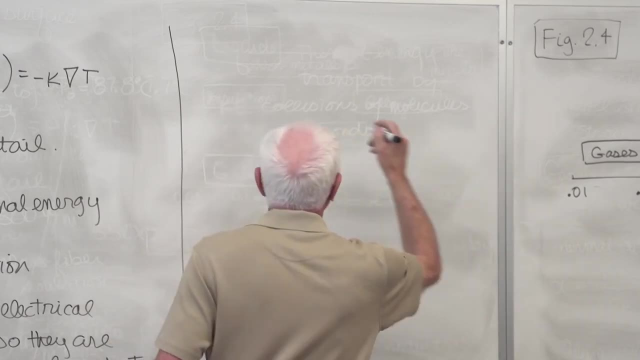 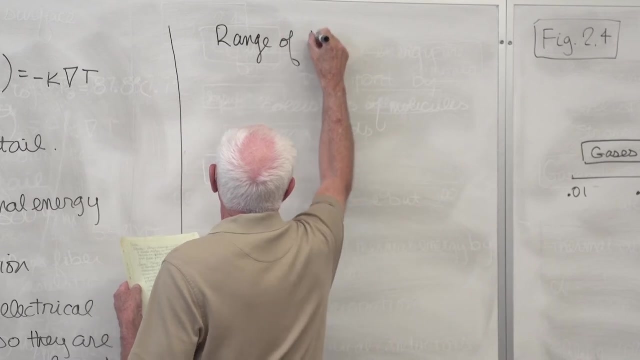 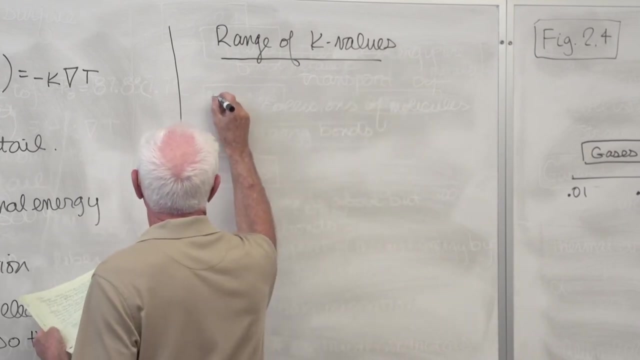 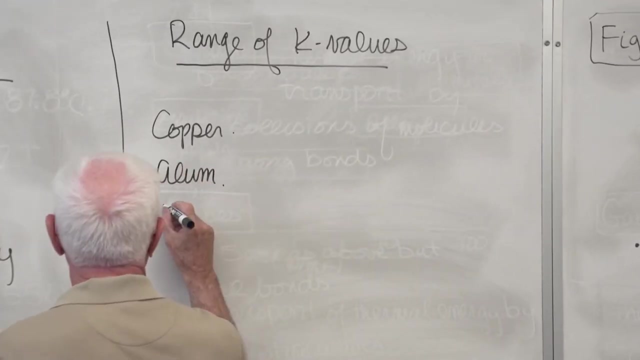 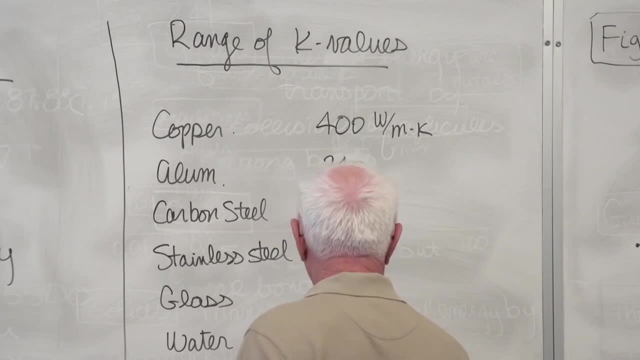 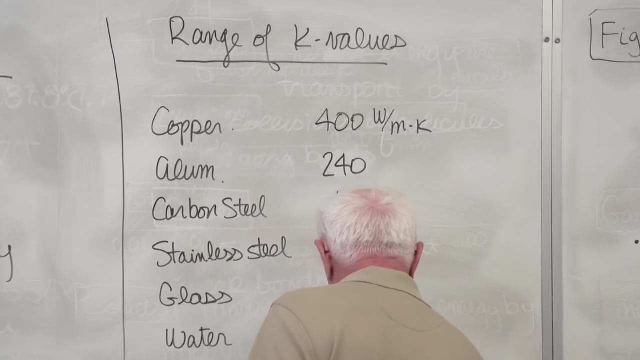 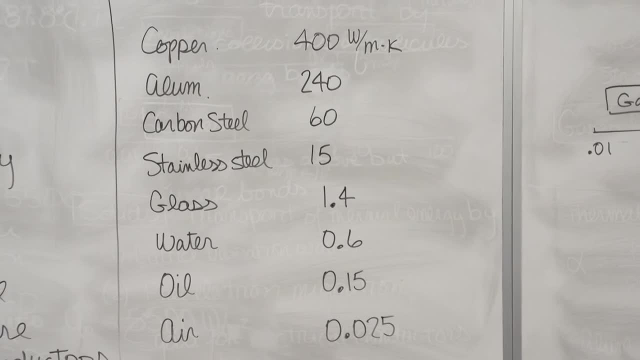 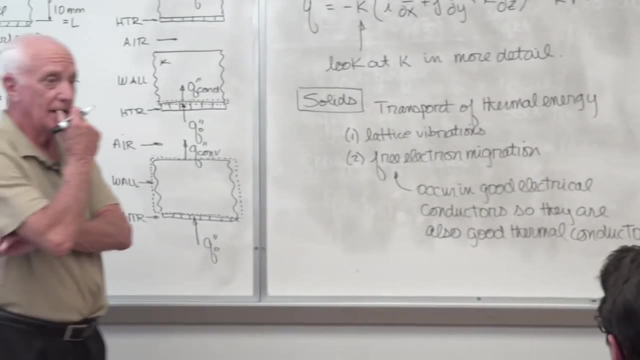 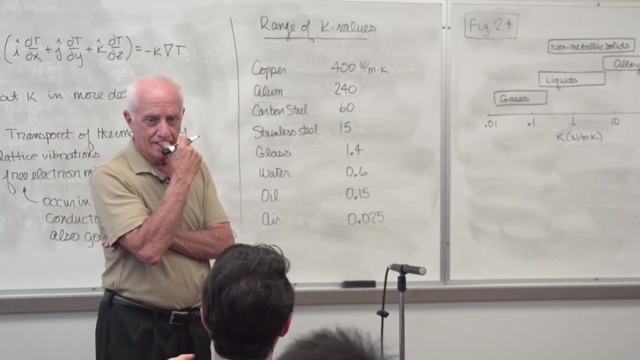 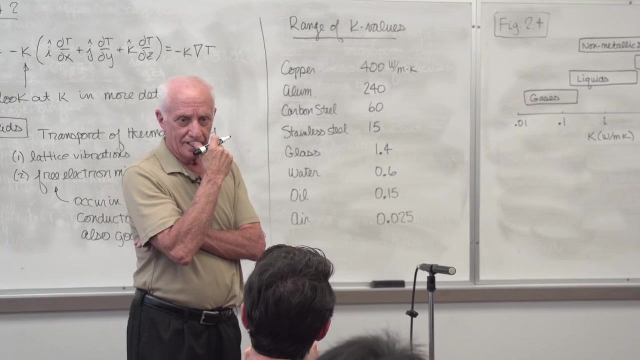 So there's a range of values of those. So it seems like materials get to be more conductive or less conductive as they become more energetic. But do plasmas then become more thermally conductive or no? Like what? Give me an example. What? 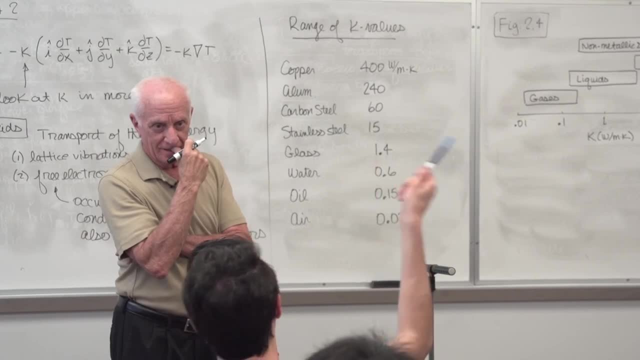 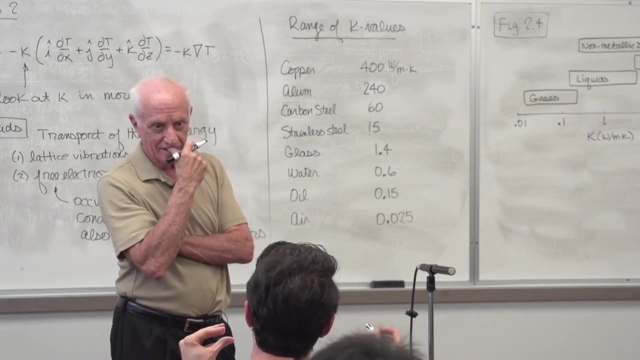 So like if you had like in, incandescent or not incandescent these lights, Yeah, yeah, yeah. Is that plasma, then, more thermally conductive than just the gas? How does it light up? By yes? the answer's yes, because it's interacting. 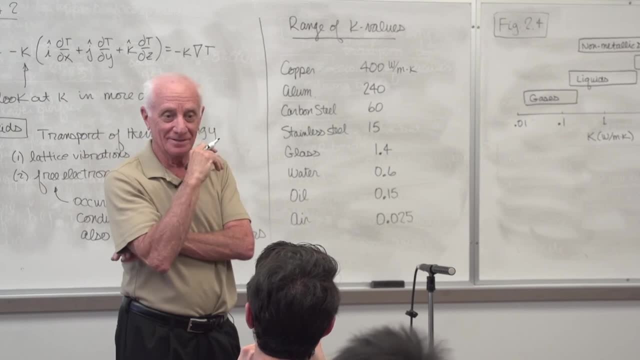 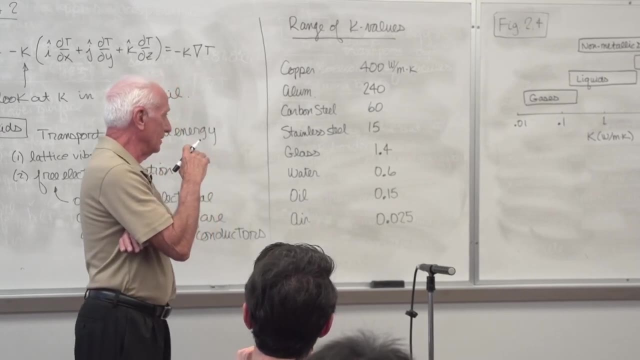 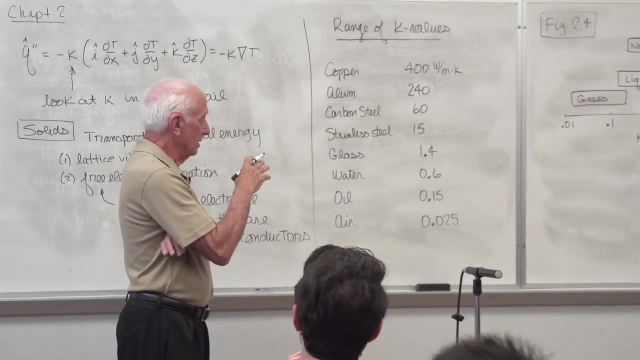 It typically starts from one and goes to the other. Yeah, it's again the collisions and things. Now, just so you understand, we can only have conduction if the liquids and gases aren't moving. This is not water in motion. 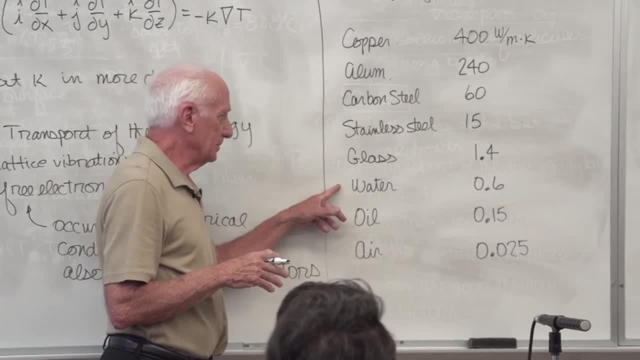 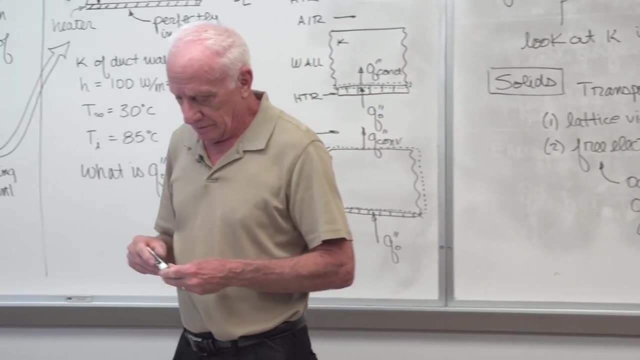 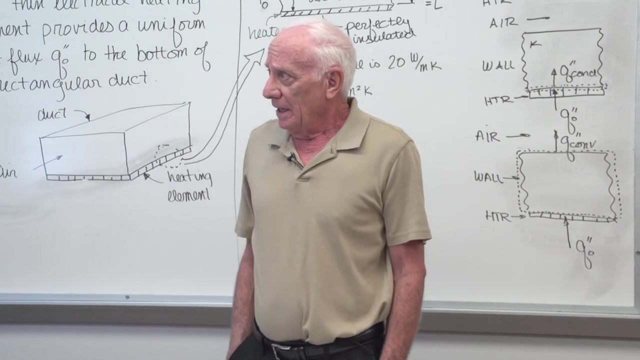 this is perfectly still called quiescent. Perfectly still water, perfectly still air cannot move, Like you say. I've got a 1960s home and the windows are single pane glass. I'm trying to be more energy efficient, so I'm going to go out and spend some money. 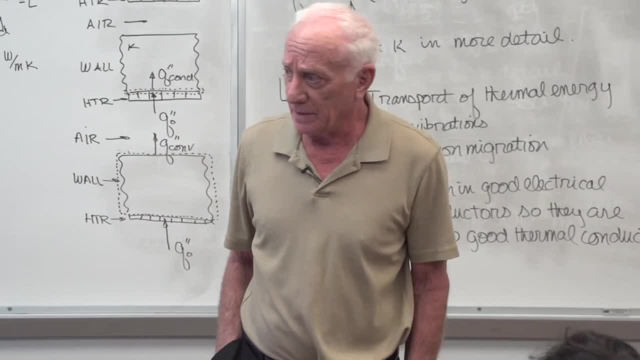 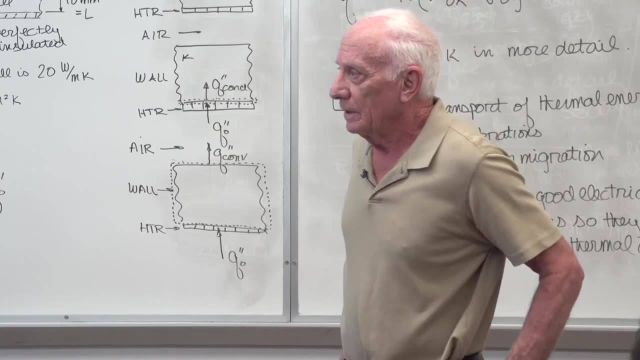 and get dual pane windows for my house to cut down on my energy loss in the wintertime. I go out and I look at them and I look at how they're made, and they're made with two glass panes. Well, that's good news so far. 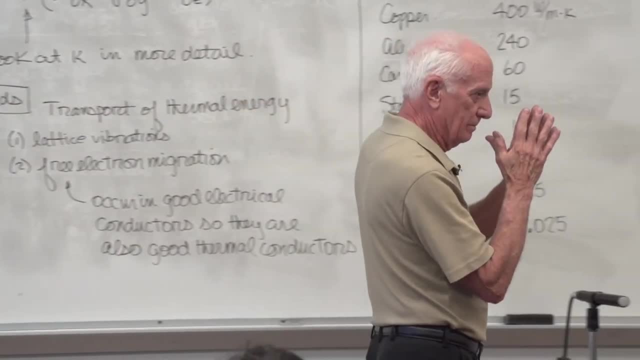 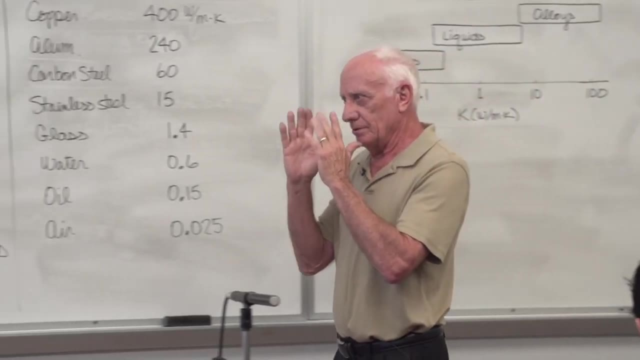 Two glass panes are better than one glass pane. They're heavier, they cost more. but that's the trade-off: Two glass panes. But you know what I'm going to do: I'm going to put those two glass panes really close together. 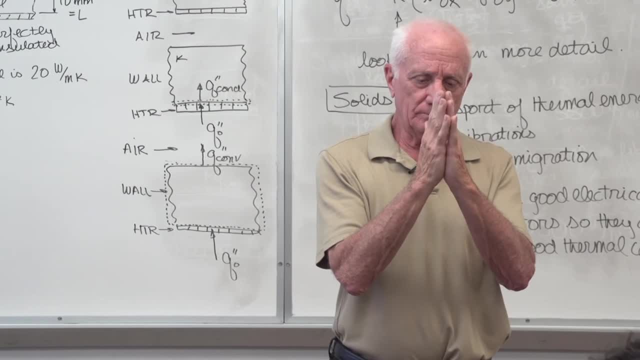 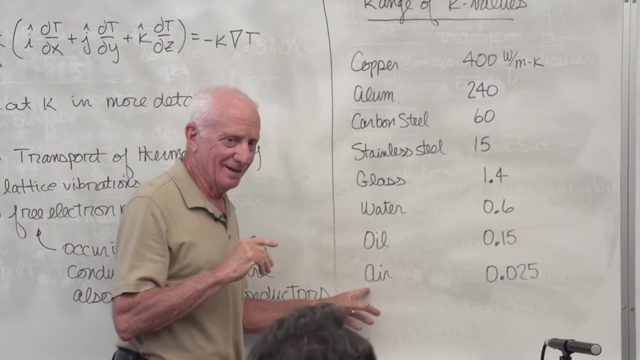 There's air between those two glass panes. Now if that air moves in there, I'm in trouble because it's no longer conduction, it's convection. So I don't want convection. So I want to get those two glass panes. 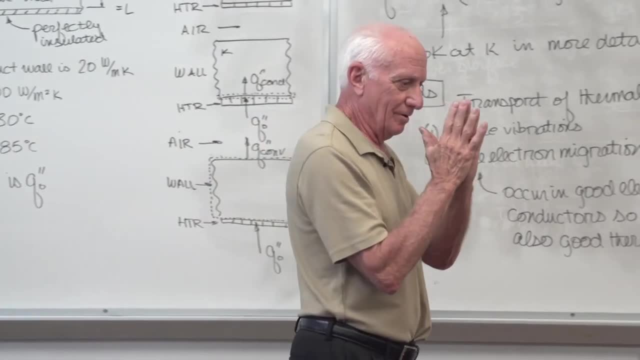 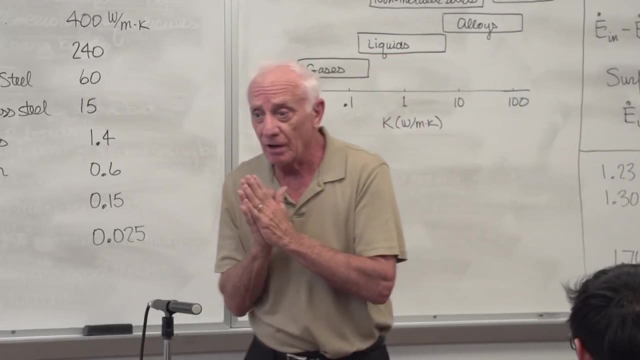 so close together, the air's not going to move. You know the old story about fluid mechanics: You've got a pipe. you want to create more resistance for the flow. you make the pipe diameter smaller. More resistance, less flow goes through. 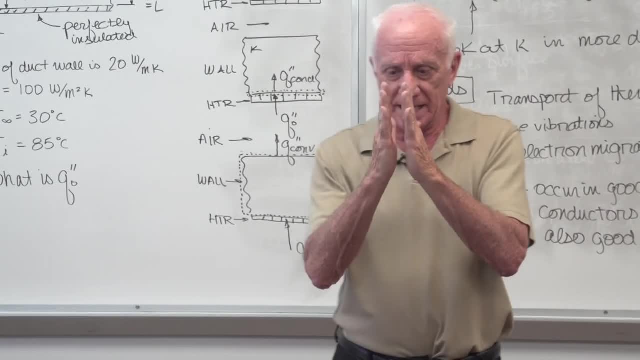 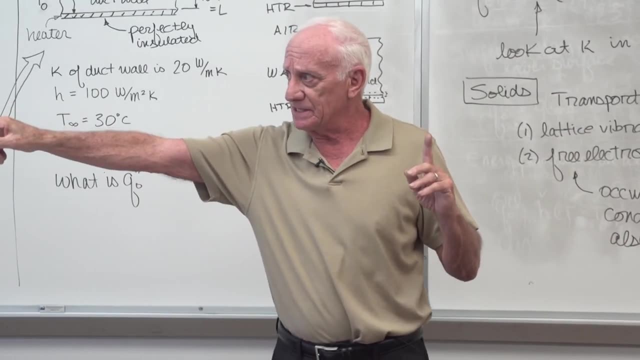 Same thing for the glass. You get those two glass panes together. there's a lot of resistance to flow. Air doesn't move easily In this room right now. that wall's warmer: it's outside, facing the sun. That wall's cooler: it's facing the hall. 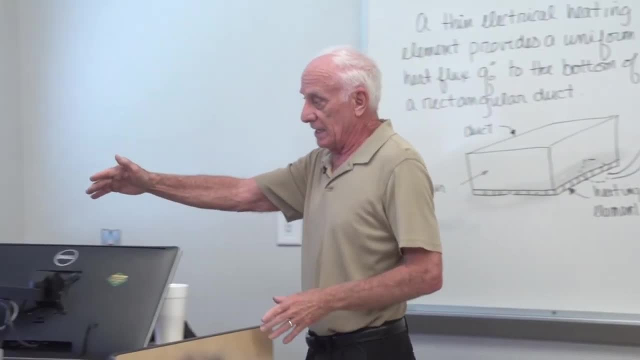 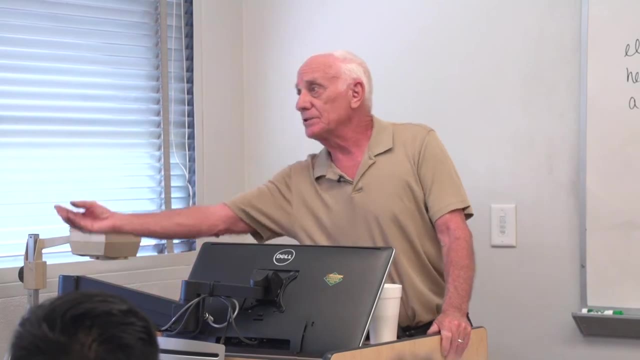 The air over here. the temperature of the air close to the wall is higher. Its density goes down. Its density goes down, its buoyancy goes up. The warm air rises on the window side of the room, goes across the ceiling to the hall side wall. 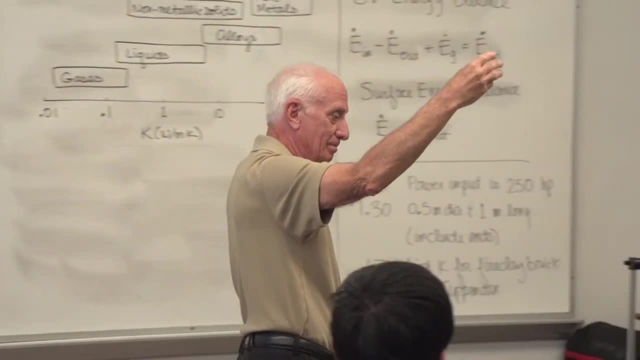 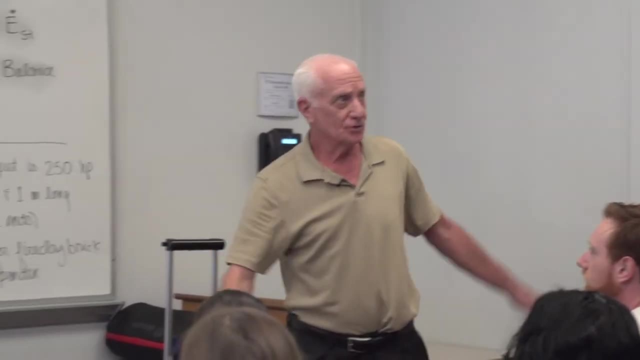 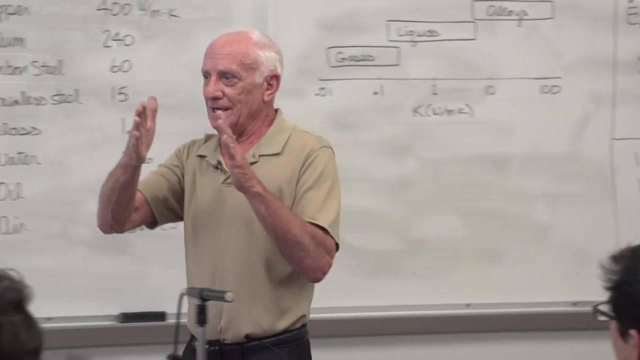 which is cooler. its density then goes up, buoyancy goes down, the heavy air falls down to the floor and makes a circuit, assuming the HVAC is turned off. So we have a circuit of air in here. Now, the closer we bring these walls together, 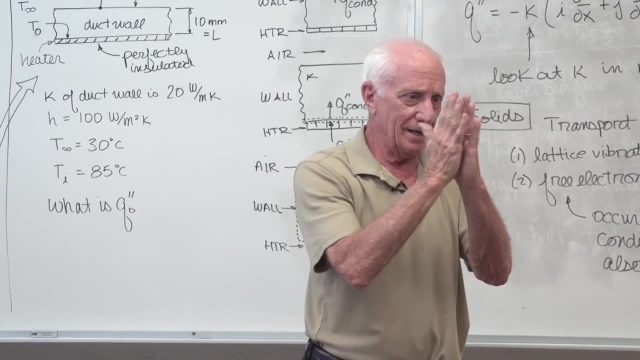 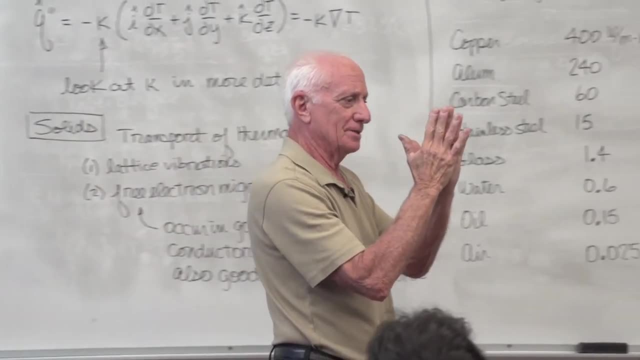 the less air is going to move. until, if we get them close together, the air is almost perfectly still. You can't get too close together. Your apartments near a freeway complex and you have big trucks and so on. vibration and the glass might hit each other like that. 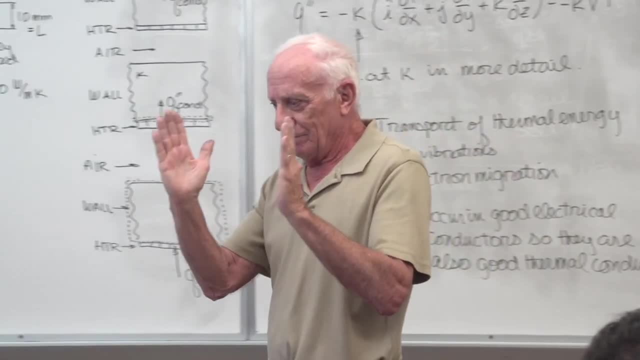 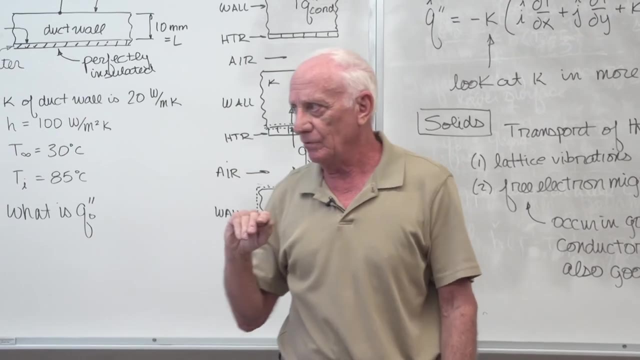 or the earthquake comes in California, and you don't want that. But you want to get close enough together where the air is not moving much at all. if at all, That's your double pane window glass there. So, yeah, the whole point is. 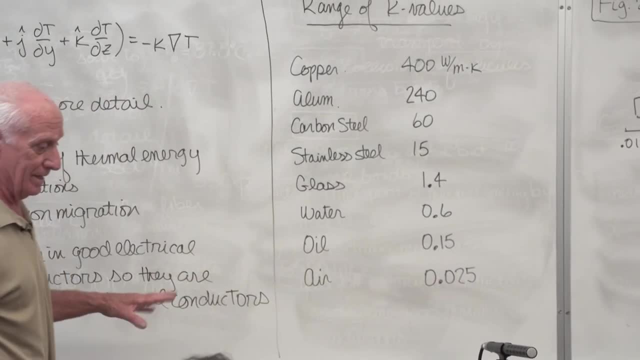 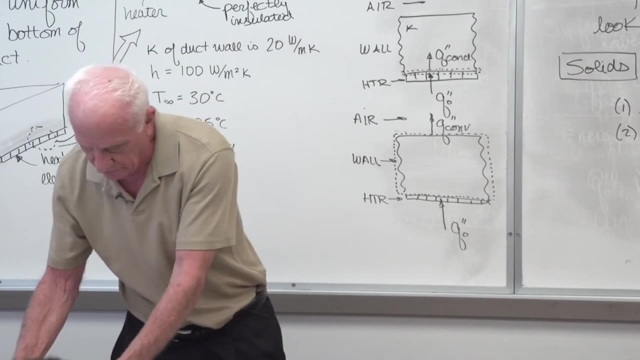 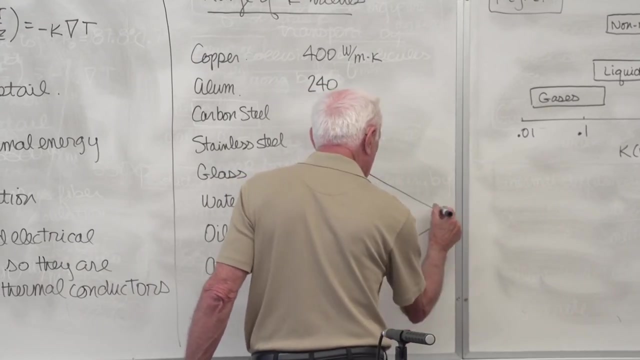 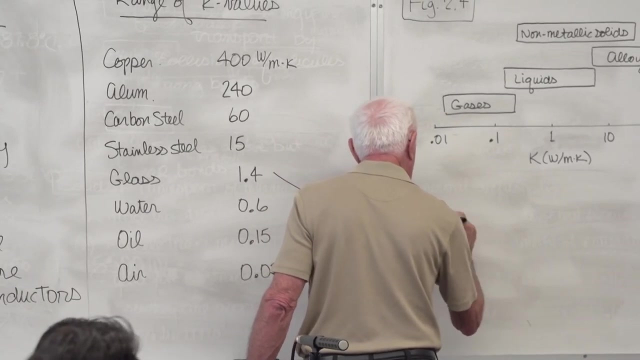 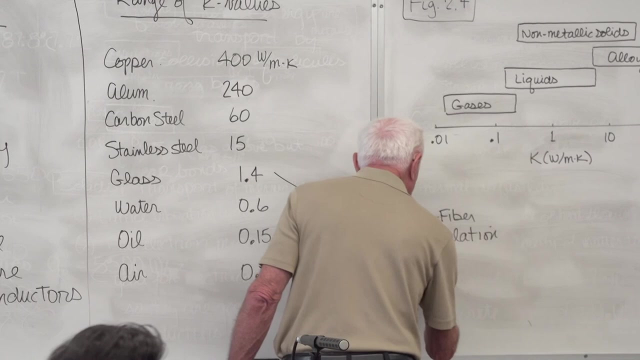 if you can keep water and air from moving, it could be great insulation. As a matter of fact, if you want, you can go ahead and combine glass and air and get what we call glass fiber insulation. K is In the range of 0.040.. 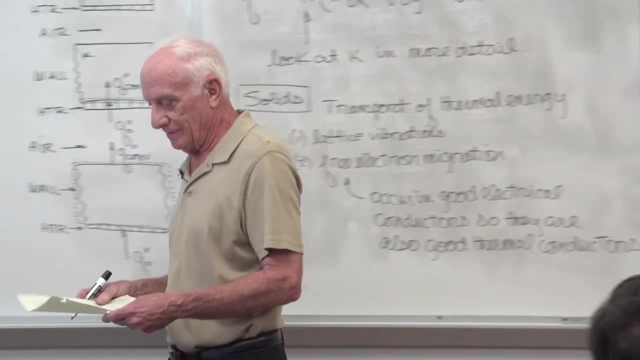 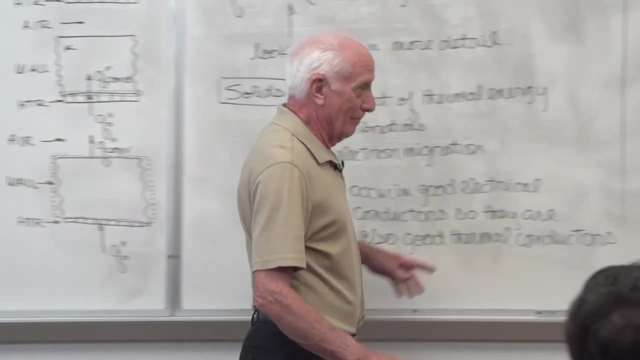 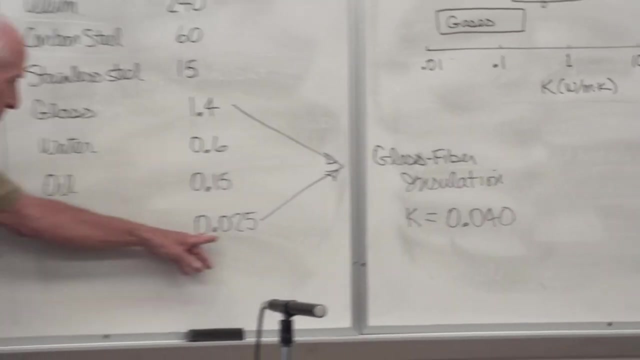 Wow, we just invented something fantastic. If you can get air not moving by, combine it with glass. what does that mean? Glass fibers, Glass fibers. that's why it's called glass fiber. insulation. 0.025 combined with 1.4,. 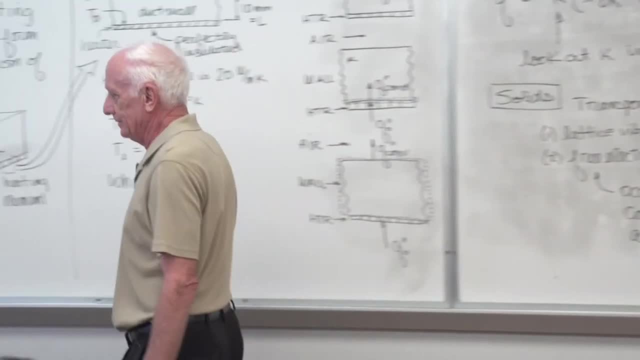 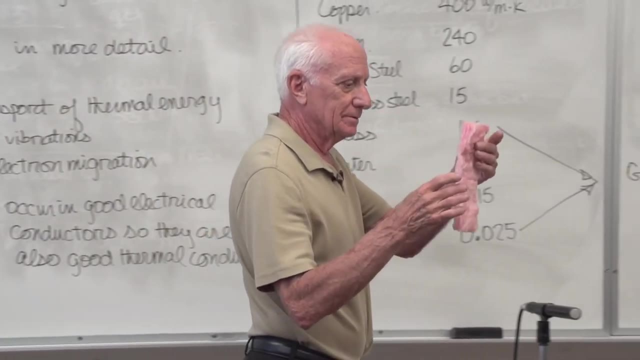 what do you get? 0.040.. Wow, congratulations, You just got something great. Yeah, there it is Fiberglass insulation, I don't know. put in your attic whatever, Put it around pipes. Yeah, what is it? 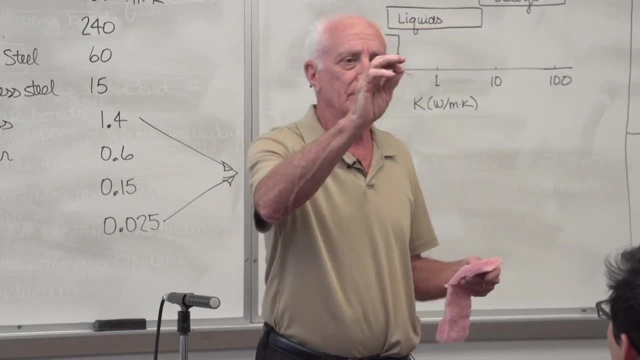 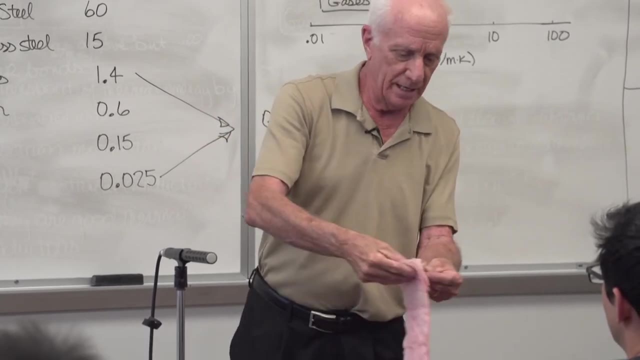 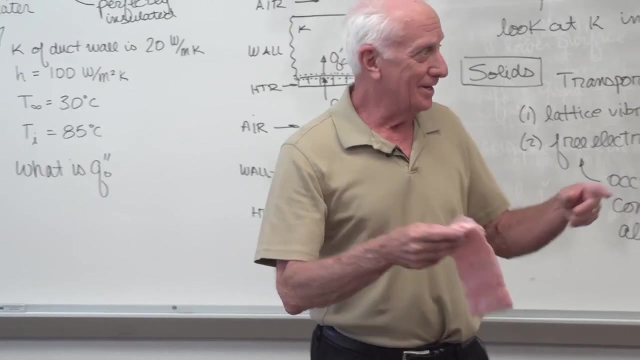 It's a bunch of little glass fibers, little tiny glass fibers, and they're arranged in layers, Layer after layer after layer after layer. There's a layer, They're layered. Yeah, don't get it wet. You get it wet, you're in deep trouble. 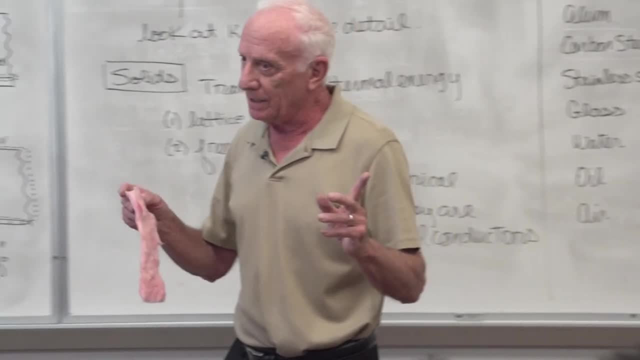 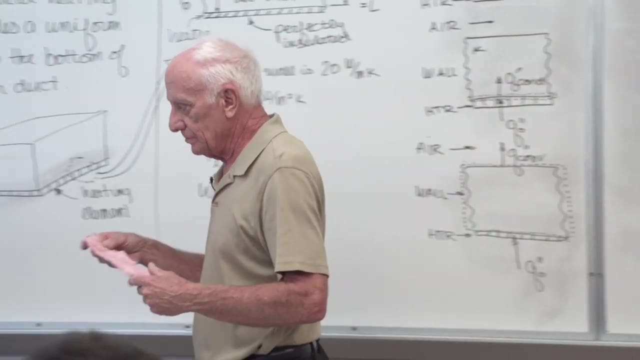 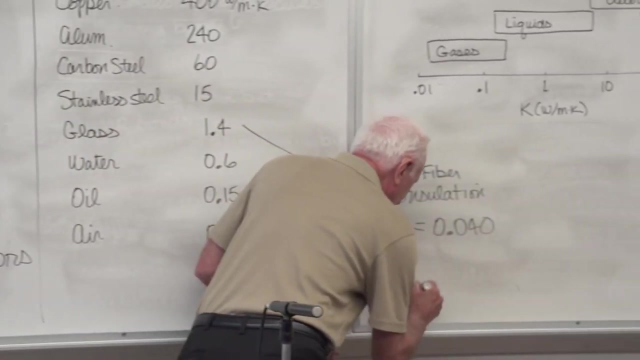 Deep trouble. Don't get it wet, Don't step on it. If you compress it, you've lost all the insulation because you force the air out of these little gaps. So the point is that you've got a bunch of spaghetti fibers like this: 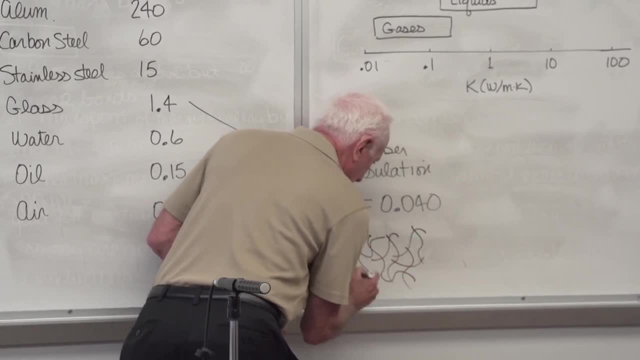 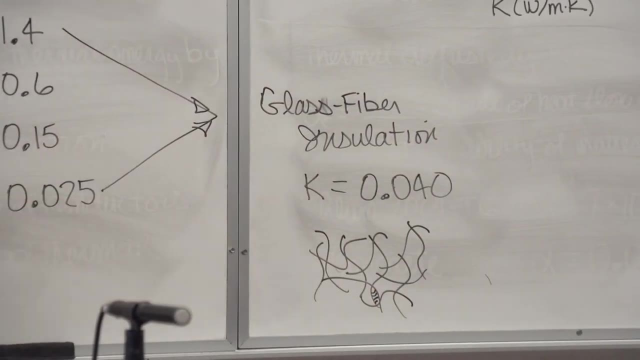 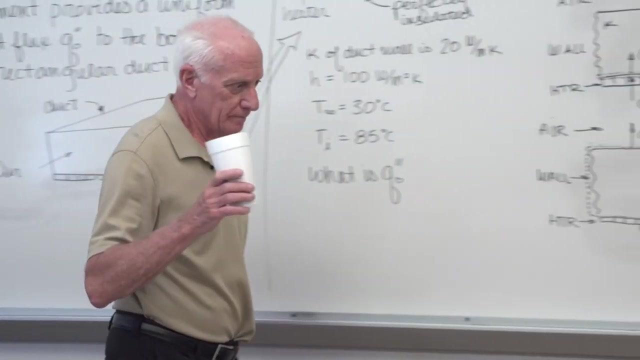 and then you've got like this: The whole point is, you want to trap air in these little spaces like this. You want to trap air in spaces like that because if you can do that, you've got a great insulator- Lightweight, It's not that expensive. 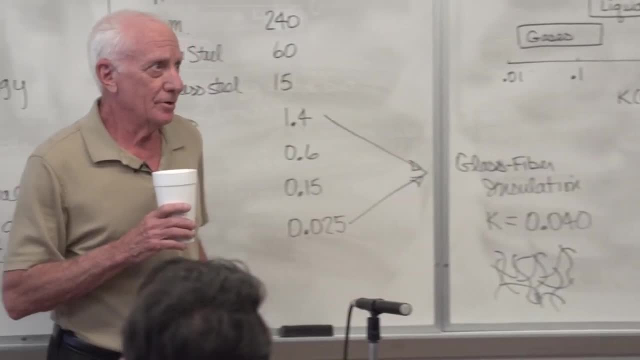 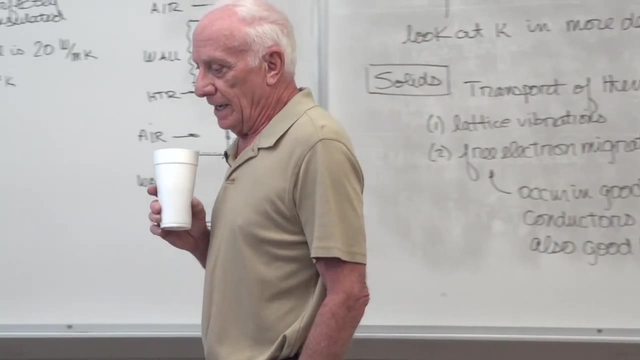 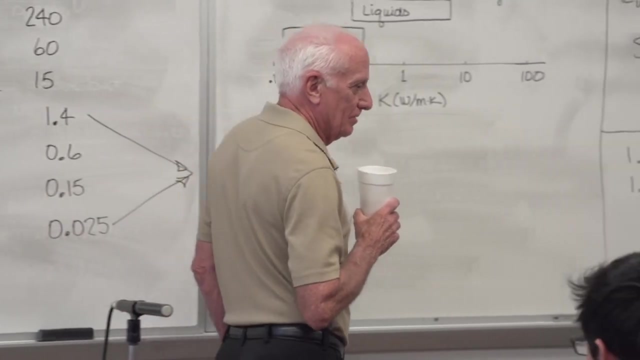 Great stuff. Let's say you're going to mammoth skiing in February and you say I better go get a good sleeping bag because I'm going to be in this cabin which isn't heated very well. So you go to the sporting goods store and you say 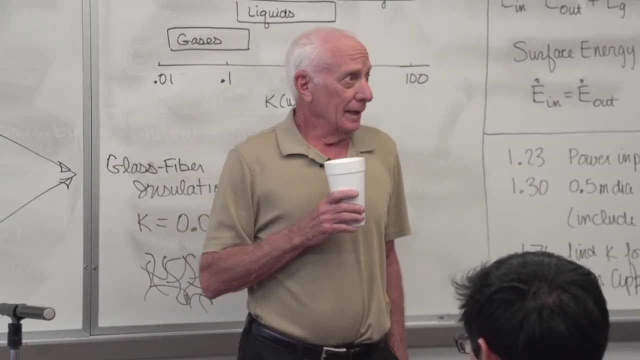 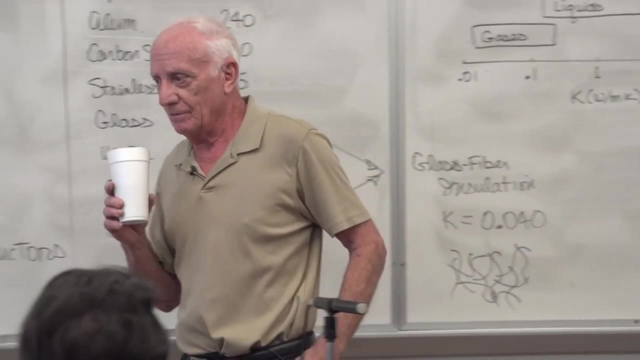 I'm going to mammoth skiing in February. I need a good sleeping bag. The guy says, well, they're on the wall over there. The cheaper ones are there and expensive ones are over there. I said, well, okay, Well, can you explain to me what the difference is? 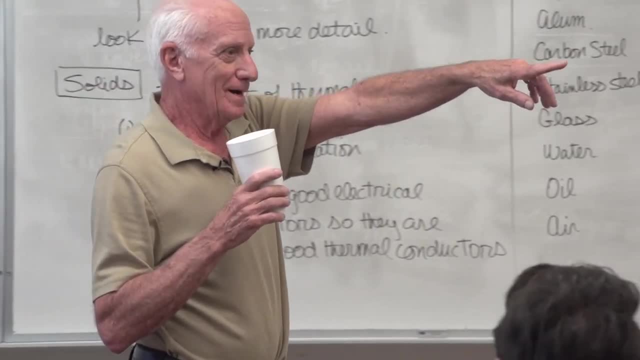 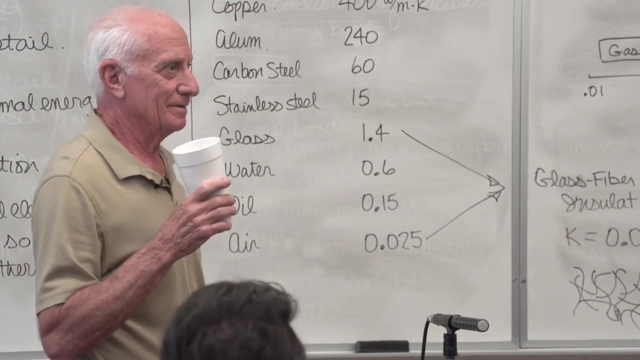 Well, that one's good to minus 10, that one's good to minus 20, that one to, let's just say, 20 degrees, that one's good to 35 degrees Fahrenheit. He said, okay, well, but what's inside of them? 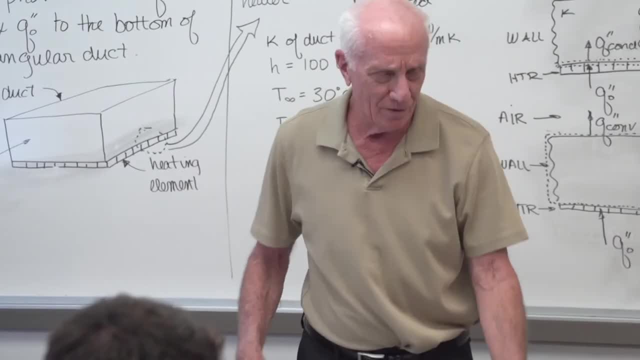 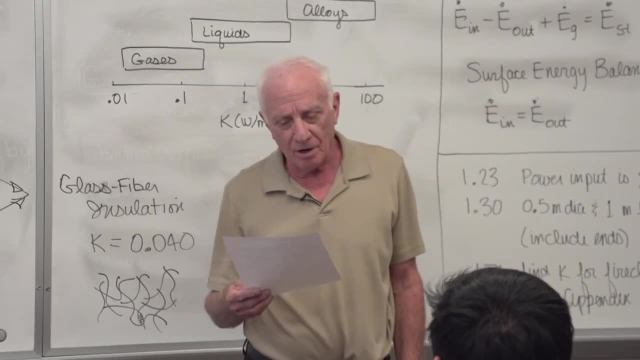 He says, well, if he, if he knows stuff, he says, well, these guys over here in the middle, these are trade names. It could be Polar Guard, Qualafil, Holofil. These are all fillings on sleeping bags. 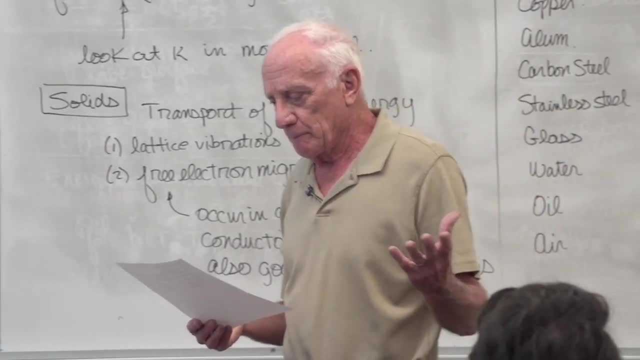 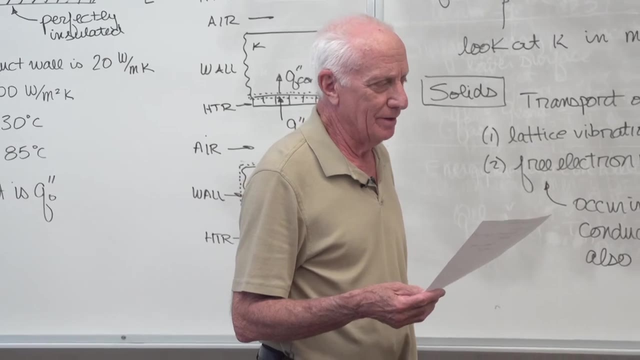 Polar Guard, Qualafil, Holofil and others. They're called holofilament polyester fibers. They're siliconized to repel water. You don't want water in there. Water destroys all insulations. No bad news: They're either in. 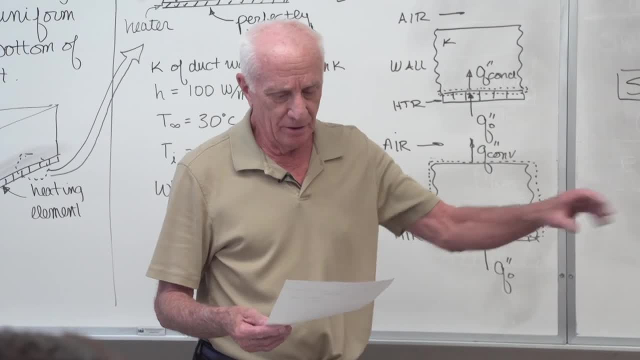 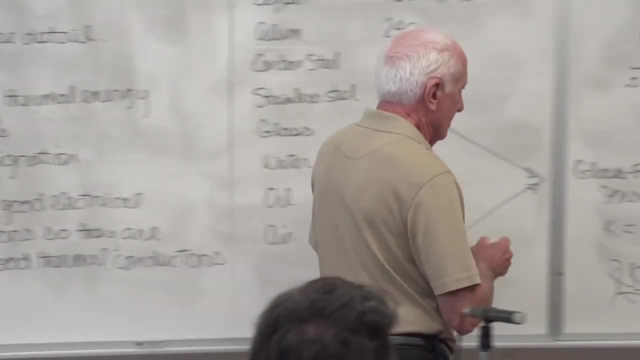 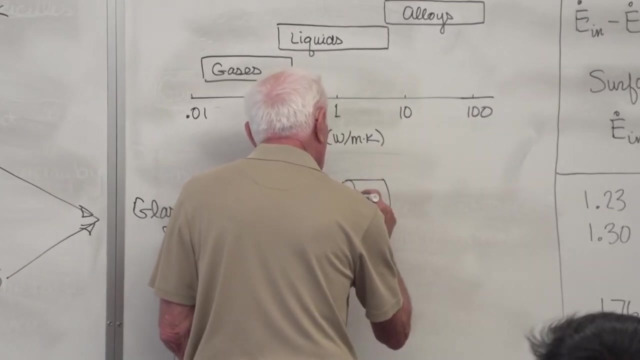 sheets, or sometimes they're loose-filled in sleeping bags, in sheets, or loose-fill. So yeah, and some of these things look like this. That's why they're called holofil. They're little fiberglass pellets like this and they're hollow, but they have. 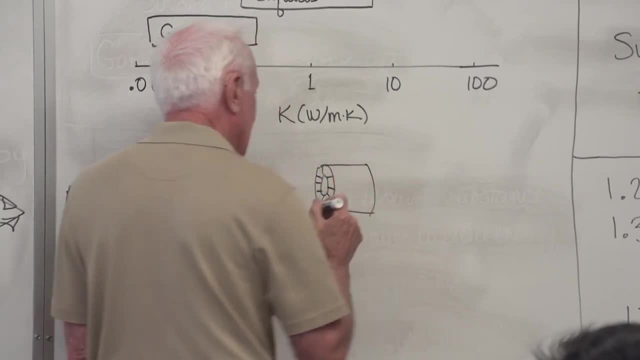 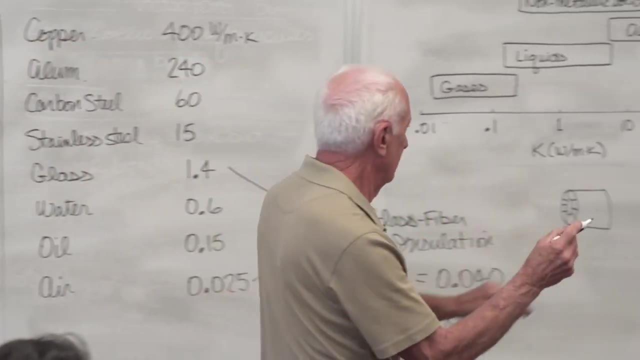 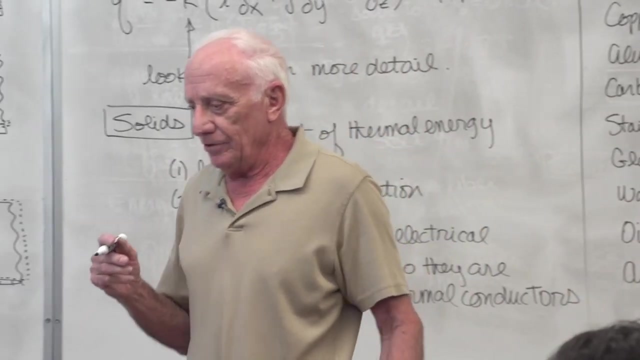 these little radial pieces like that. They're about the size of that black pinpoint there. That's how big they are, that pinpoint. What do they do? They trap air in those little areas right there. So if you sleep on them at night, 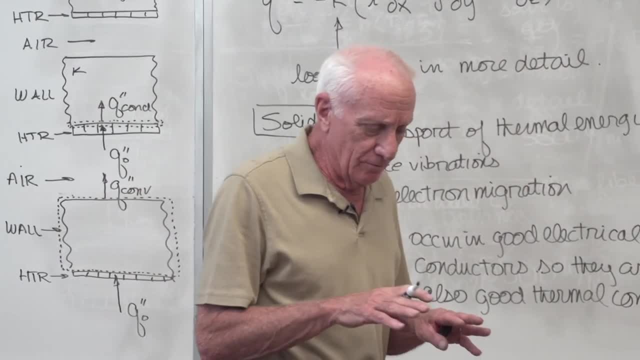 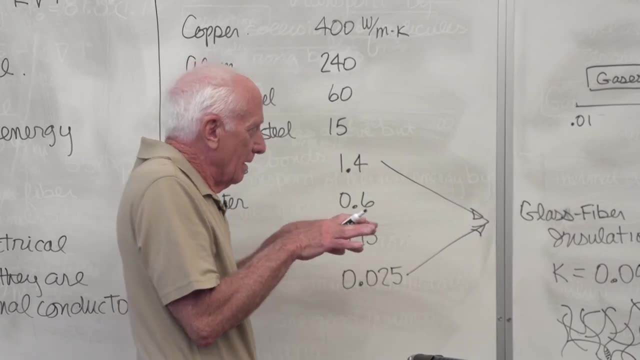 you crush them down a bit, but then the morning they pop back to their original shape. Great, that's what you want. You don't want to be squashed and stay flat. You've lost all the air in there. then They pop back up. The guy says: 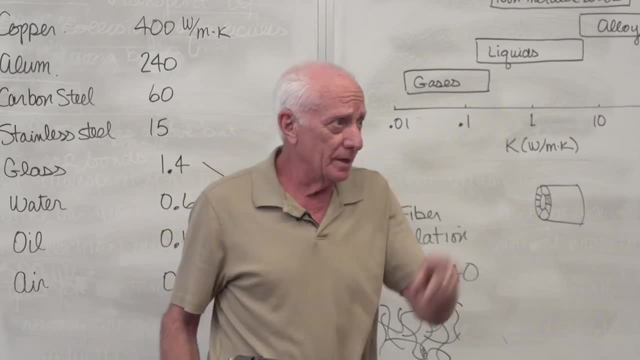 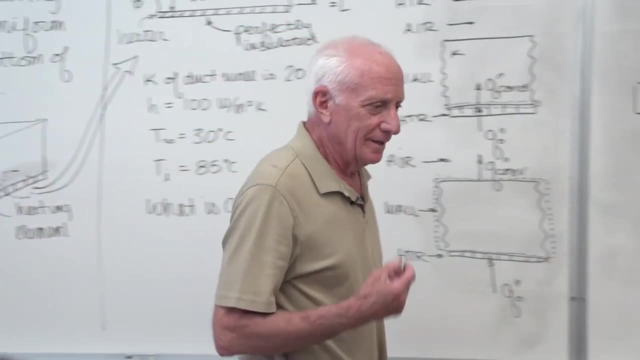 okay, that's great. How about that expensive one over there? He says, well, that's a special one. he says That's called a down jacket. The guy says: well, what's a down jacket? He says well, that one inside of there. 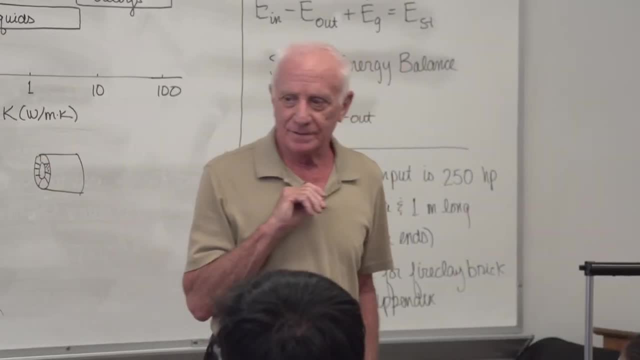 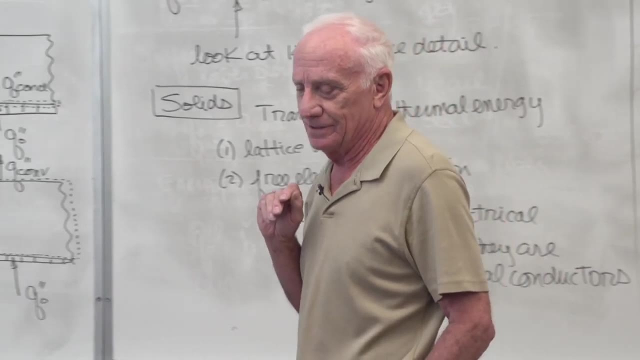 there's down feathers. He says, oh, where do they come from? He says, well, ducks and geese. The guy says: how did they get those? The guy says: don't ask me, I don't want to go about through that. 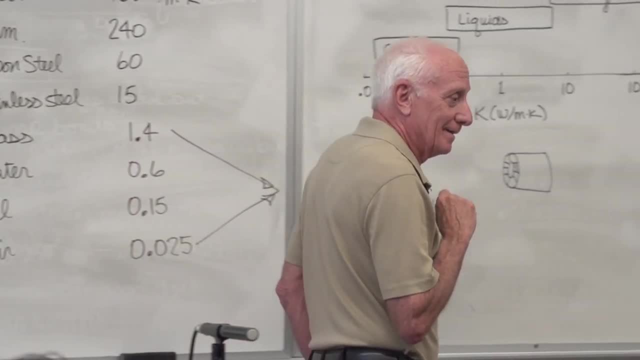 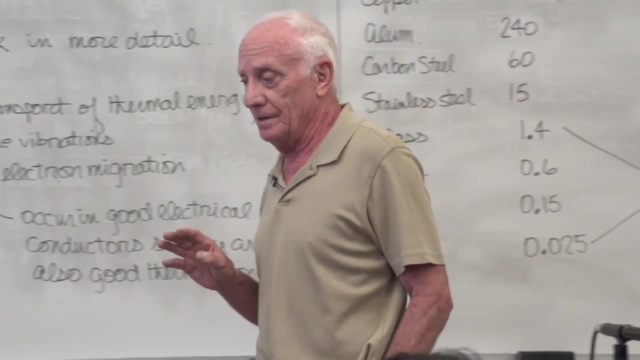 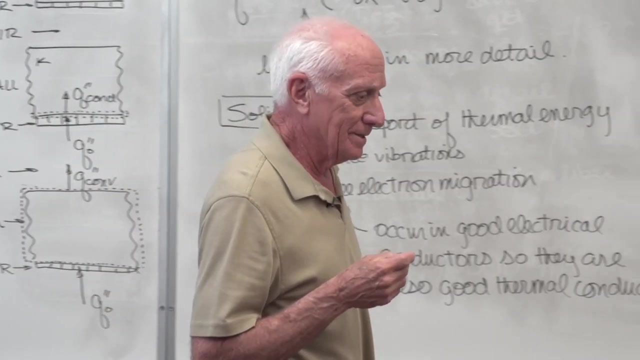 That's not a good topic to discuss. Yeah, ducks can be on a lake in spring of water. The temperature in the lake is 40 degrees and the duck is happy because the duck's insulated from that cold water. How Well, a duck has three kinds of feathers. 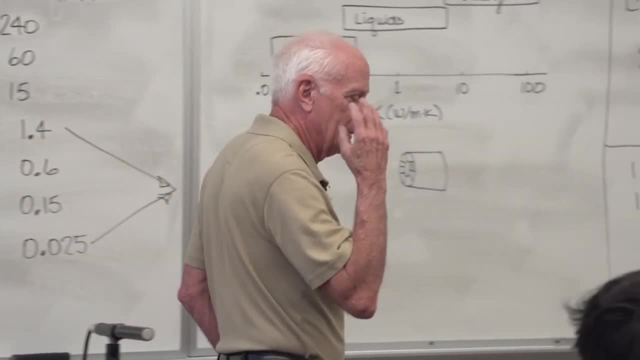 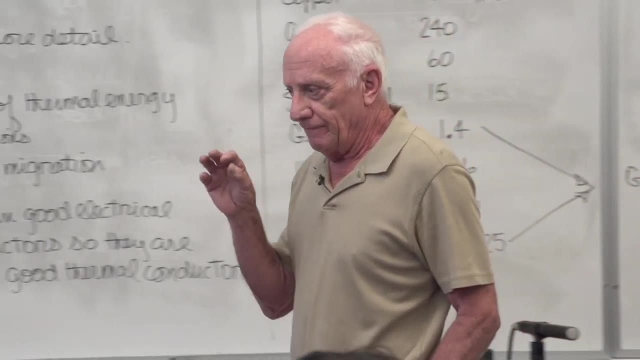 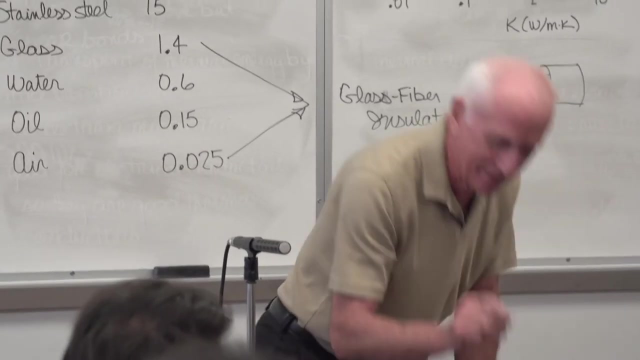 flight feathers for their wings, farm feathers for their body and their head, and down feathers close to their skin. The down feathers are very, very tiny. I threw it away now, but here it is. They're even smaller than that. My wife's got a down jacket and when she sits in. 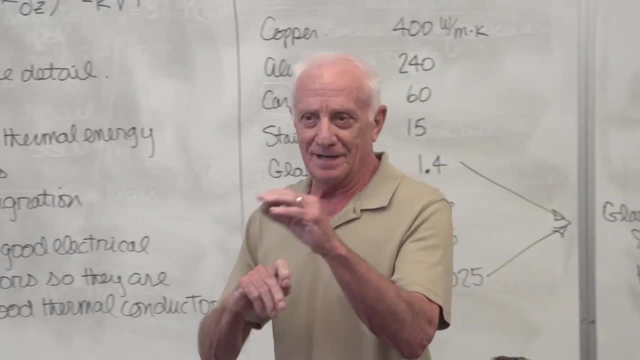 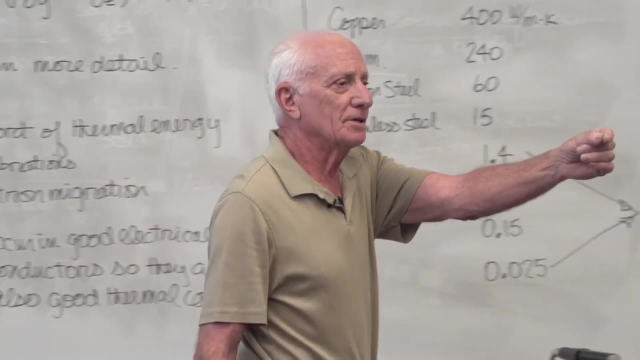 my car and I have black upholstery. she has a little cut in her down jacket. Next day I'll find little tiny down feathers on the black upholstery. They're that size. That's how big the duck's feathers are. close to their skin- that big. 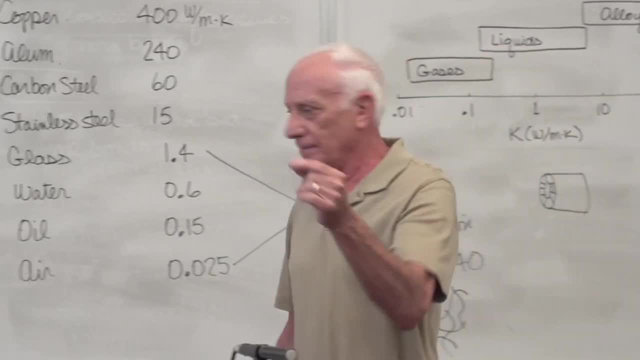 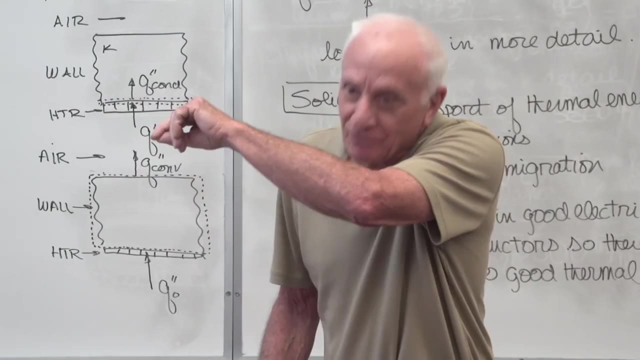 Now those down feathers are the ones that trap air. They look like that, They trap air. That's why you always see a duck doing this. They're fluffing those feathers up so they get air in them. They got to get air because they can get compressed by sitting. 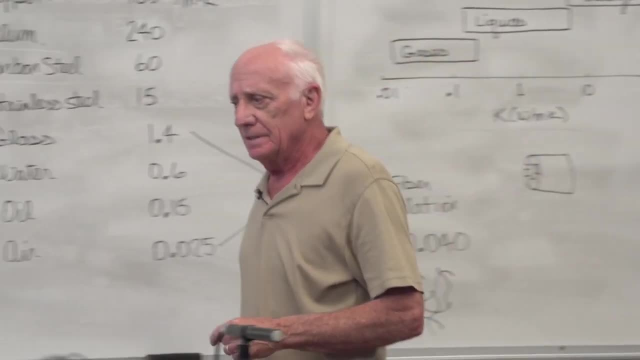 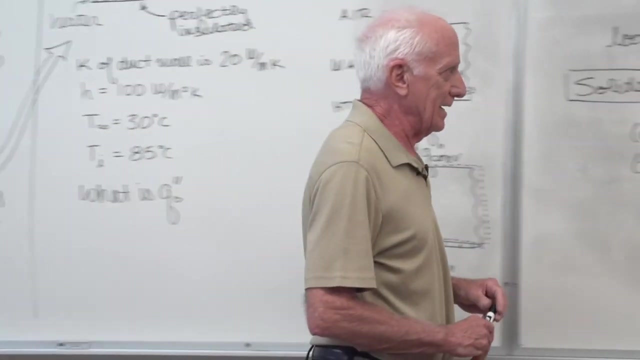 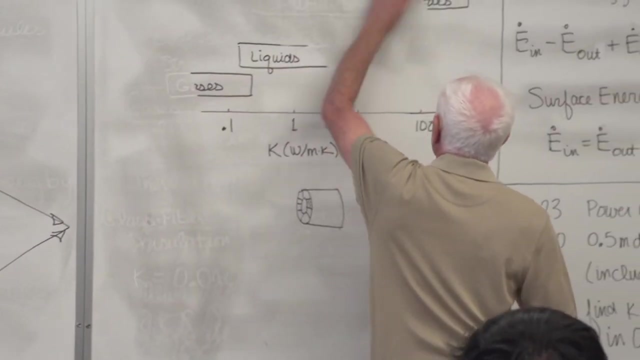 So they fluff them up, so they get air in those tiny feathers. Yeah, The lesson is: quiescent air, not moving, is a great great insulator. Now there's one more property which is interesting, and that property is called thermal diffusivity. 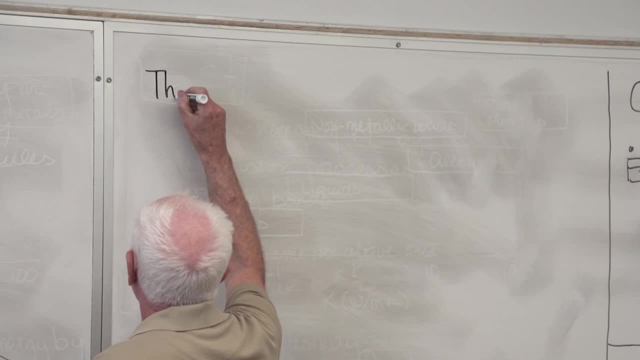 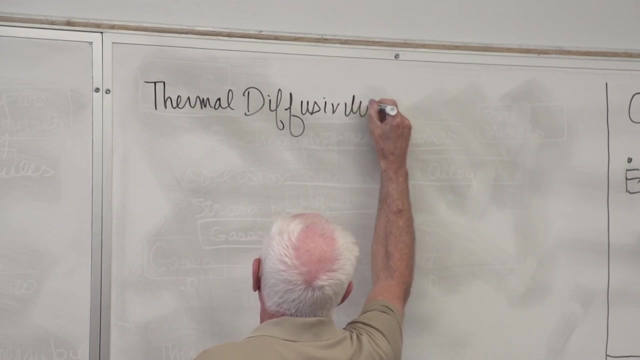 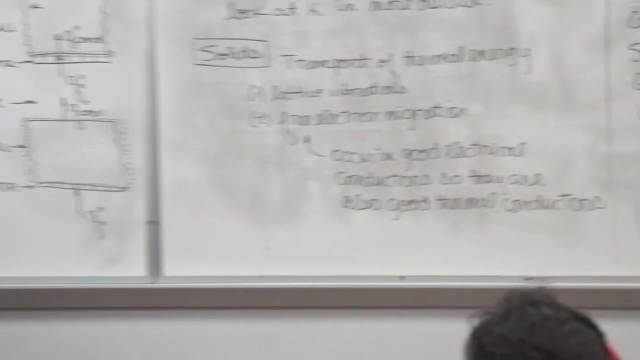 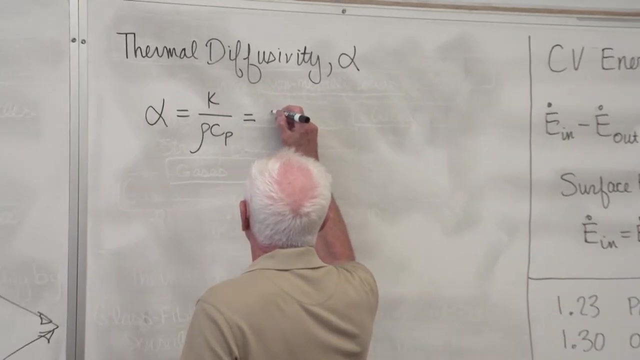 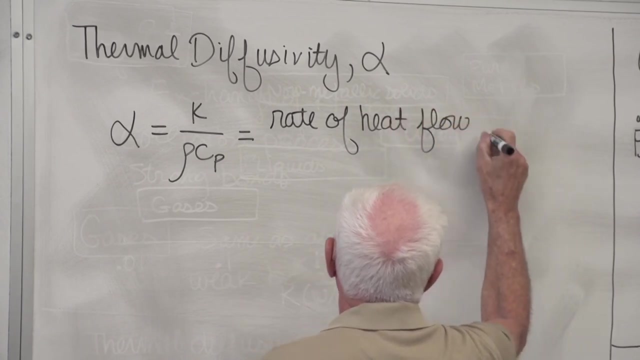 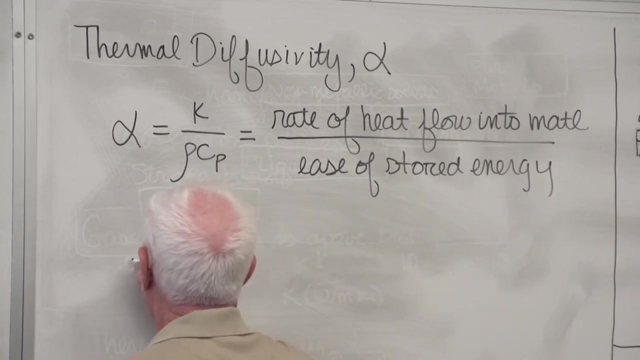 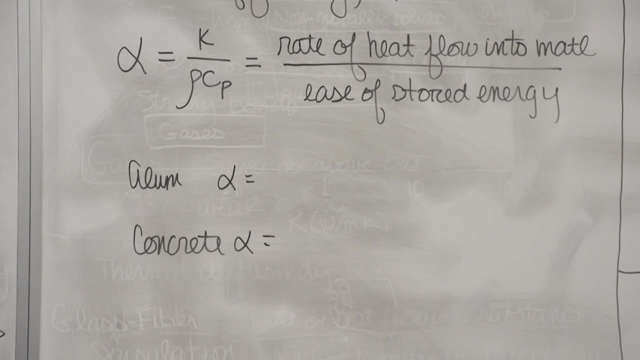 So let's just mention that real quick, called alpha. Alpha is K over Rho Cp. Now in words I'll put down what the words mean here: Alpha, Alpha, Alpha, Alpha. So to have a high value of alpha. 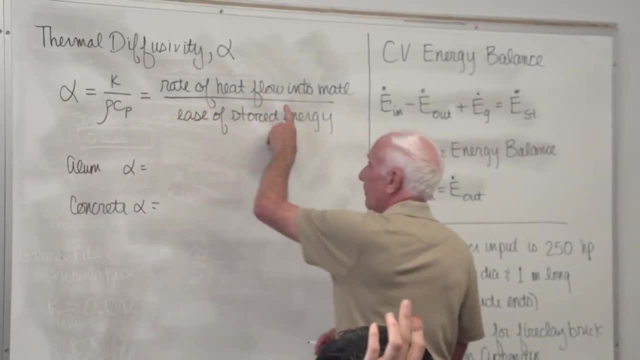 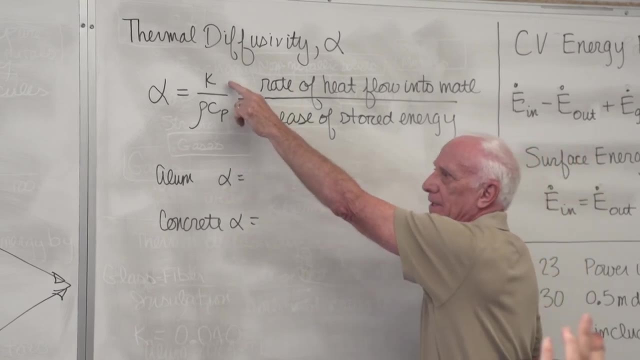 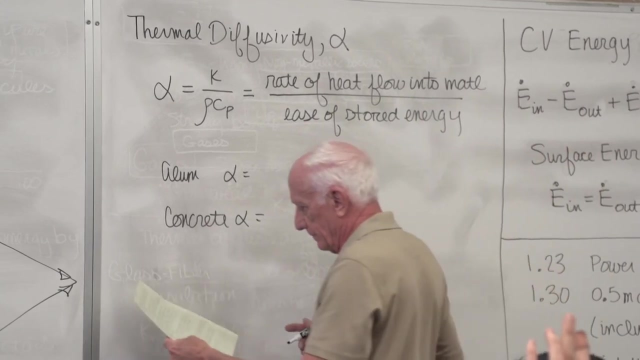 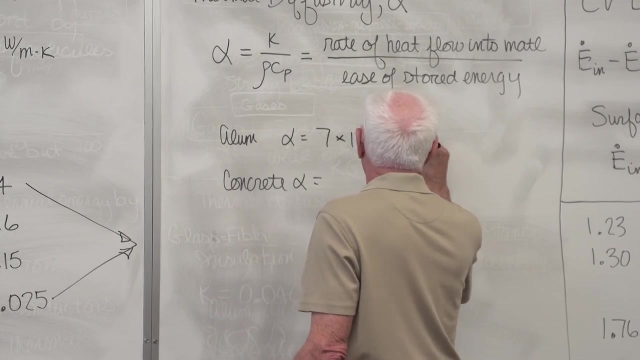 means that they conduct heat easily by conduction k, but they don't store much. Small denominator, big numerator: They conduct heat easily but they don't store. So aluminum seven times 10 to the minus fifth meter square per second. 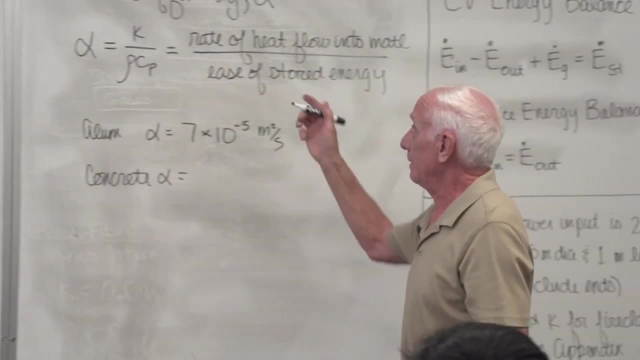 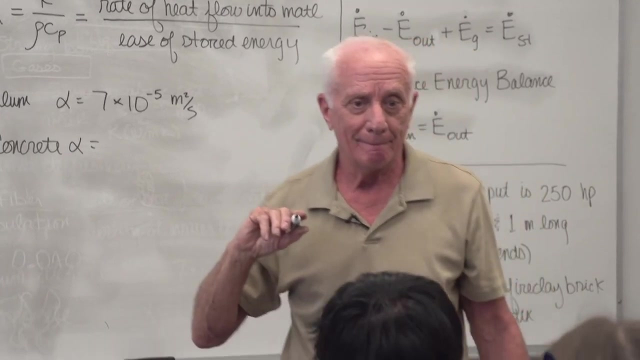 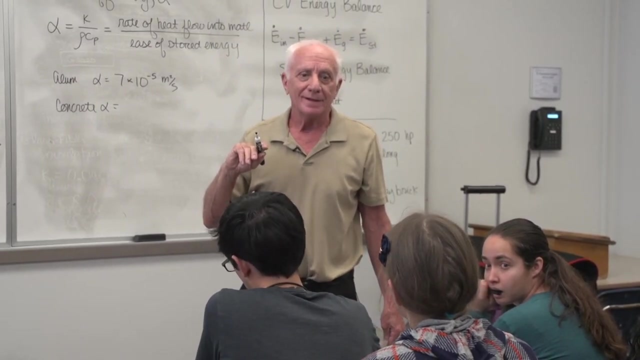 Concrete. now, concrete doesn't conduct heat very well, but it stores a lot of energy because it's massive. You said we don't want water within the stuff. What about? where does wool fit in? Because it's known for keeping you warm, even when wet. 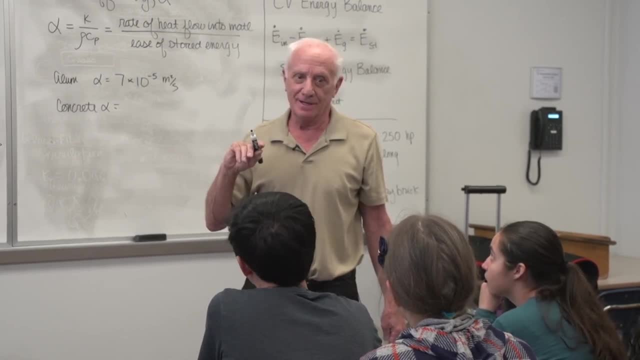 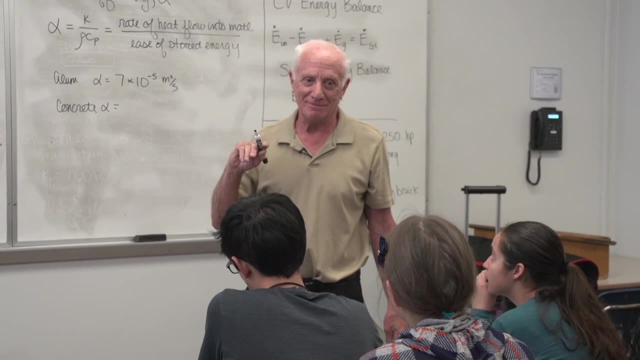 It's wools, sheep. It's great for trapping air, right, Look at it. Look at a piece of wool, It's great. So, yeah, it's also good. Not as good as down feathers, though. Yeah, Try and find k of wool. 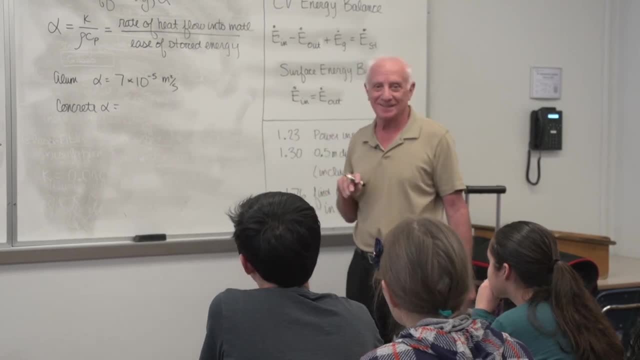 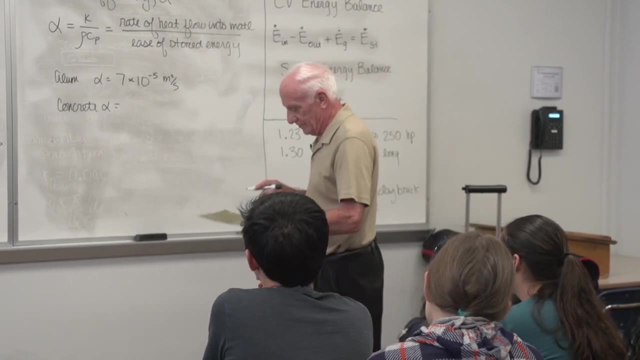 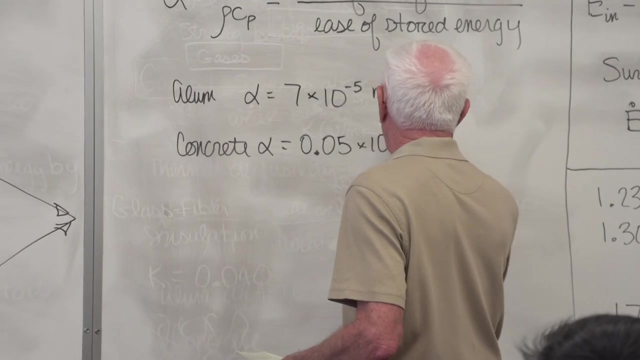 Let me know next time we come to class. Yeah, Google it and see what you get. It might be in the back of the book. even I think it is. I think it is in the appendix Concrete 0.05, 10 to the minus fifth. 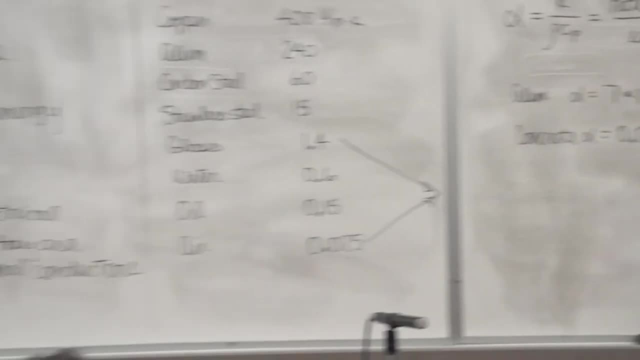 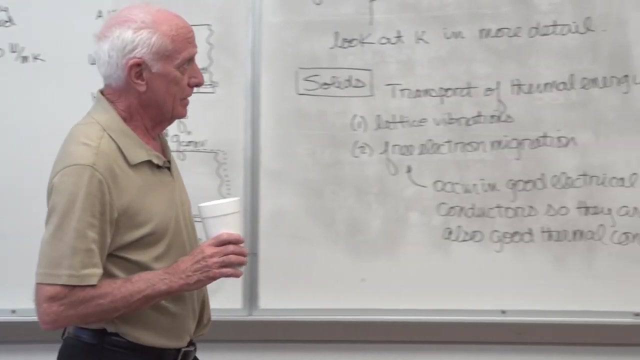 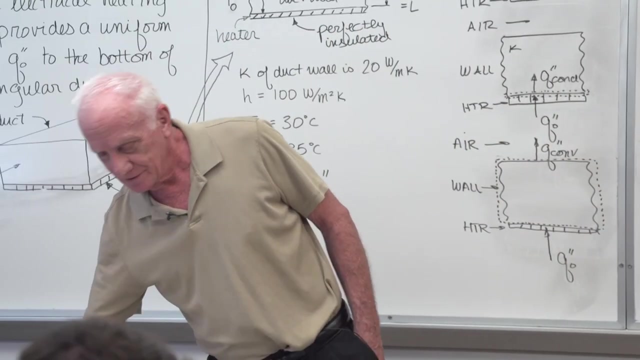 What does that mean? First of all, it's an important property in heat transfer. It is a property because it's a combination of three properties: k, rho, c, p. So here's a game to play with your friends. 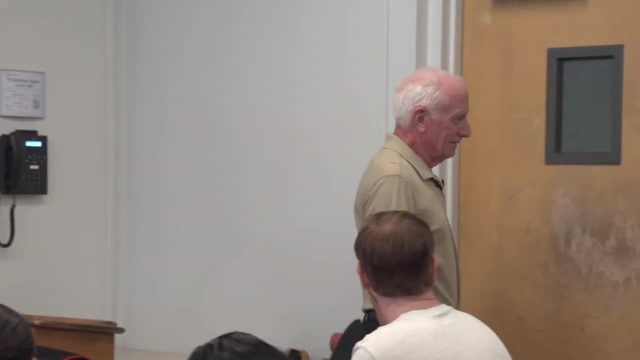 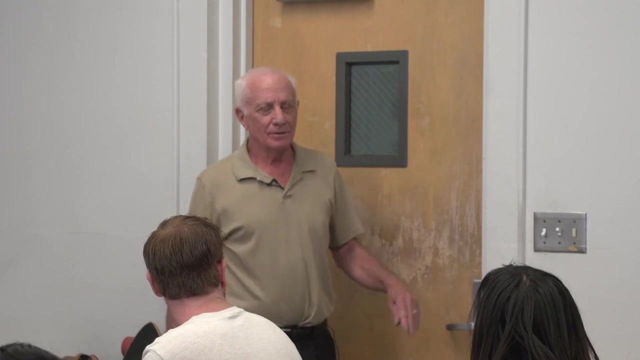 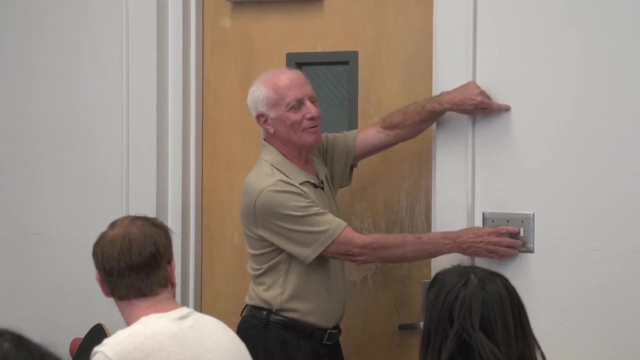 non-engineering people maybe Say: you know what? Here's an aluminum plate here, switch plate, Here's a concrete wall. You tell them: close your eyes, put one finger on the aluminum P, One finger on the concrete. 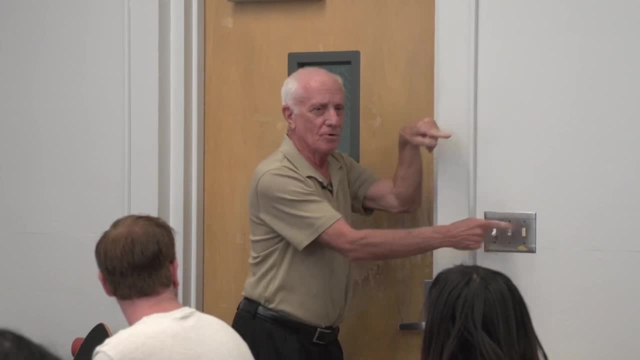 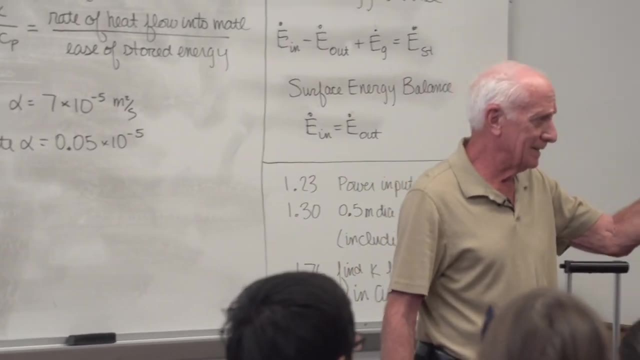 Which one's colder? The guy says yeah, the aluminum's colder. I say okay, Do you really believe that in this room Is there a little mini refrigerator behind that thing keeping that plate cold? No, Is there electrical heating wires in the wall. 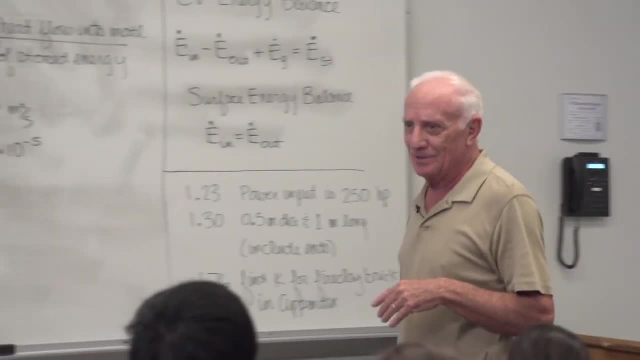 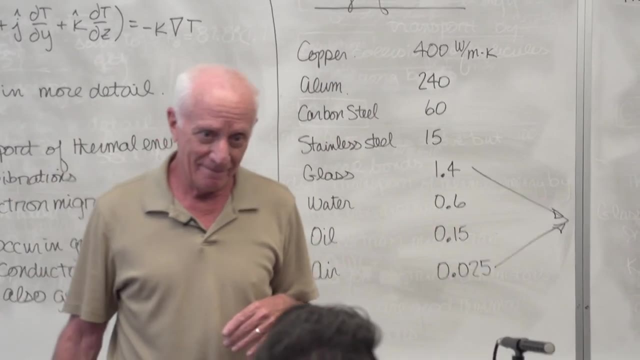 keeping the wall hot. No Conclusion: I guarantee you they're the same temperature, but something's fooling you. I heard there's a story similar to that with diamond miners, because I guess diamonds have the nickname of something like ice or something. 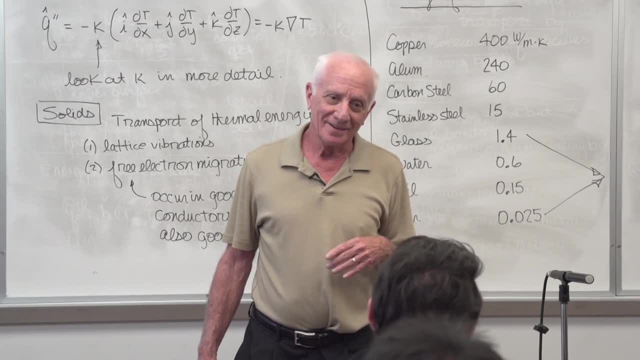 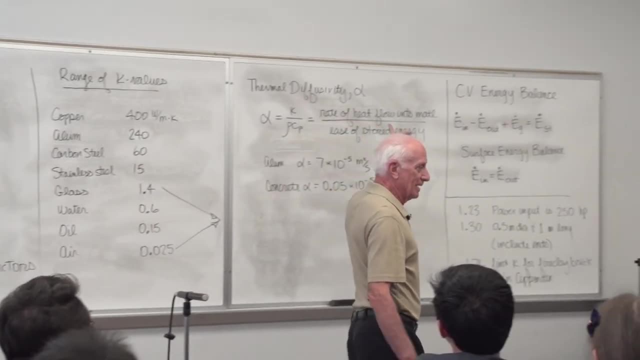 Because if you lick a diamond, even though it's the same temperature as this running area, because it's so conductive, it pulls the heat out of you, Probably explained by this. Because it's explained by this, My fingertips are the same temperature.